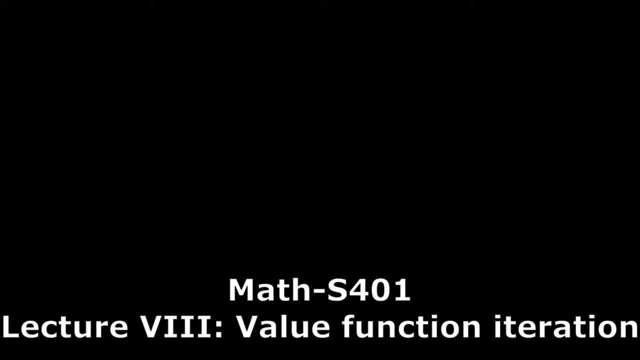 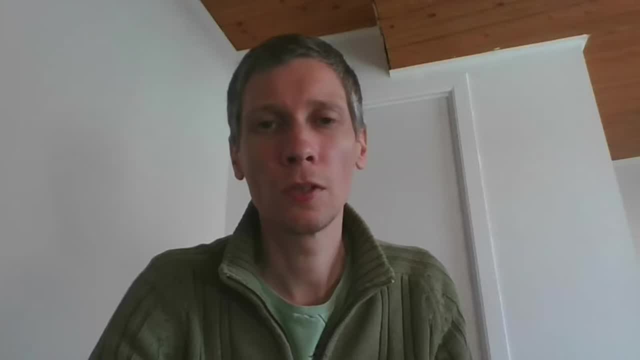 Hi, welcome to this new lecture of Math S4.1, Dynamic Optimization. Today we're going to look at value function iteration. So in the previous lectures we have seen all the mathematical concepts and tools surrounding the Bellman equation and the Bellman fixed point and so on. 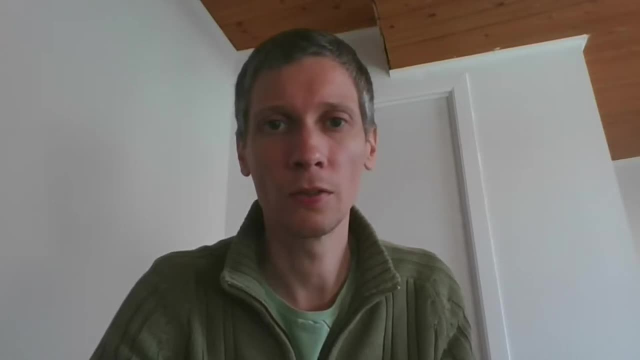 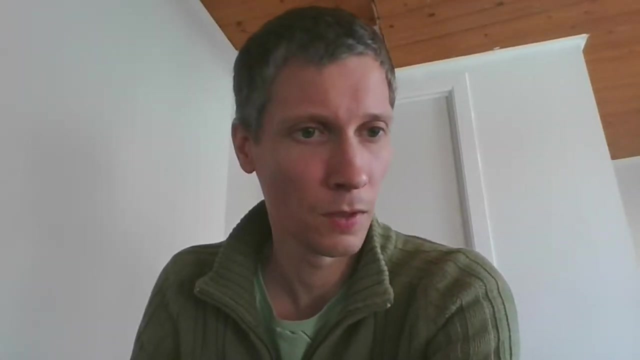 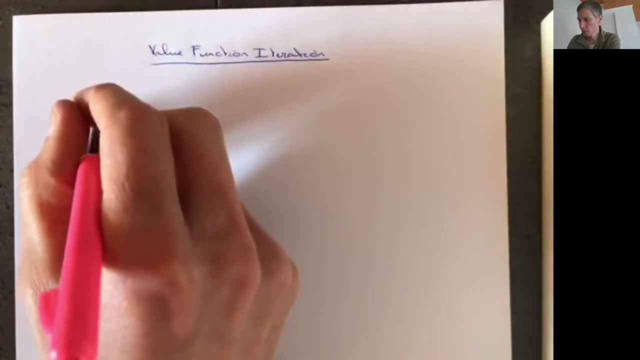 Today we're going to see how to use a computer in order to apply these concepts, And the first part we're going to work with is called value function iteration. So recall if we have a Bellman operator, it can be written like this: 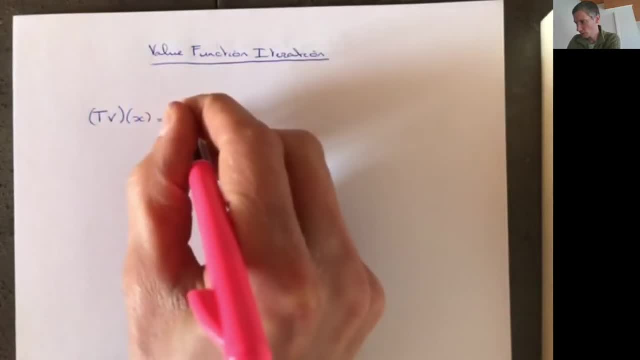 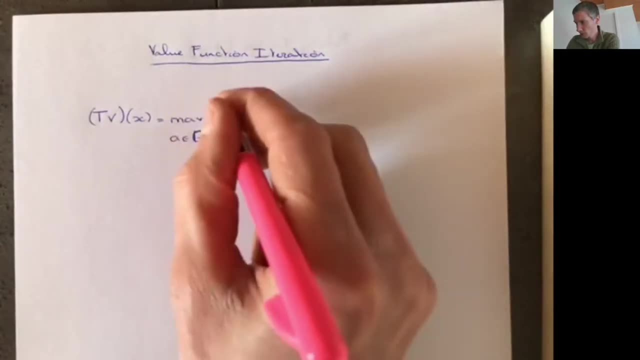 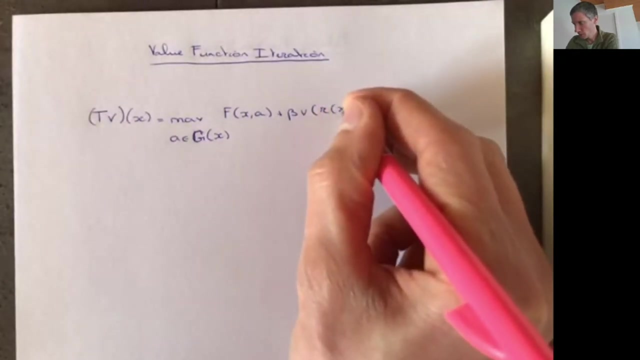 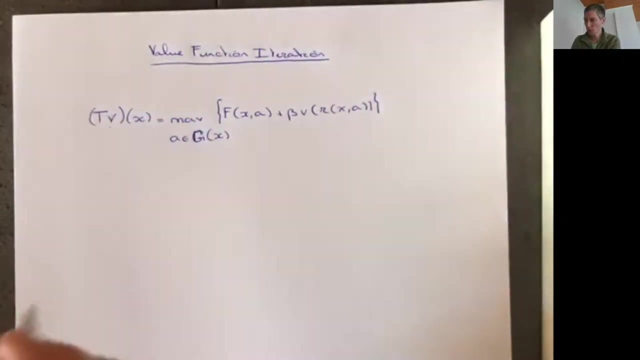 Tv of the state, x is a maximum over actions in some correspondence g of x, over the instantaneous utility function, fx xa plus beta v and then r xa. Okay, so this is the Bellman operator And if you want to solve the infinite horizon dynamic optimization problem, 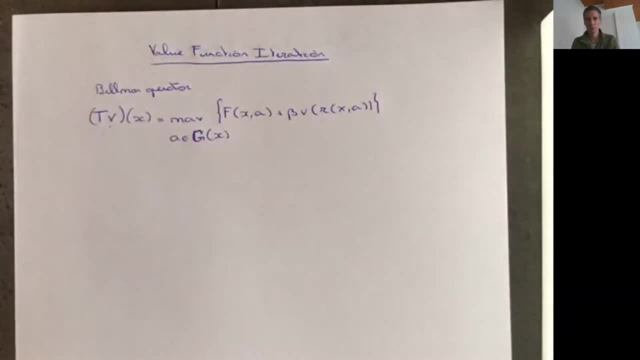 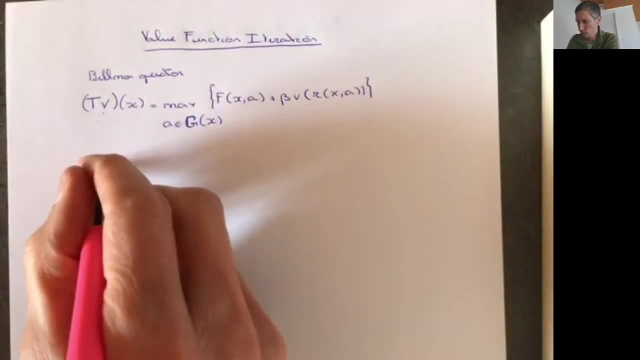 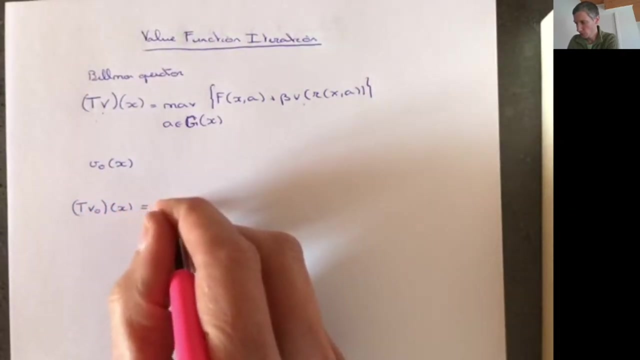 then basically you have to find the fixed point of this operator. Okay, but because this is a contraction mapping, what we can do is we can start with some function: v0 of x, okay, then plug this in here, And then we have, we apply the Bellman operator t, v0, okay, so which is going to be equal to: 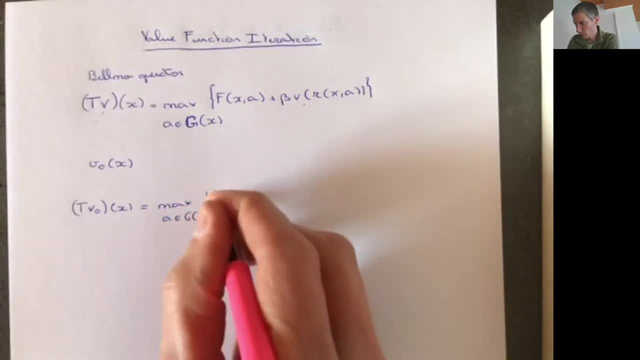 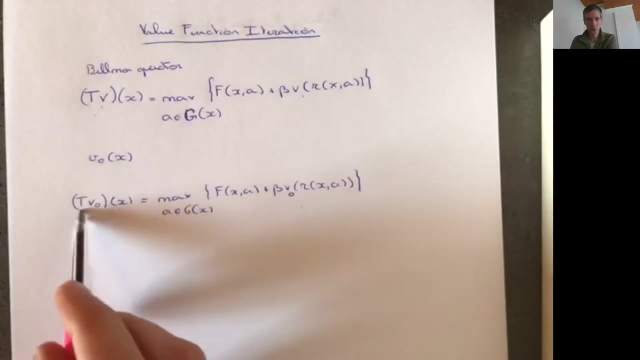 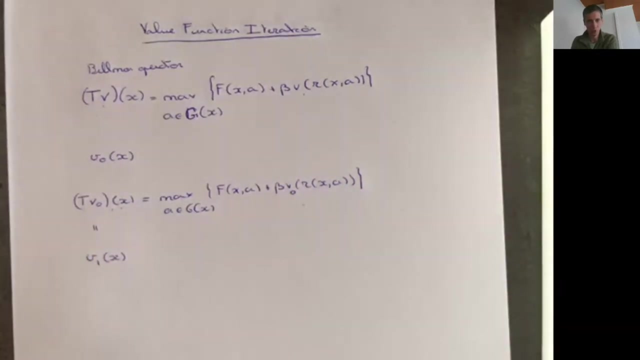 the maximum of a in g, of x, of f, xa, plus b, v, r xa, of v0, okay. So for every x, we solve this problem- we get a new function which is going to be t of v0. And we can call this the function v1, okay, which will be a function of x. 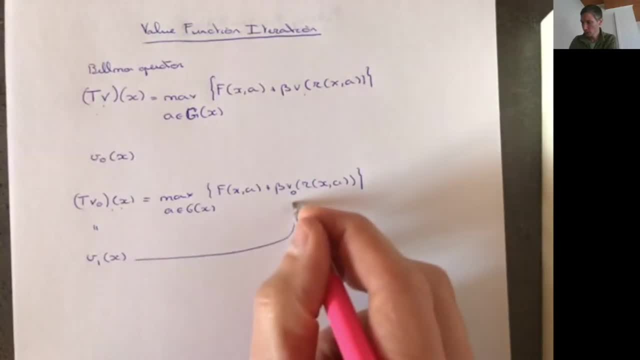 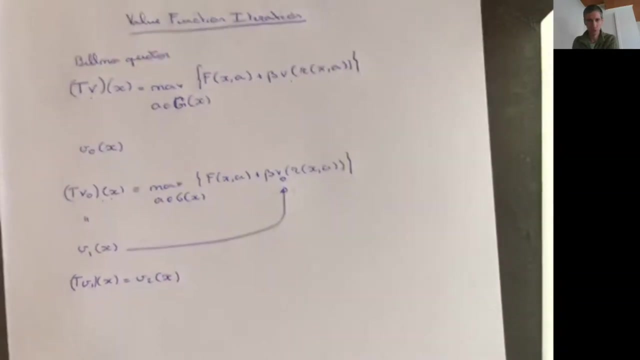 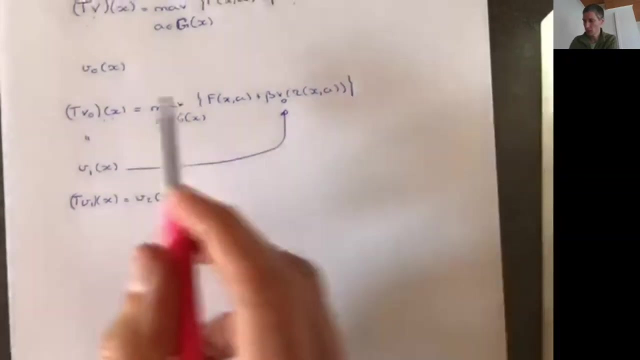 Then what we can do is we can plug this back in to our Bellman operator. Then we get a function t, v1 of x and we can call this v2 of x. okay, So if you do this over and over again, plugging in our current function into the maximization problem, 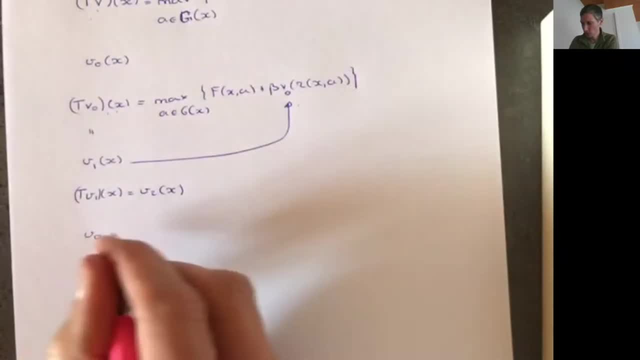 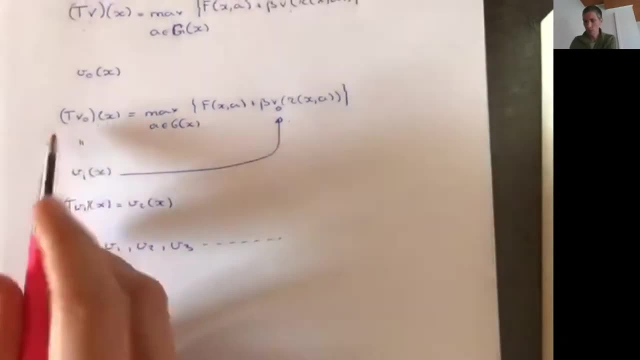 we get a new function, and so on, and so on. So we get a sequence of functions: v0, v1,, v2, v3 and so on. okay, And you know, because this is a contraction mapping, this will converge to our fixed point v star. 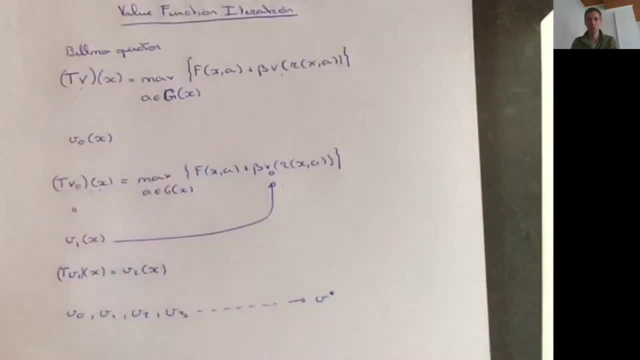 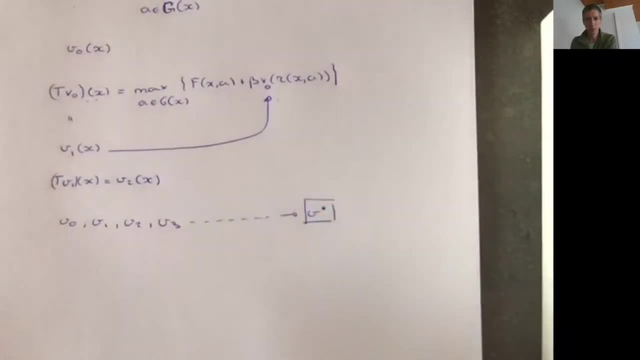 which is the function that we're interested in, because it will solve our infinite horizon dynamic optimization problem. Okay, So the problem is now: how can we compute this v star? Well, in principle, it's very easy. We start with any function that we can think of. 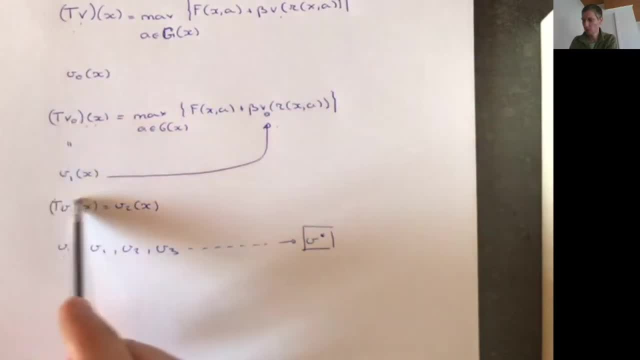 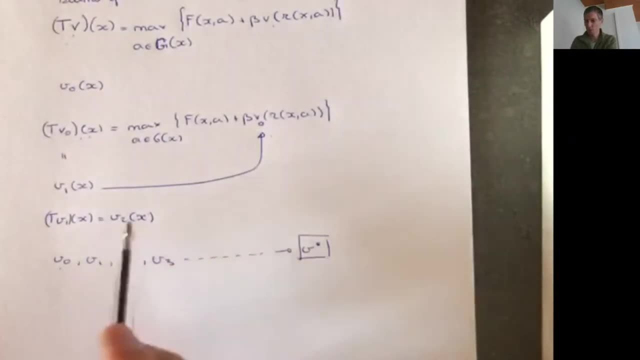 We plug it in here We compute a new function. We take this new function, plug it in here, We compute a new function, and so on, and so on. okay, So this procedure of starting with some function, generating new functions by using the Bellman operator. 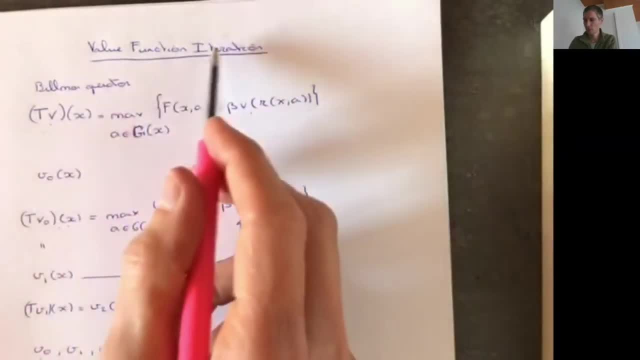 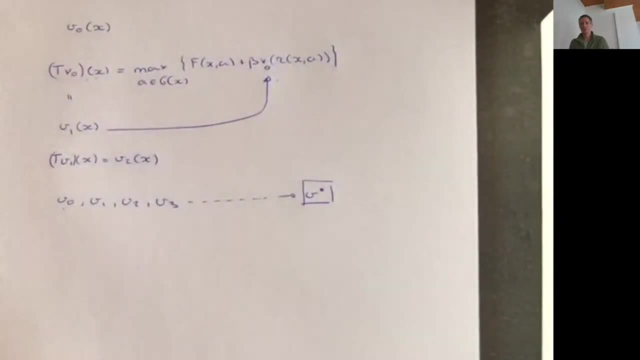 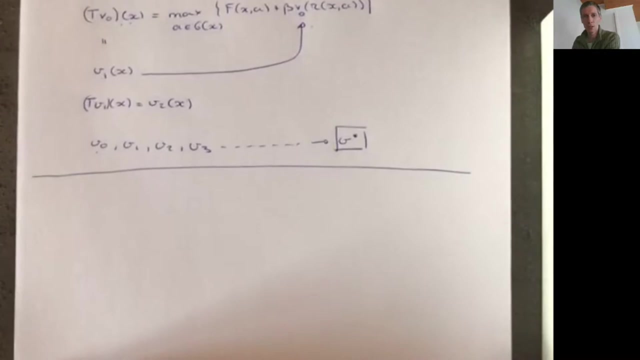 this is called value function iteration- right, because you iterate the value function over and over again. So mathematically, this is all very nice and easy. Of course, you would like to implement this on a computer. okay, And if you want to implement this on a computer, there are a few things that you have to take into account. 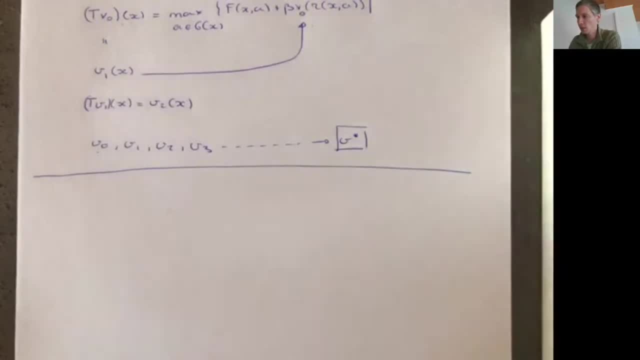 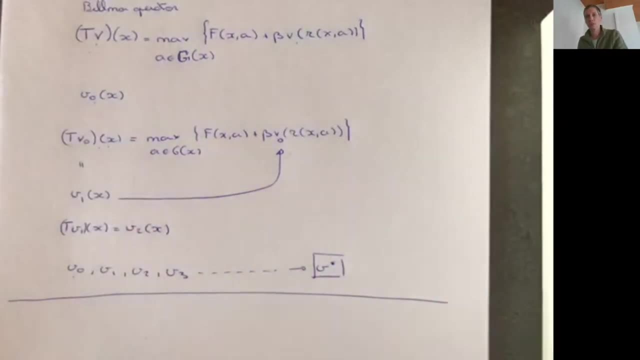 And the most important thing is that computers don't take as inputs continuous functions. right, because computers are finite. You can only store finitely many data in a computer. You somehow need to transform, You somehow need to transform this into a finite setting. okay, 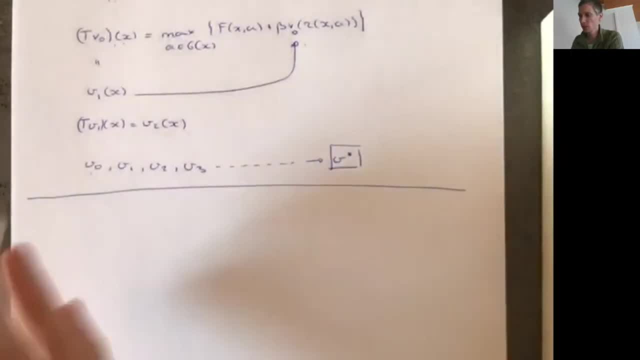 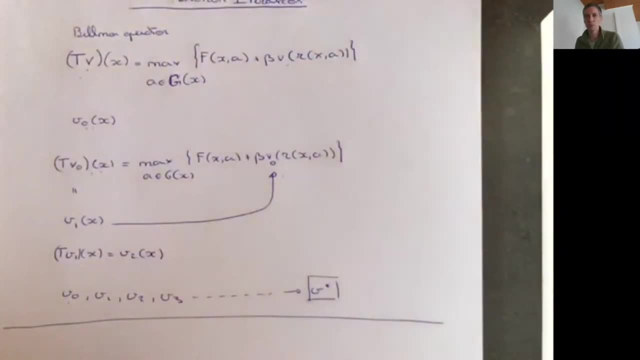 So the first thing that you probably need to do is to transform our infinite horizon dynamic optimization problem, which we treated as being continuous and, for example, the set X of all states was infinitely big. right could be a subset of Rk. 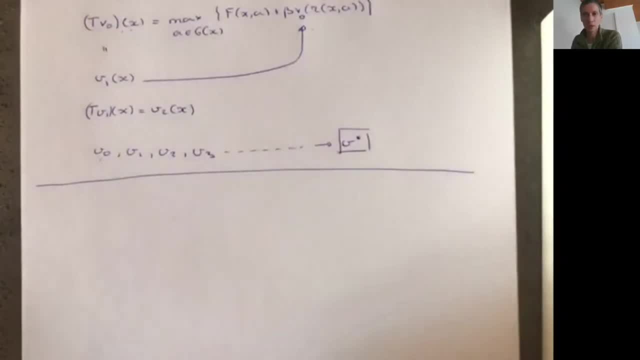 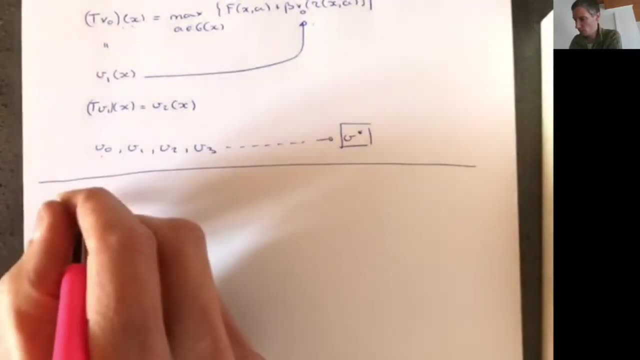 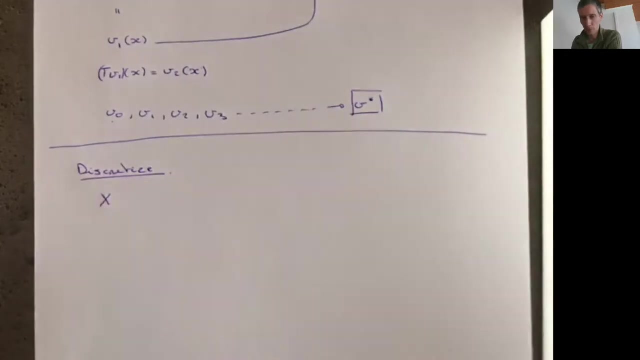 So now we have to make it discrete, which means that we have to somehow discretize all these sets, okay. So this will be the first step. The second step that you need to do: you need to discretize everything, okay. So, in principle, in particular, what we need to do is we need to substitute our infinite set X by finite sets of possible Xs, okay, 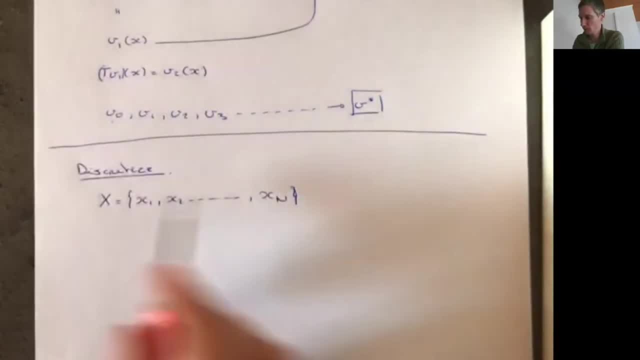 And let me call big N, let me call this the size of the width of the set X. okay, So here N, And in some way we make a grid, finite grid of possible states. okay, You have to do the same with the set A, okay. 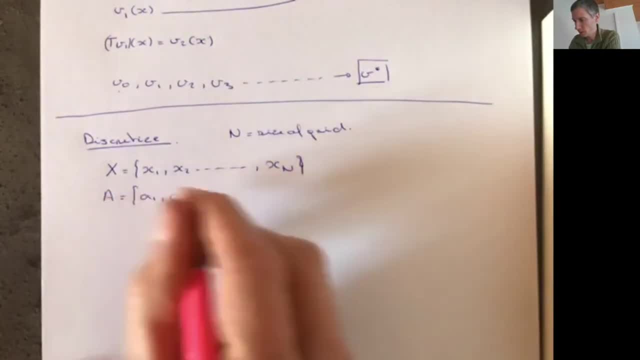 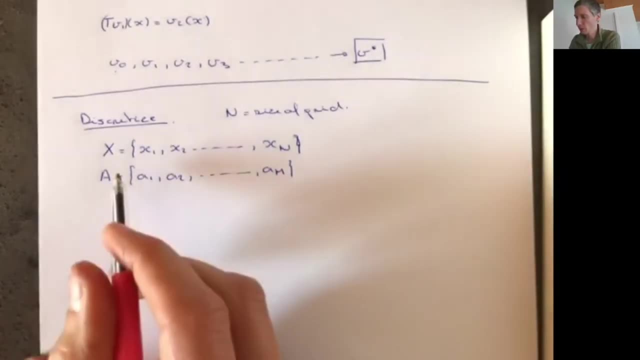 You have to say there's a state A1, there's an action A1, an action A2, and so on. okay, So maybe there's M actions that we can take, Of course, if you have a finite grid of states, a finite grid of actions. 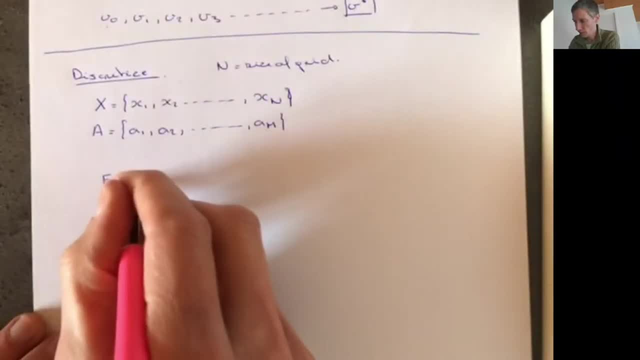 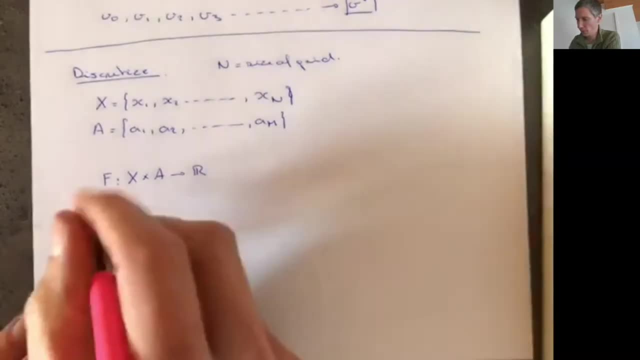 then all these functions: F now takes a state here and an action here and produces a number R. Our correspondence G takes a state here and produces a subset of this set A of actions. okay, So basically you have to transform everything to the finite setting. 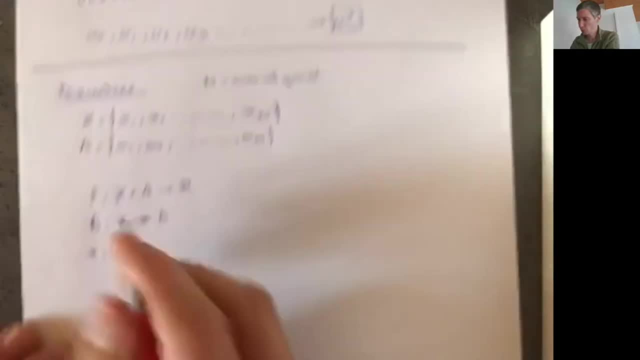 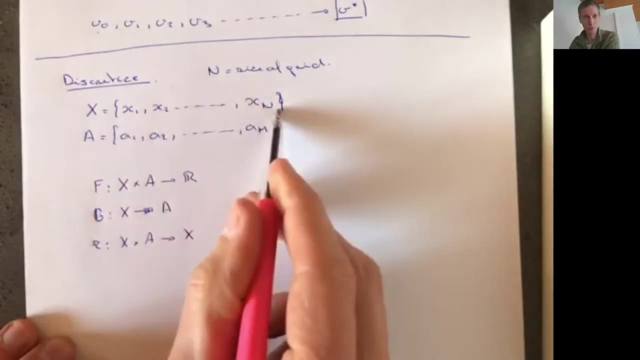 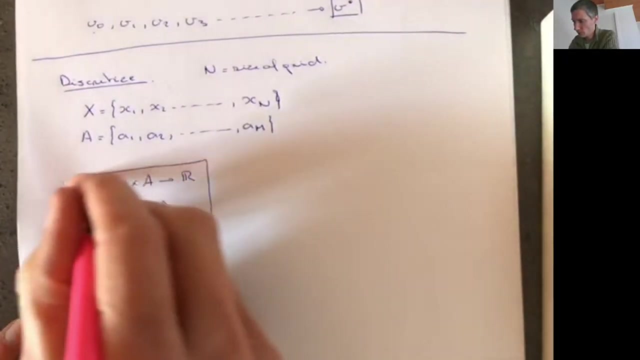 And then R. We take a state in here, we take an action in here and we produce a state in this finite set. okay, So we have to make everything adhere to this finite setting. okay, So you can say: okay, but we analyze this infinite setting. 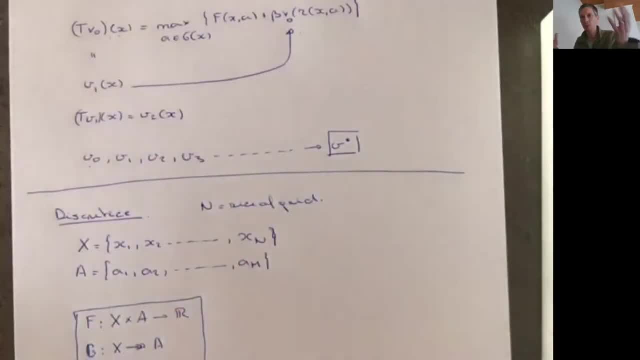 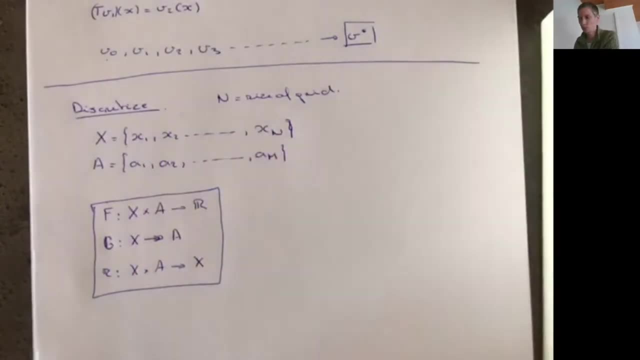 And we have shown that, indeed, okay, this converges. but we assumed everything to be continuous and infinitely big and so on. Well, you can show that if you make everything finite right, so if you only consider a finite number of states and a finite number of actions, 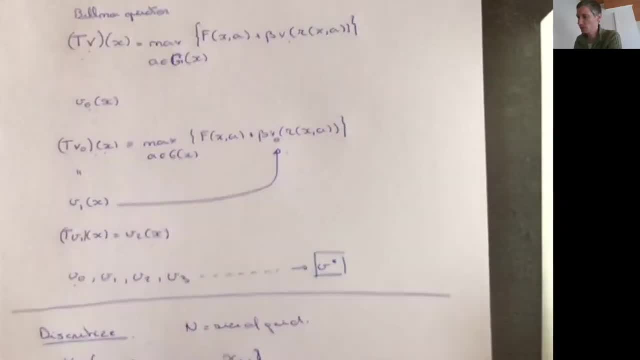 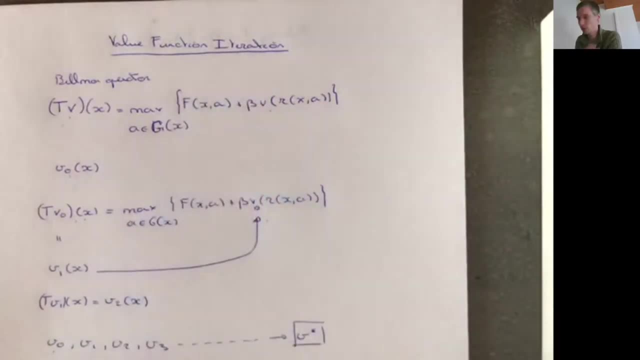 then all these results also hold, And in fact it's even easier, because if you only have a finitely many Xs and finitely many As, then this function is bounded anyway. okay, So we don't need all these boundedness conditions on the growth rate of some phi function, right? 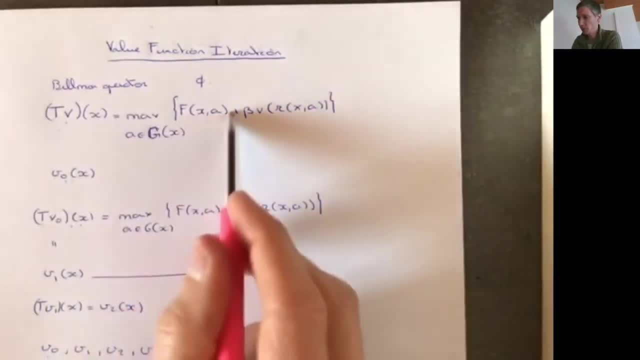 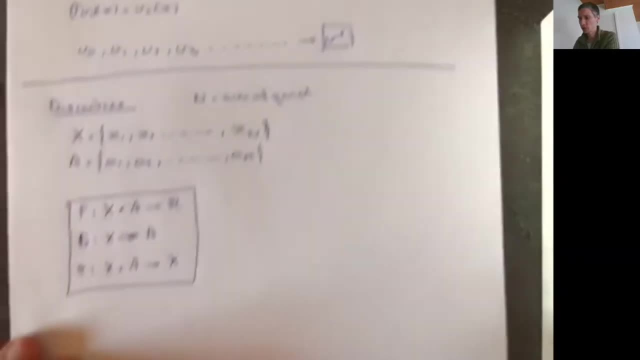 Remember, we take continuous and we don't need to bound this F from above by some function. function Okay, so we don't need all these additional conditions. Actually, if you only have finitely many states, life gets a lot easier from a mathematical point of view. 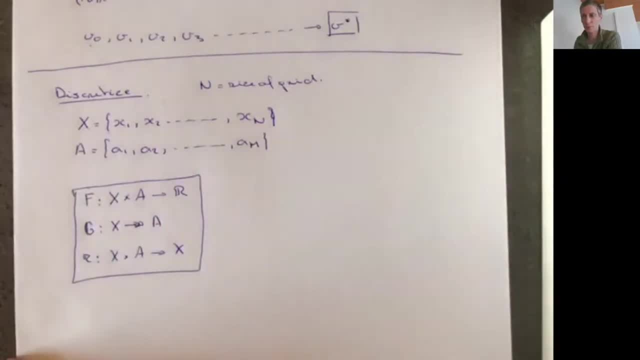 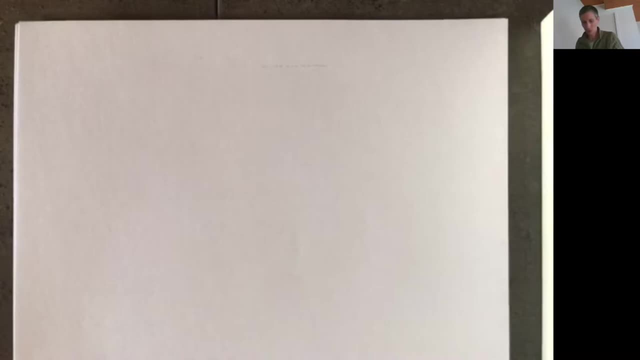 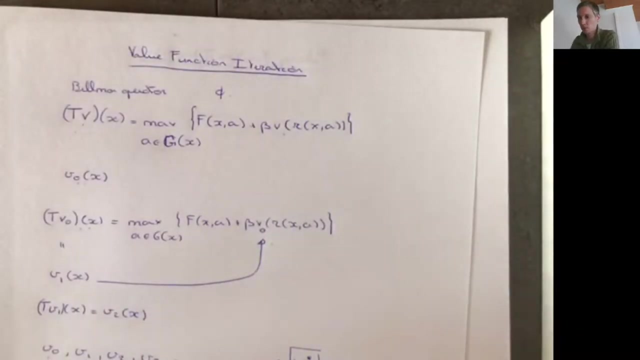 Okay, so this is the first thing that we need to do. We have to make it finite. Okay, then what we need to do is somehow we have to implement this maximization problem into a computer. Okay, so, in order to do this, 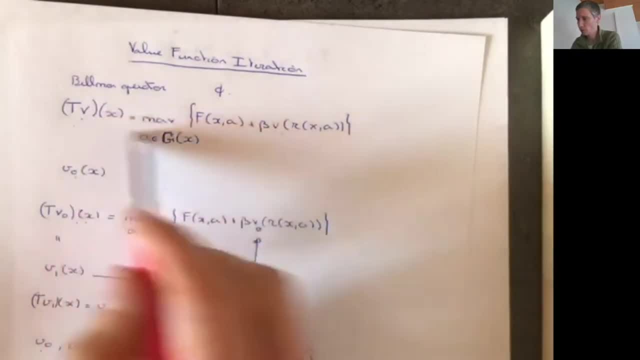 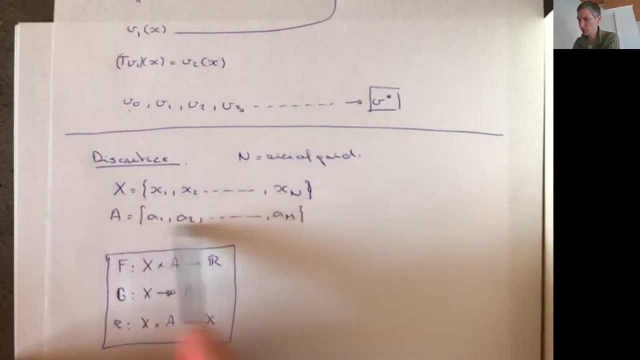 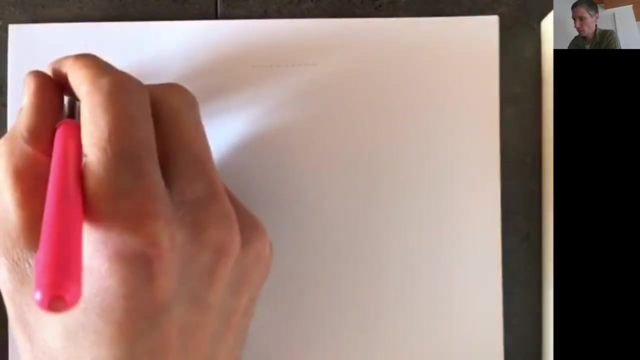 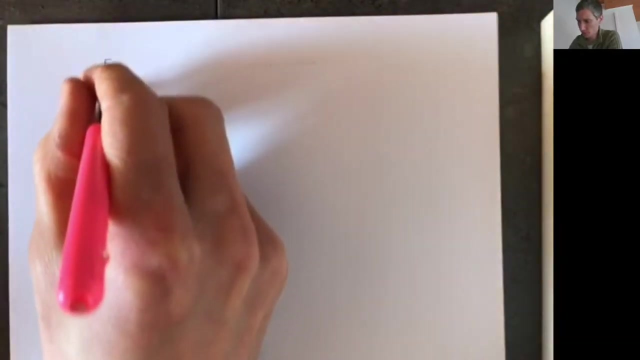 we have to store the set of states X into some data structure. We have to store this set of actions into some data structure. Okay, and maybe the easiest way to do this is the following: So X, we can put this into some vector, a big vector, right? 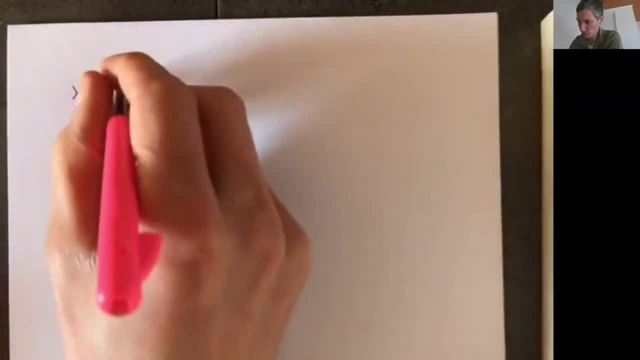 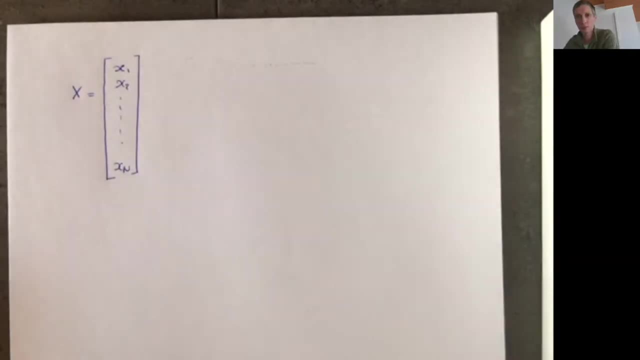 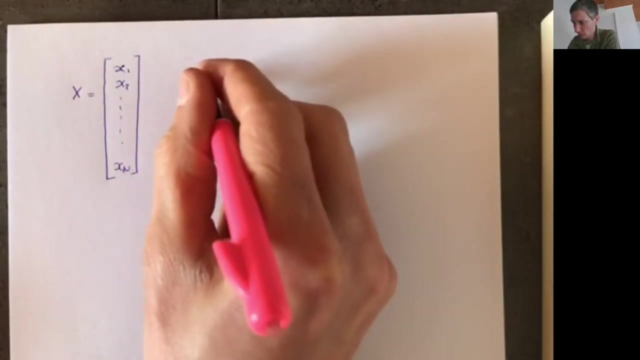 Let me write it like this, With values X1,, X2, and so on until Xn. Okay, so this is going to store this in the computer as an n-dimensional vector of size n. Okay, and the ith element, which I will write by: i. 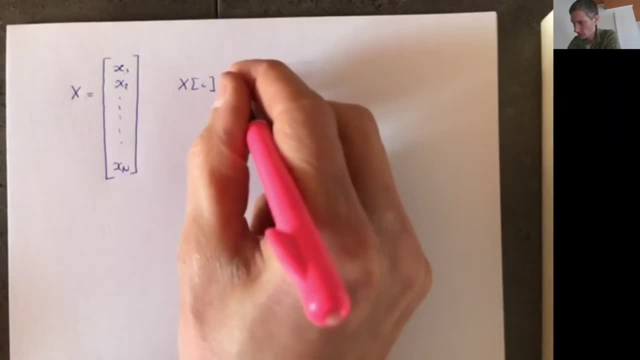 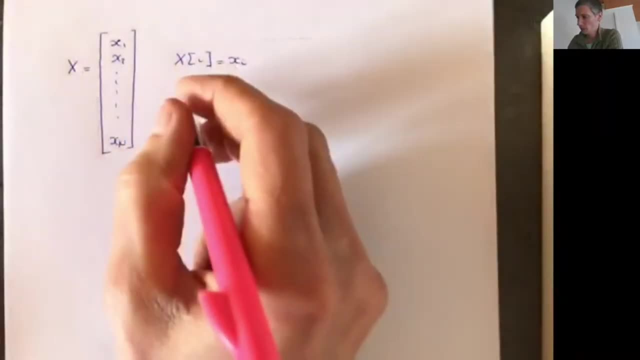 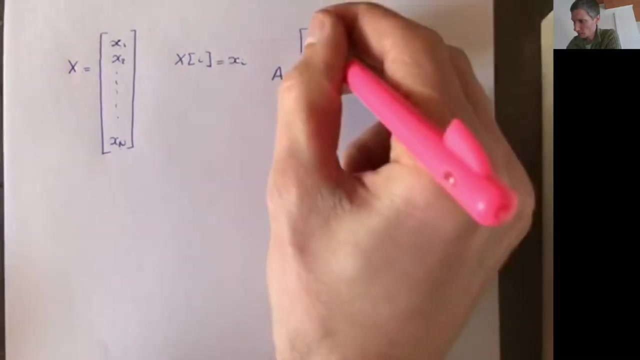 Okay, the ith element of this vector is going to give you the value, the ith value, of the state. Okay, so the value of state i. Okay, so that's the first thing, And then we can do the same thing with our a. 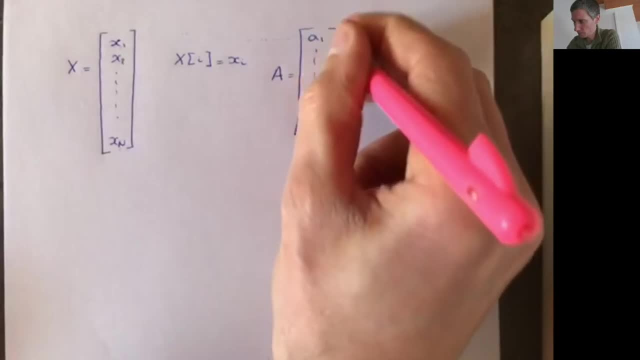 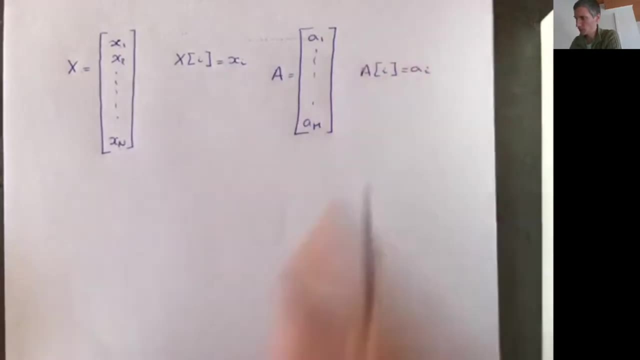 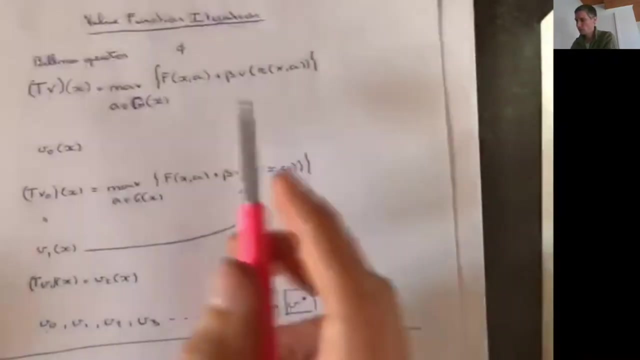 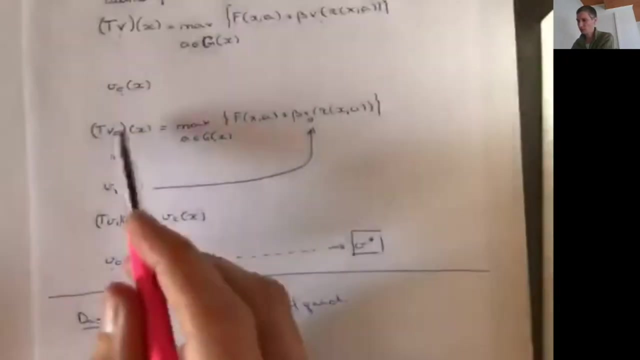 This is a1 until am. Okay. so here, ai, the ith element of this vector will give you the action ai. Okay, then you also need somehow to store the value function. Okay, Because at every time you're going to compute this one and you have to compute this on these finitely many states. 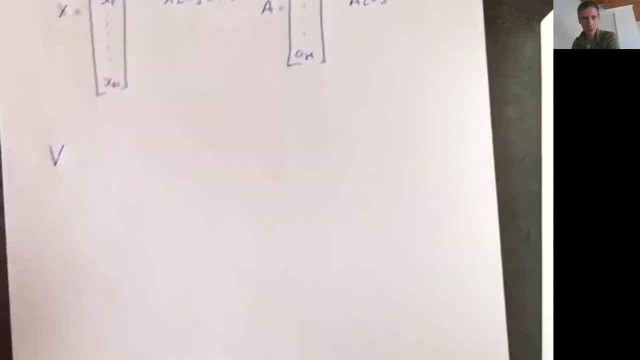 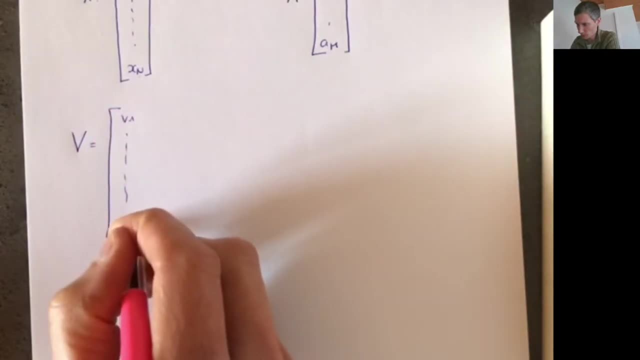 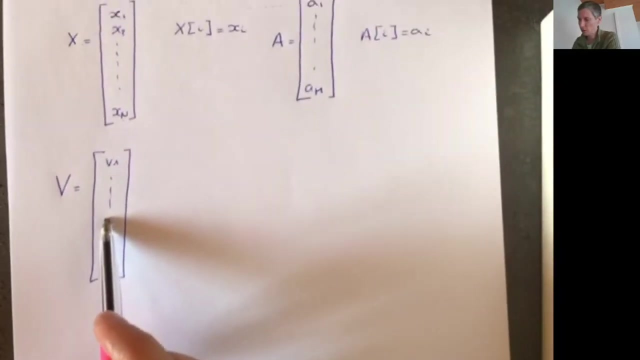 Okay, So a value function. you can write it as a big vector, v, which is going to have v1 until vn elements. So it's n-dimensional And the idea here is that v at position i gives you the value function of the state xi. 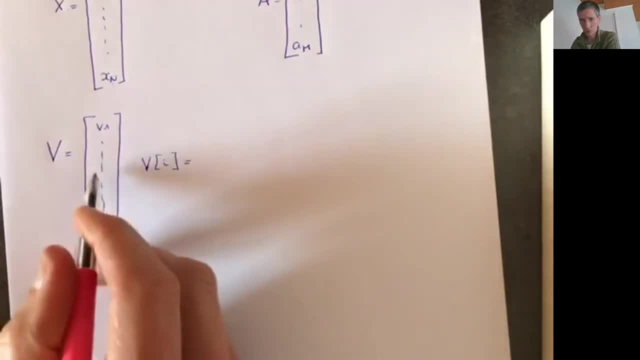 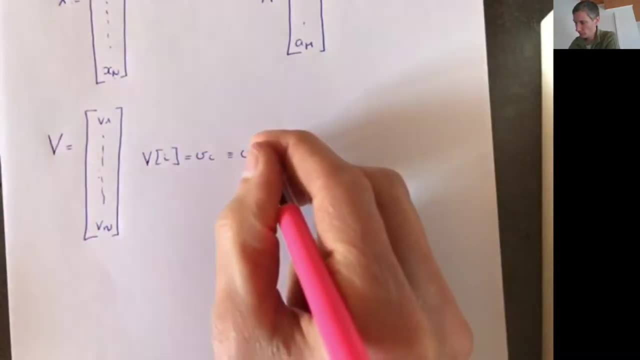 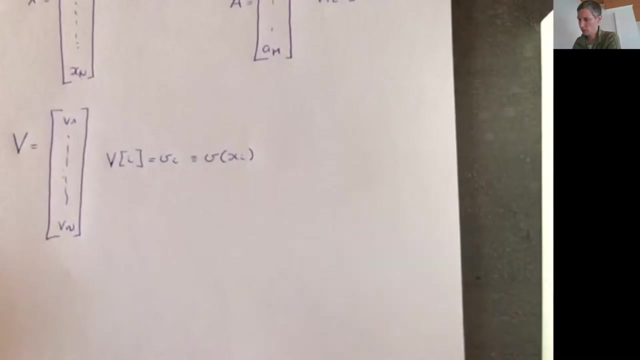 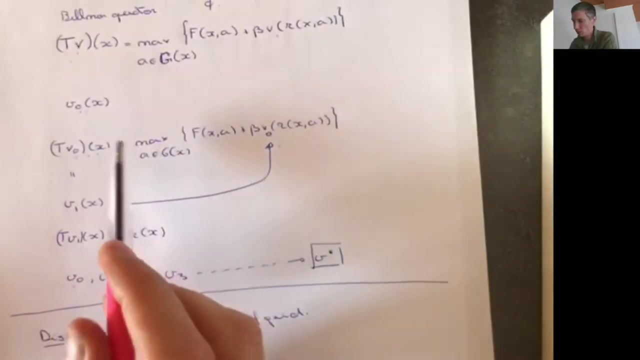 Okay, So vi, which is here the element vi, we're going to define it as being the value of a function, v at xi. Okay, And here xi is the ith element of x. Okay, So that's good. A final ingredient that we need is we have to solve this maximization problem. 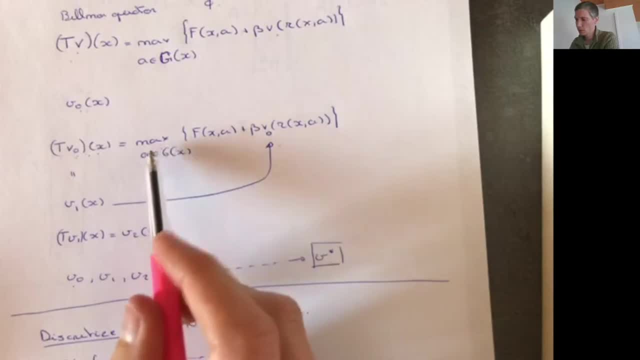 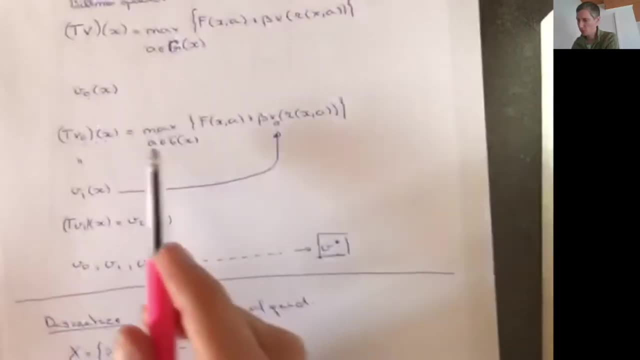 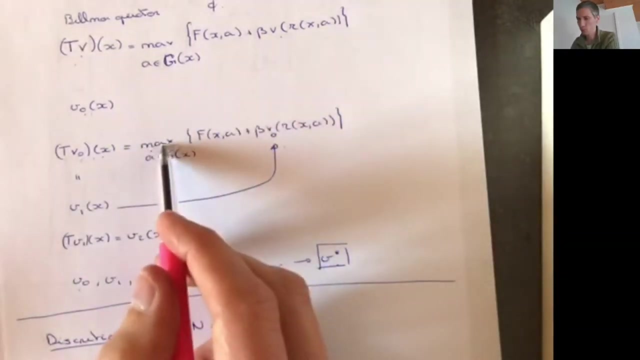 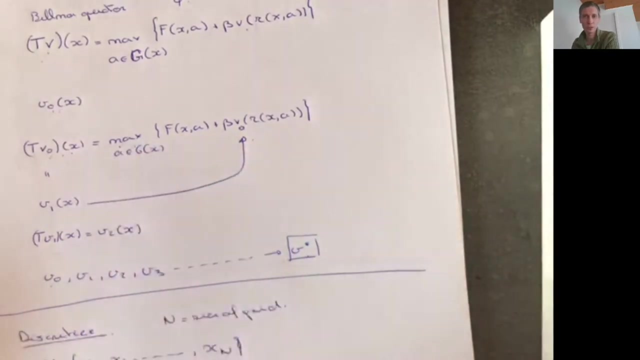 And at some point we also want to store the optimal solution of this maximization problem. Okay, So in principle, once we get to the fixed point, we want to know the policy function that corresponds to this fixed point. So we want to also not only know the value function, but we also want to know what action we should take at each state. 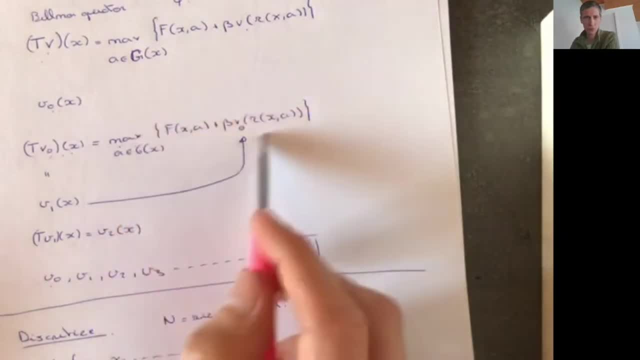 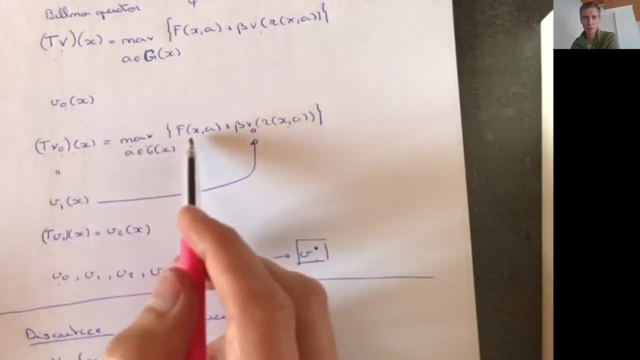 Okay, So we're going to store this solution of this optimization problem. Okay, So what do we have here? Here we have a state x- You want to solve it, And this gives us an action a, So we're going to. 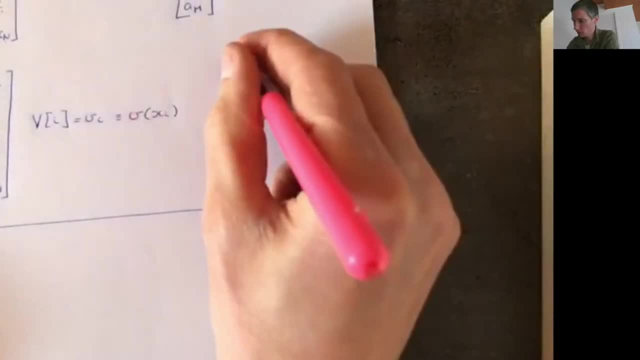 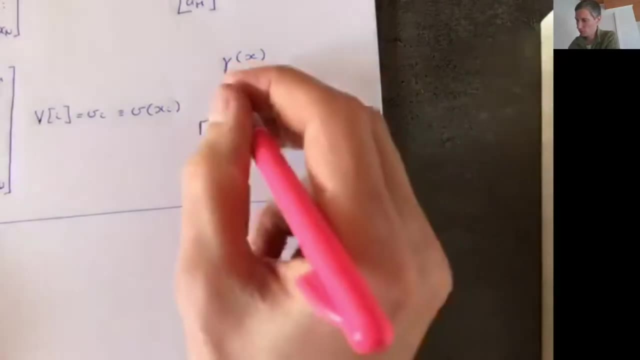 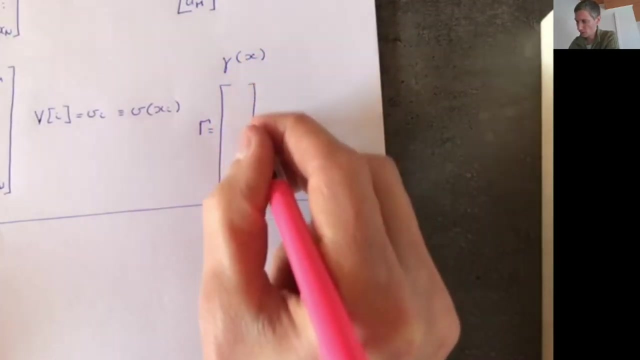 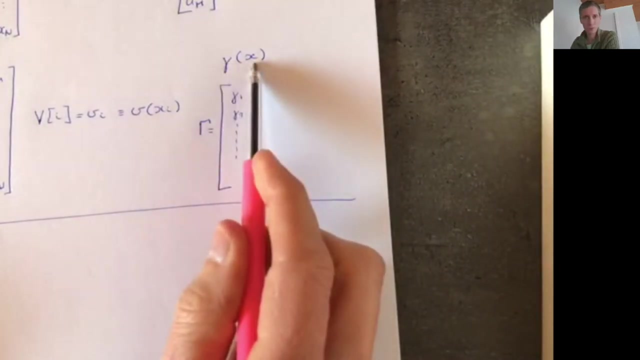 So previously we called this a correspondence gamma x, which tells you what action to take if a state is x. So we're going to store the solution of this problem into a vector gamma of numbers: Gamma 1,, gamma 2.. So we need to have a gamma for every x. 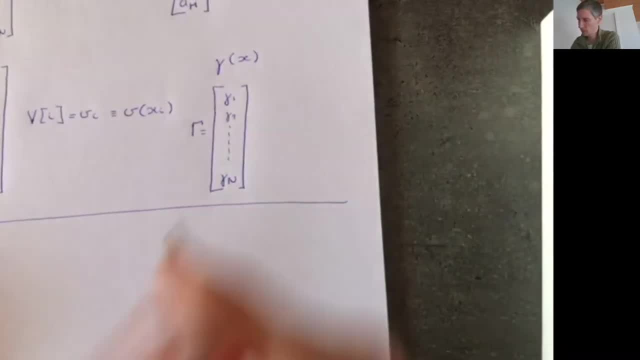 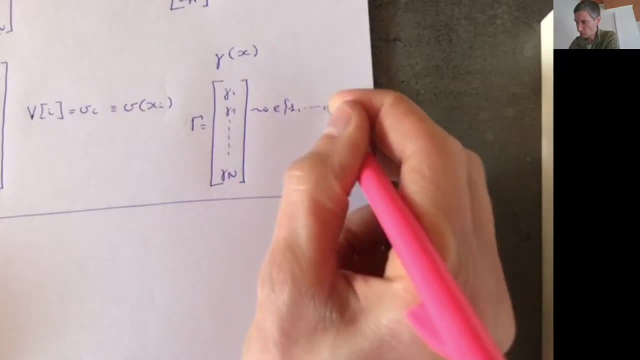 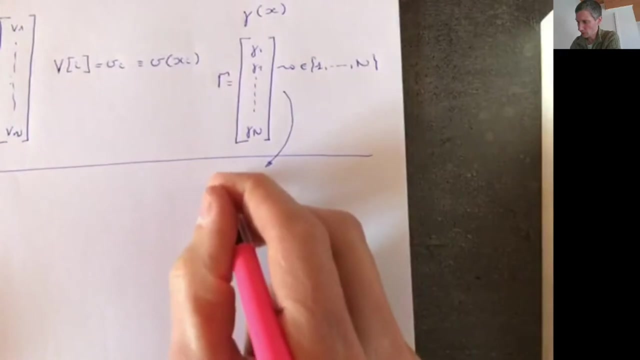 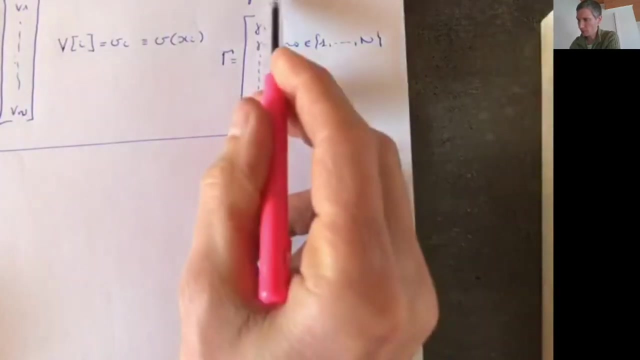 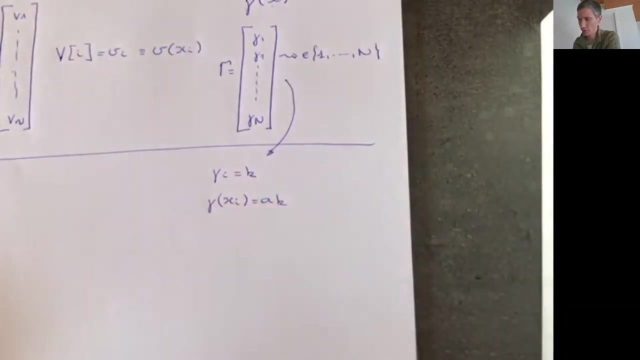 Right, So n of them, And the idea here is that these will be an element of 1 up to n. Okay, So what's the idea here? The idea is that if gamma, i is equal to, Let's say, k, Well then gamma, if the state is x, i will tell you to take action. a k, 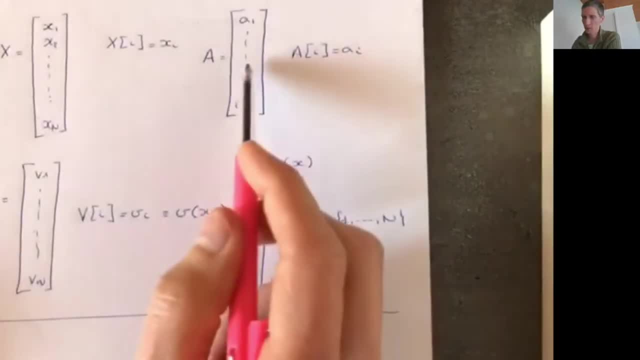 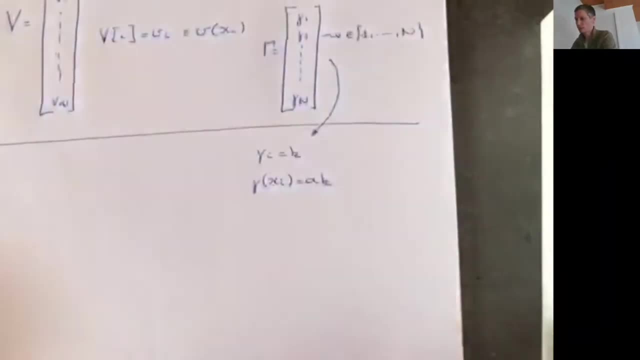 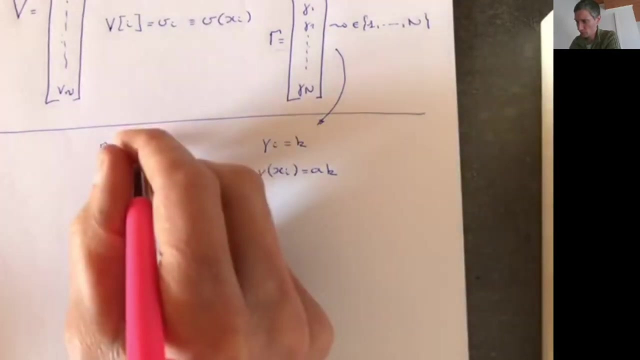 Okay, So it captures the index of the action that's optimal for the position of the state. Okay, So this is how we're going to do it. For example, if you have two states, 1 and 2. Then gamma is equal to, for example, 3, 7.. 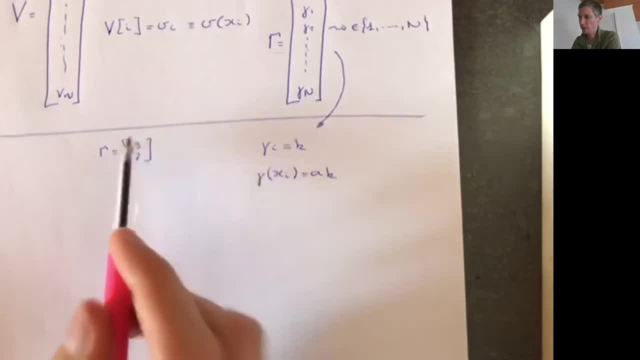 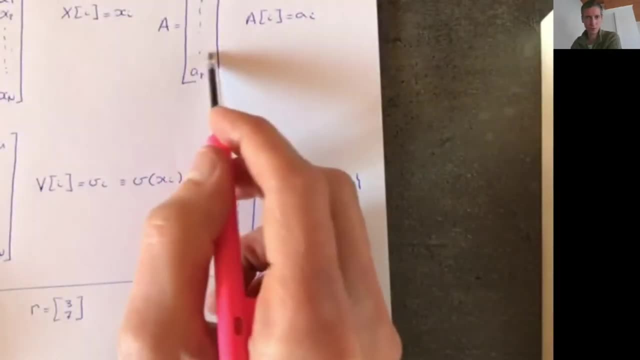 And says that at state 1, the best thing to do is to take action a 3, the third value of the action. At state 2, the best thing to do is to take the seventh element of the action. Okay, So this is basically how we're going to store everything. 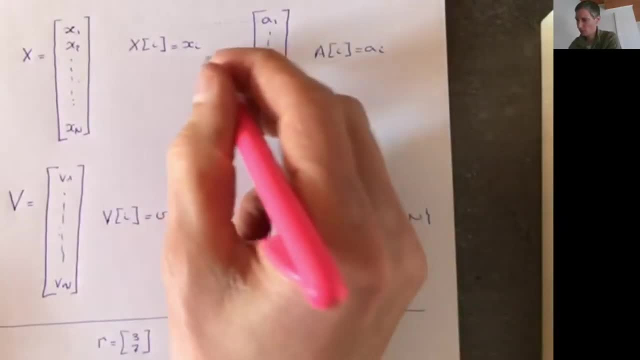 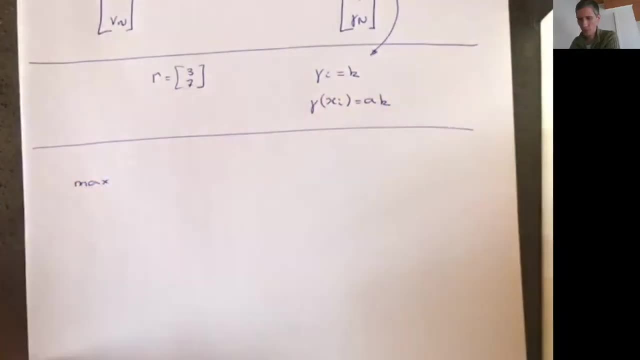 Okay, And to make my life easier, I'm going to equate the actions to the states And I'm going to look at the problem. Maybe I should have said this before, but I'm going to look at the problem that we have seen previously. 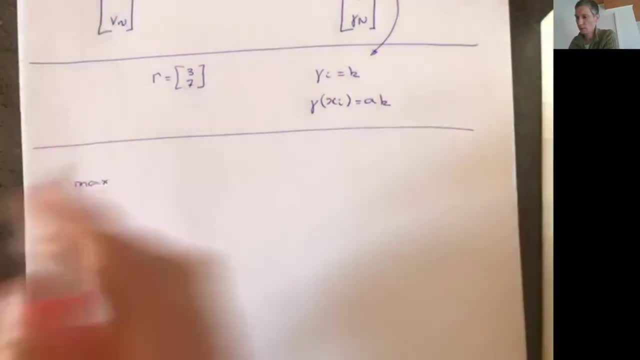 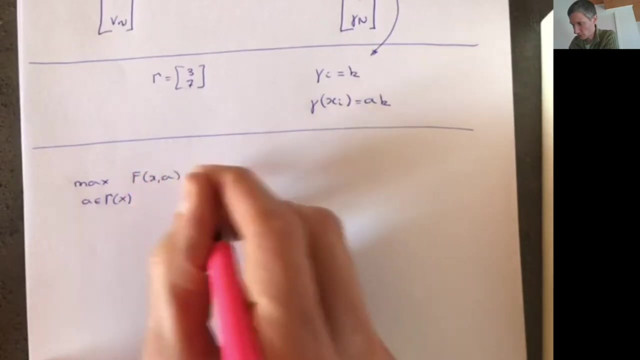 Basically, where the law of motion is the identity function And what you do is you pick the state tomorrow immediately. Okay, So we're going to take an action a in gamma of x to maximize f, x, a plus beta, b, a. Okay, 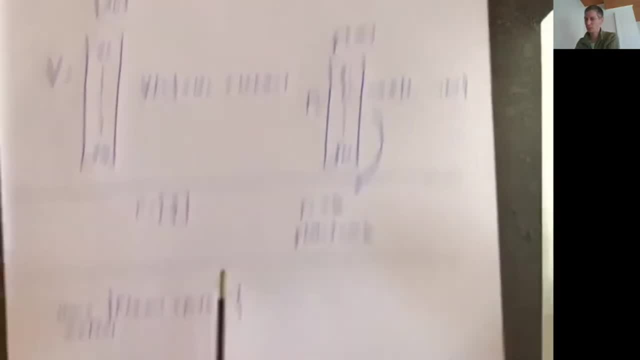 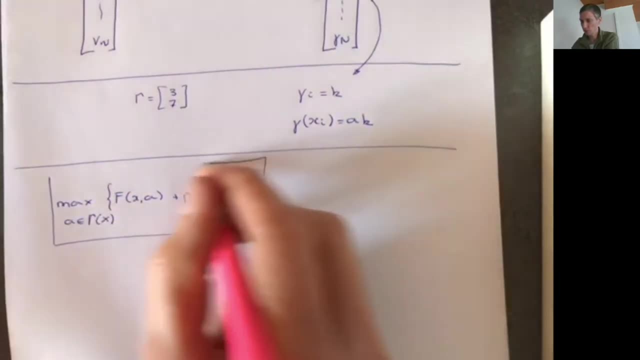 So we don't need to distinguish between x and a And we don't need to make the law of motion r, because here are the identity And in many cases you can reformulate the problem such a way. Okay, You can do it also more elaborately. 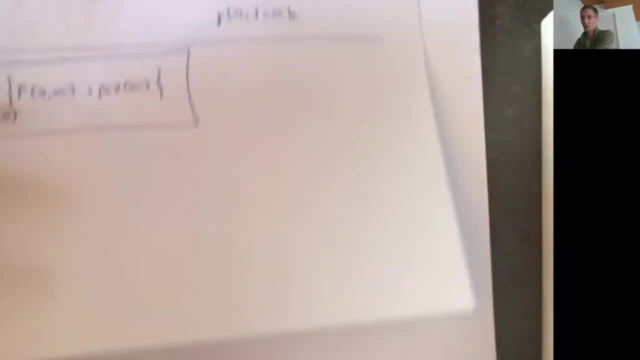 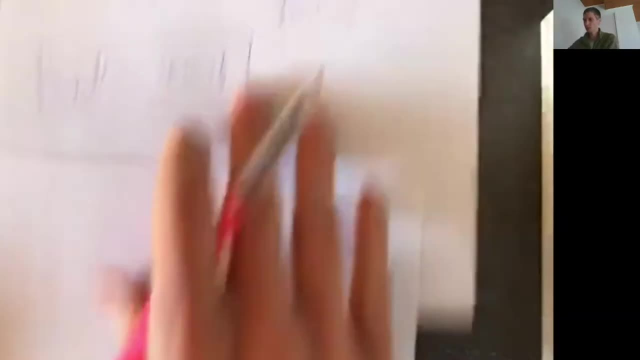 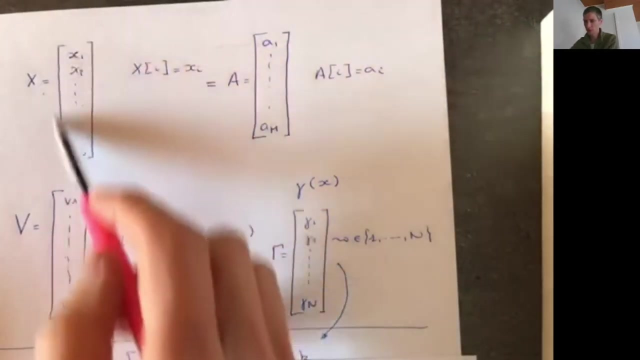 But here I'm going to look at this problem. Okay, So we're going to have to solve this problem using a computer. So here we already have our data structure: Data structure to solve. Data structure to save all the states. Data structure to save the values. 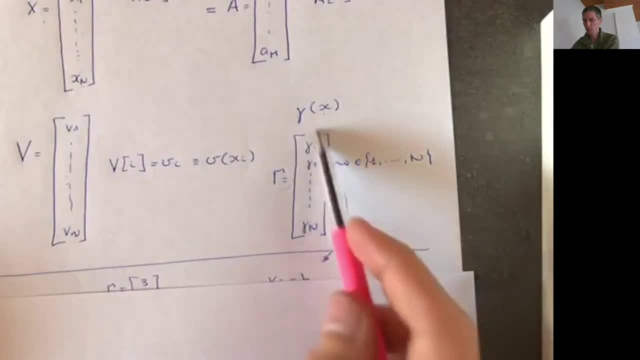 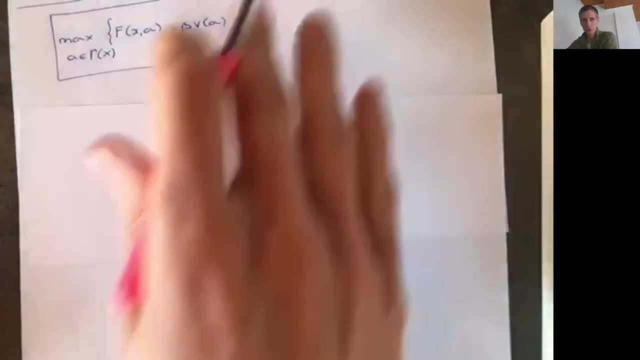 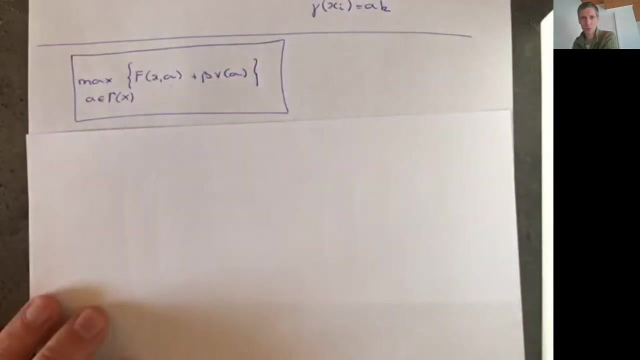 The value function, That's on iteration, And then data structure to capture the policy function. Okay, So, first thing, So this is a maximization problem. Okay, So, for every x and a possible states and possible actions, first thing that we need to do is we're going to have to evaluate it. 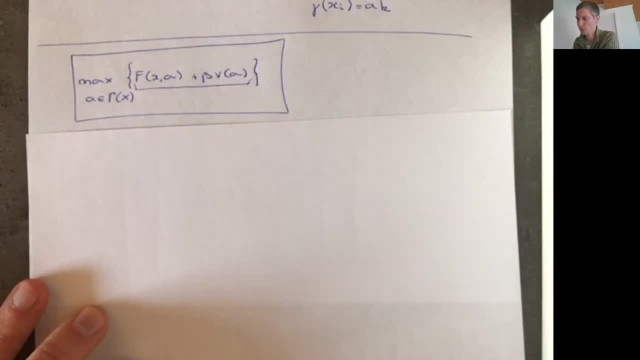 This value here, Okay. Next step: you're going to have to take the maximum of all feasible actions, Okay. And then next thing we have to do: you have to do this for every x, Okay. Once we have done this for every x, you get the new value function. 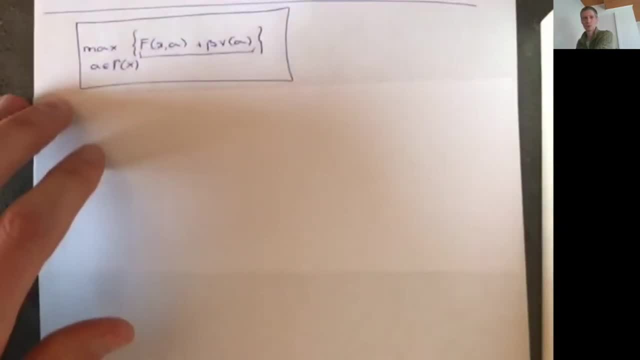 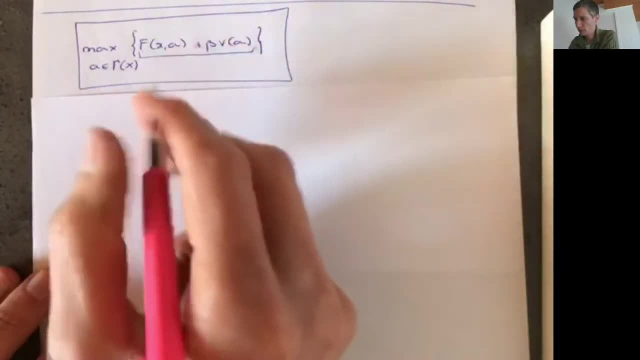 And then you have to iterate this over and over again. Okay So, let me first start by the first problem. Okay So, first let me for a given x and a, let me try to- And a given function And a given function v. 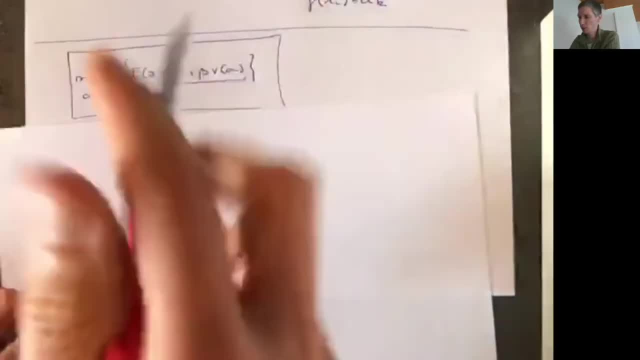 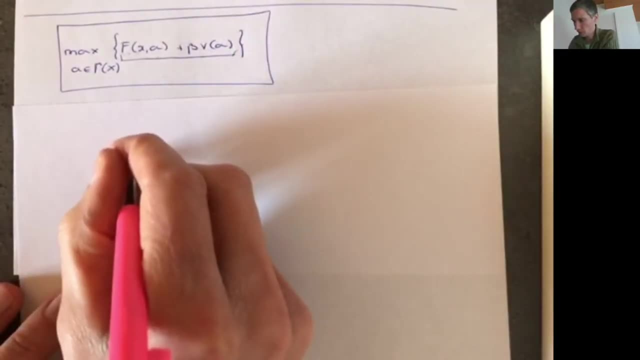 Right, Which will here be captured by a vector. Let me try to compute this value here, Okay, So this is something that you have to solve, Right? So this is going to be a function. I'm going to use some kind of pseudo code here. 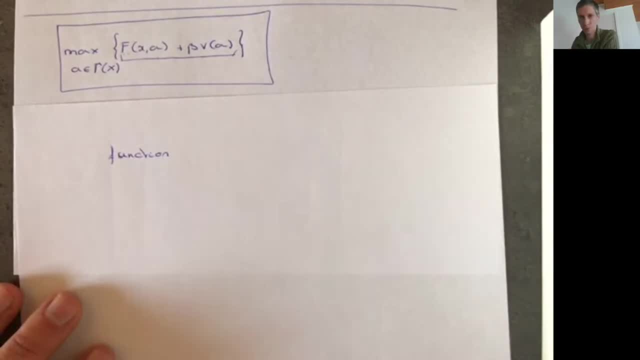 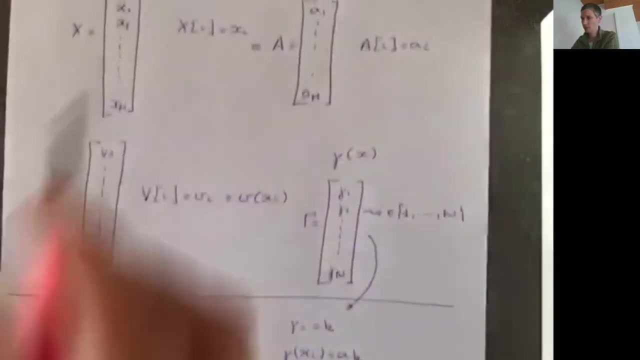 Right. So in order to get the ID straight before I start programming, So let me call this value function Right? This is a. It's going to take in A state x And a state x. I can just use the index here. 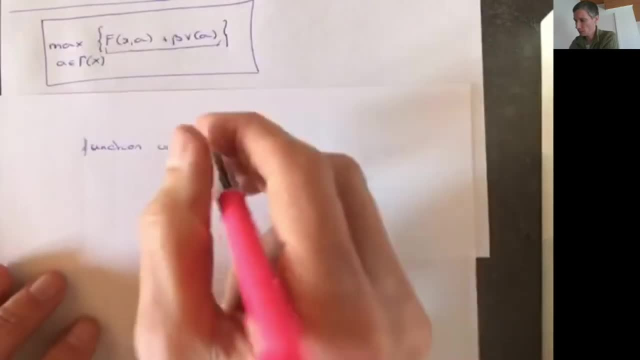 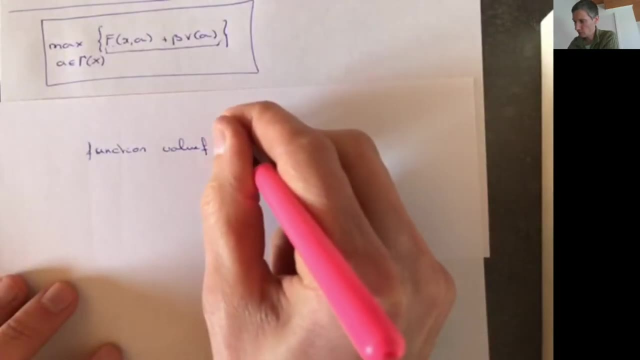 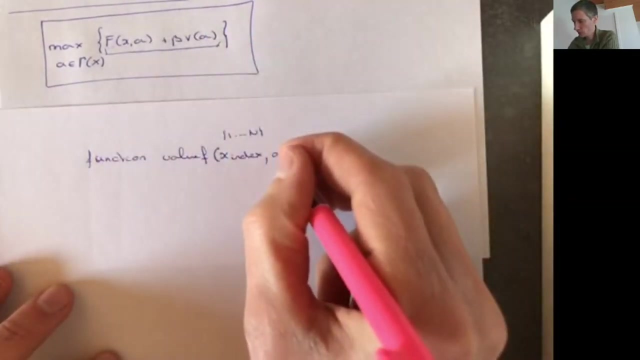 Okay. So let me call this x Index, Okay, And this is going to be a number between: Okay, Then I need to have a value of a. I'm going to call this a index, Okay, This is also a number between one and n. 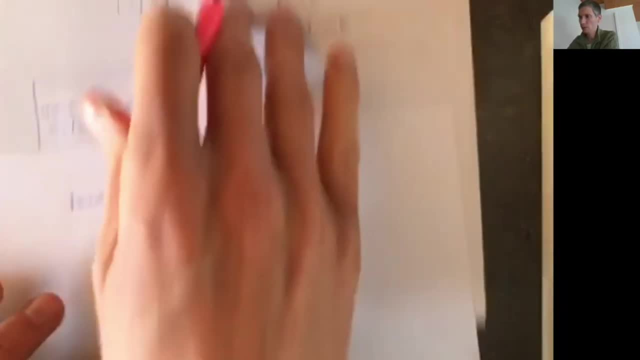 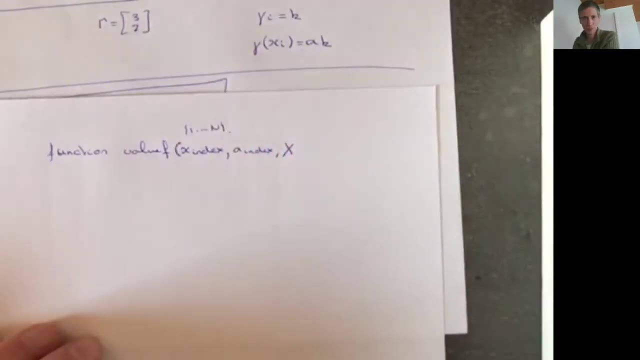 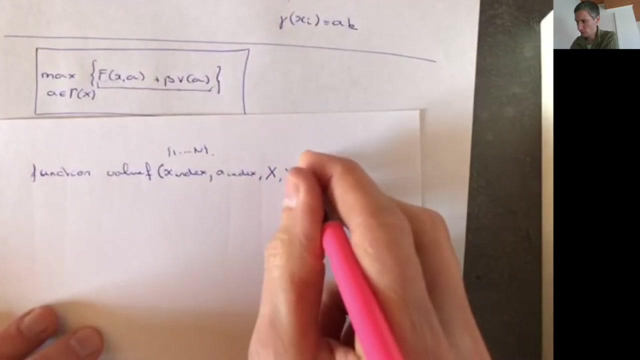 Okay, Then I'm going to have to get the value of x and a Right, So I have to somehow give it to this big vector here, This vector x, And I'm going to have to use v- Right, So I'm also going to have to use this value here. 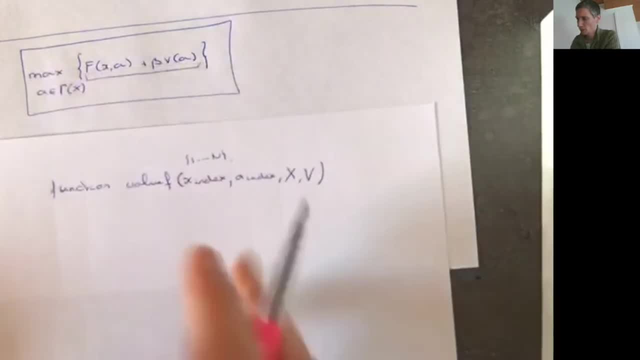 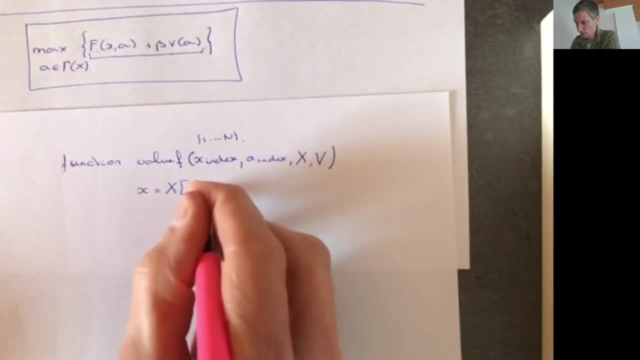 Right. So these are the inputs of my function. So If I have the x index Right, Then my x is equal to x at X and x. Okay, My a Is going to be Also my x. A is equal to x here. 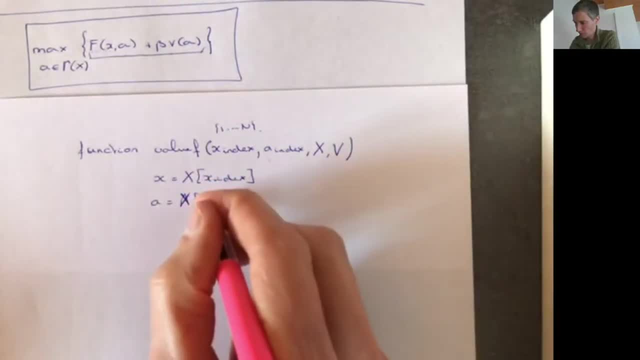 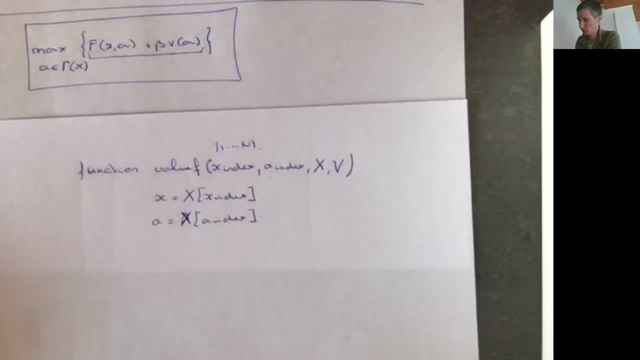 Right At a Index, And then somehow I have to Compute this. This is Not so difficult, Right? So for First of all, I have to make sure that a is in. It's not going to be g. 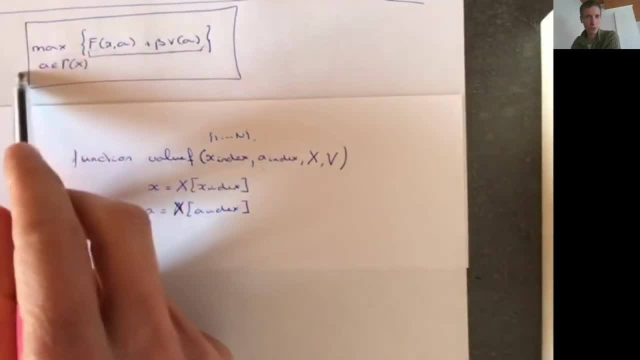 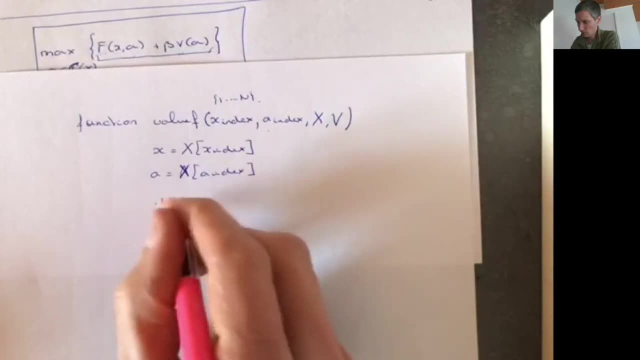 G of x, Right? So if a Is not in g of x, Right, Then I have to compute this. This is Not so difficult, Right? So for First of all, I have to make sure that a is in. 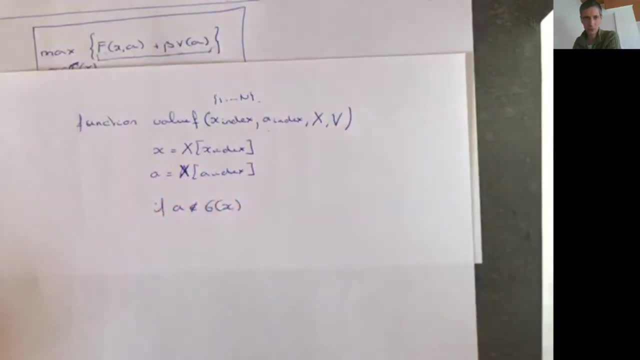 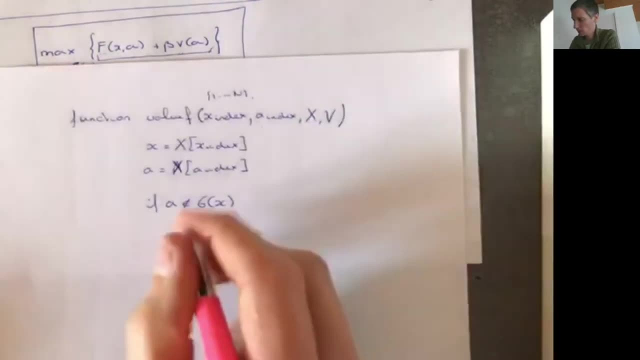 It's not gonna be g, G of x, Right, And then I have to. This depends on g of x, Right How it looks like, So I have to Write something else here Probably, Then, If a is not feasible. 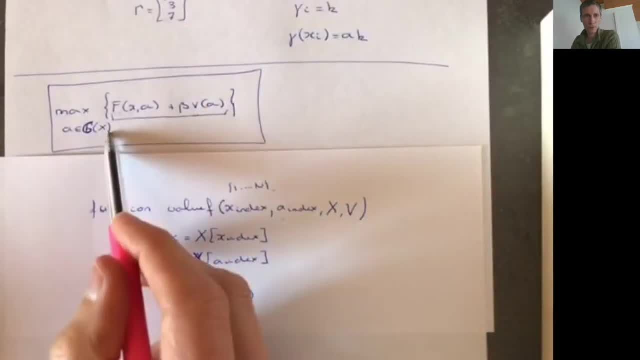 Well, What I can do. Actually, I cannot compute this Right, Because There's no value here. But one thing, Because I'm maximizing here. What I can do is I can give it a very, Very low value. 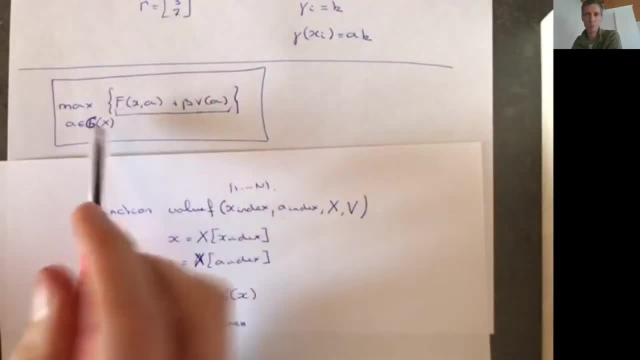 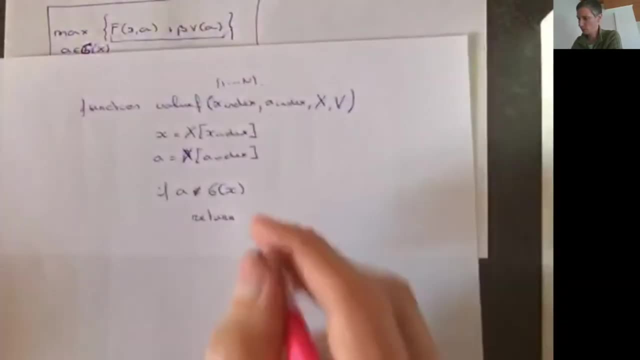 Right, Such that the maximum Will never be reached At this value. So Basically Same. So What I'm doing Is just Giving it a very low value. Okay, So Here I'm going to return. 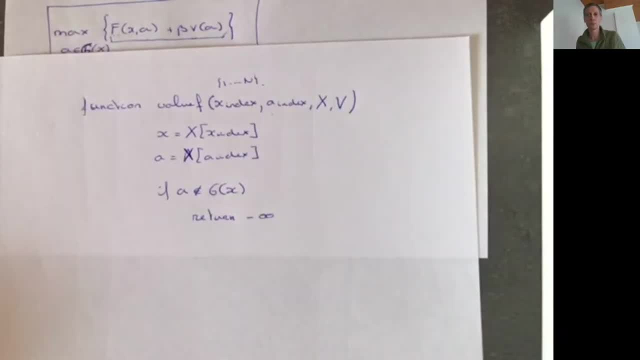 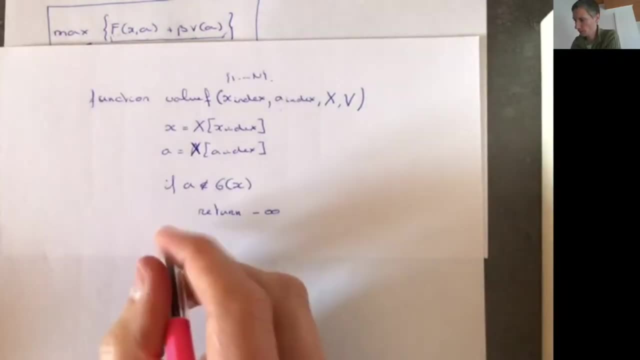 Minus infinity. So Minus infinity Doesn't exist on the computer, But you, In Several software packages You can use it. So This is what I'm going to do here. It's just a very, Very big. 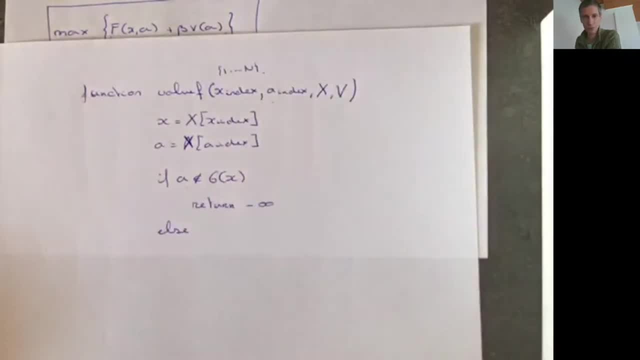 Negative number, Okay. So If it is feasible, So Else, Then I'm going to return F, F, X, A Plus Beta Times V Right And Here V At A. 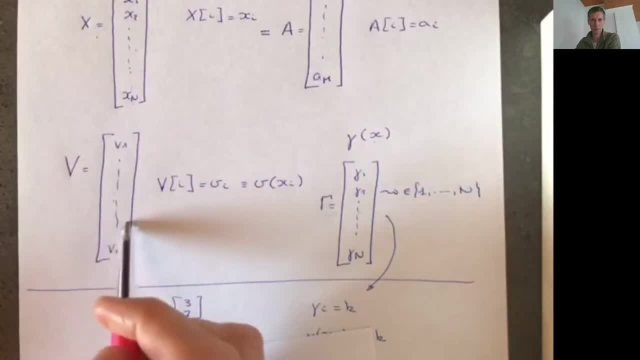 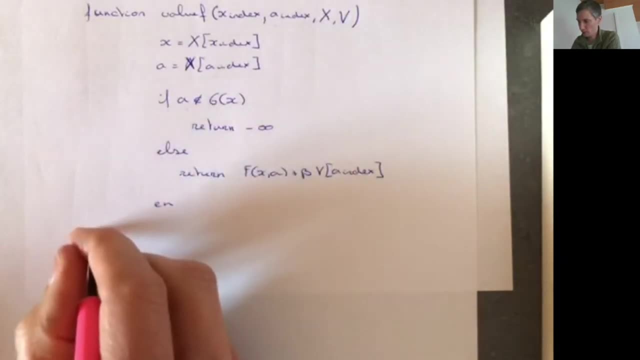 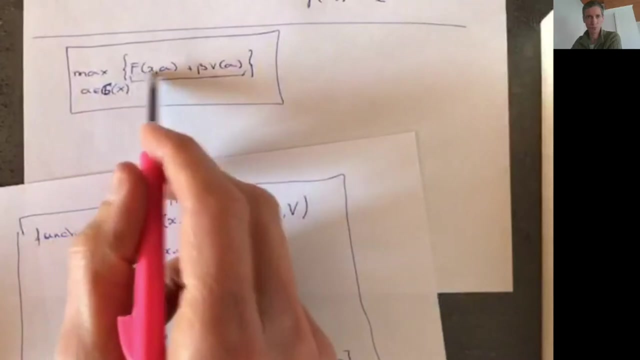 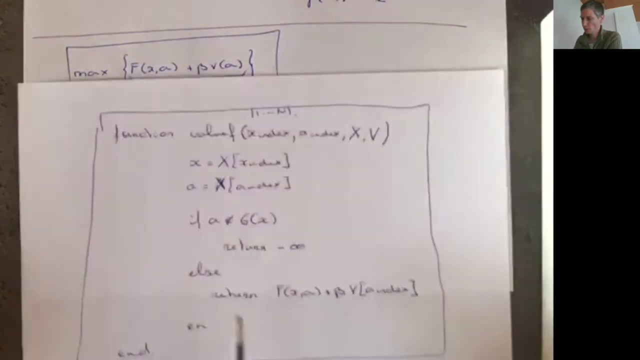 Right, So This Is Each Element Of V. Well, It's The One For The Next State, So I Can Use To Compute This Thing Here. 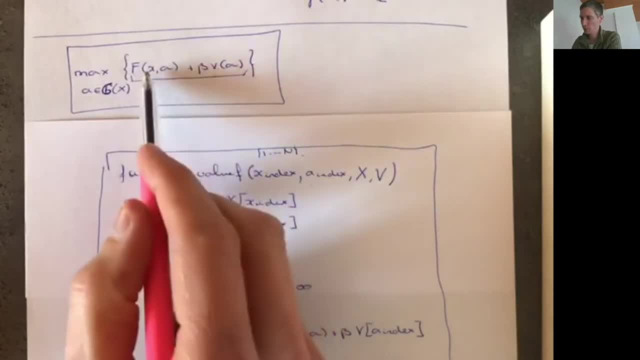 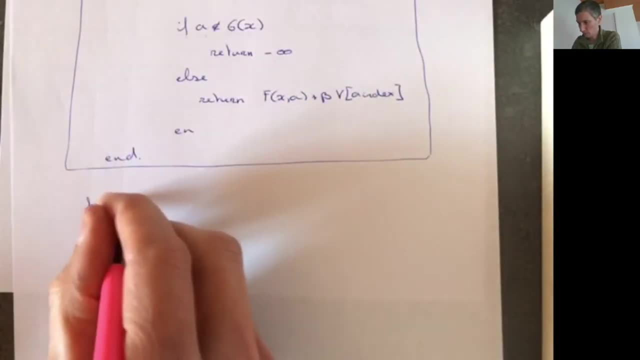 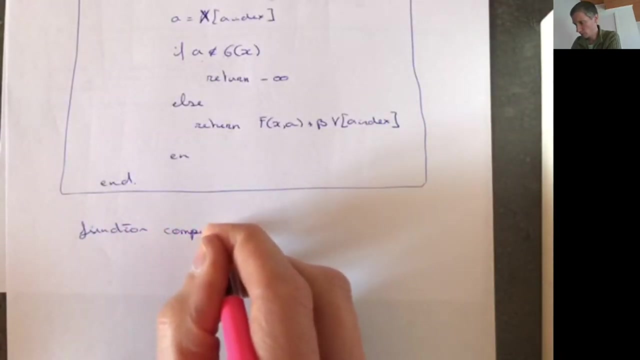 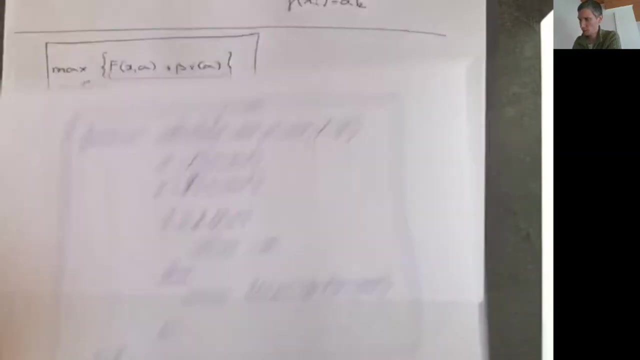 Okay Now, So I Can Evaluate This For Every A. The Next Thing Would Be For A Given X To Compute. Okay, So What Do I? 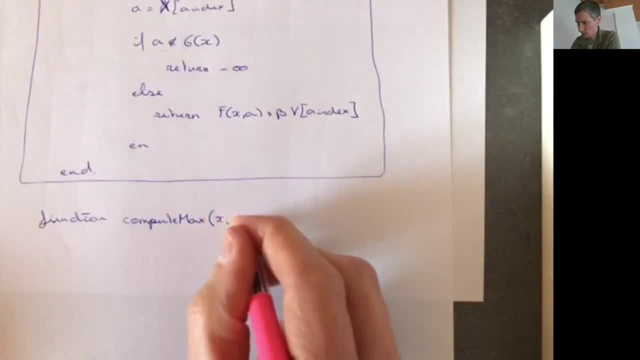 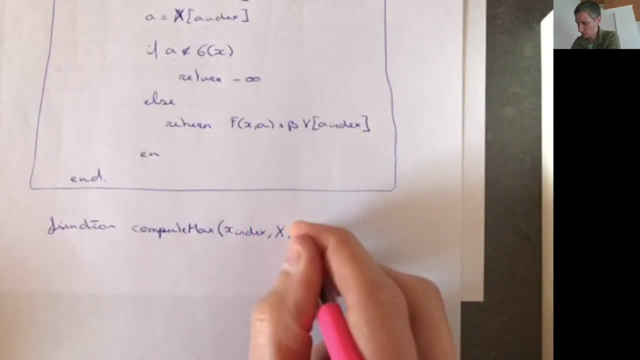 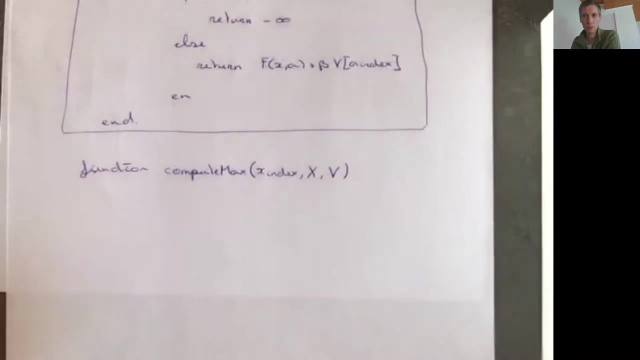 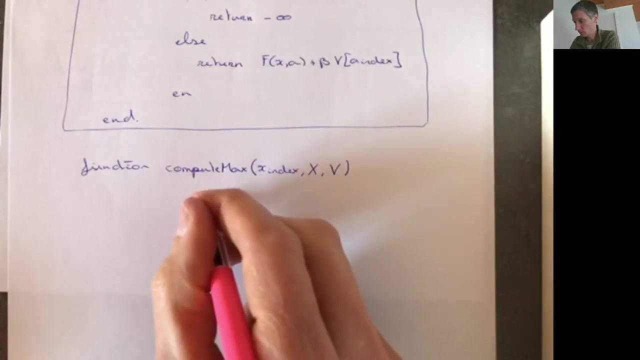 Need. Well, I Will Need To Have A State Right. So X And X, And Then I Probably Also Need X And I Probably Need To. 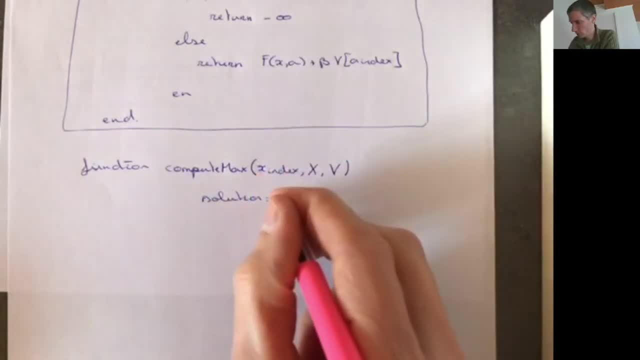 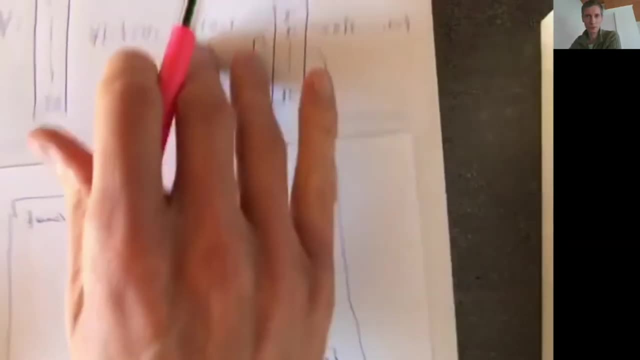 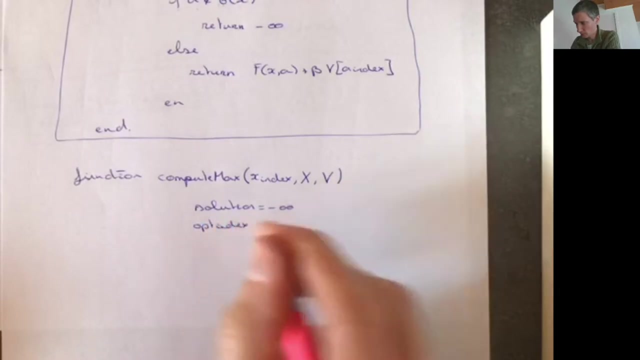 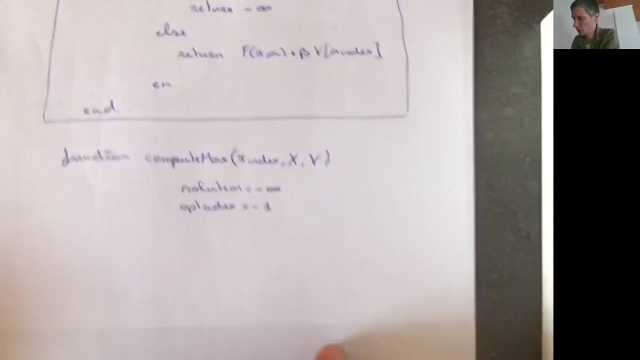 Have A Solution Right, And I Can Put It At Minus Infinity To Start, And I Can- I Probably Also Want To Store This Thing. 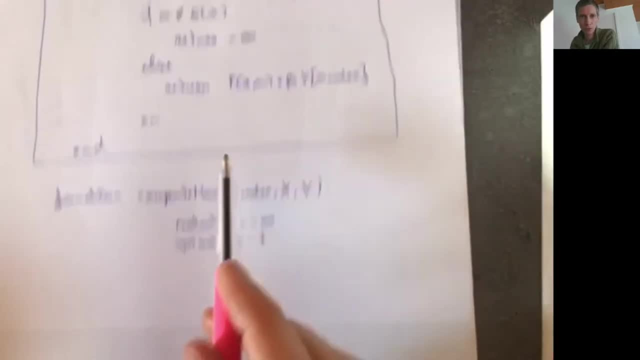 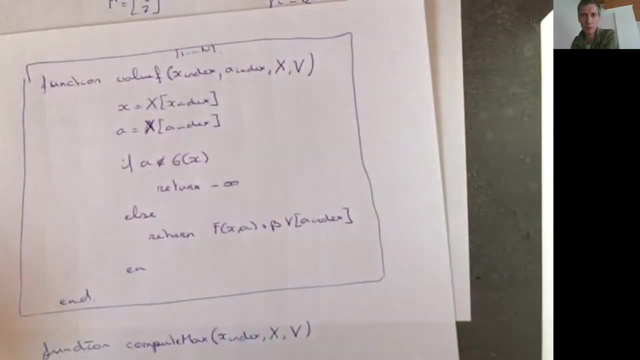 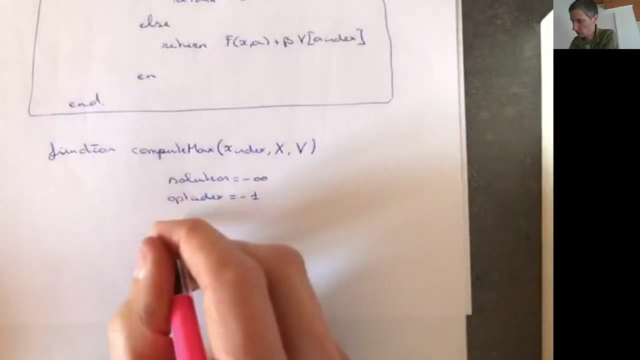 Here. The Ease You Could Do Is You Can It At All Possible Indices Each Time, Compute This One And If I Get A Higher Value, 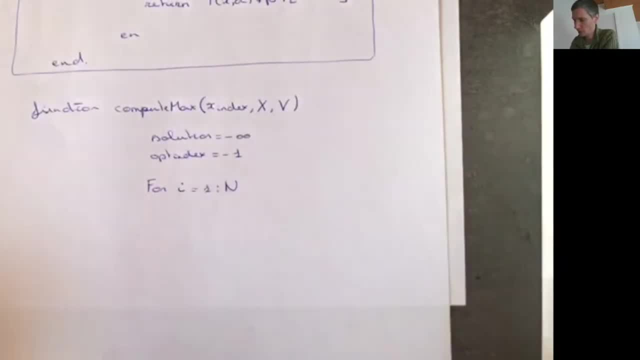 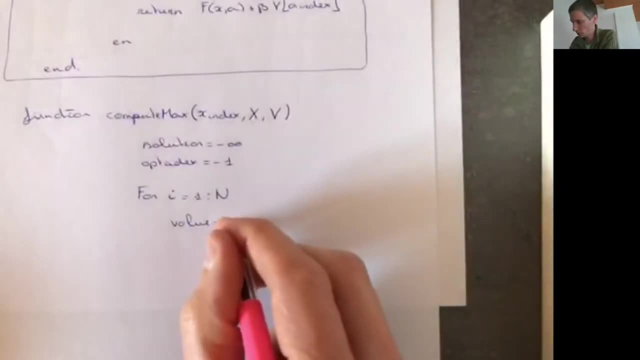 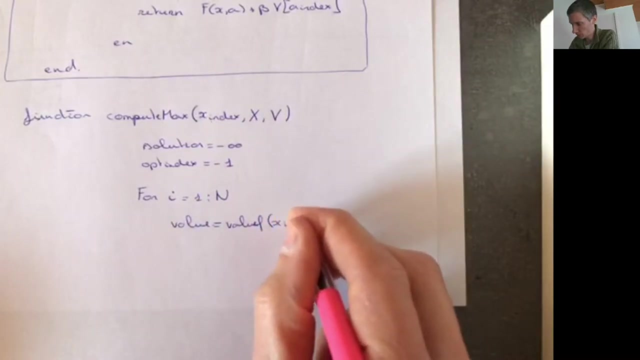 Then I'm Going To Update, can compute value. this is going to me, this function here, value f of what of this? at this point, x index, my a index is going to be i. then i'm going to have to give it a value x. 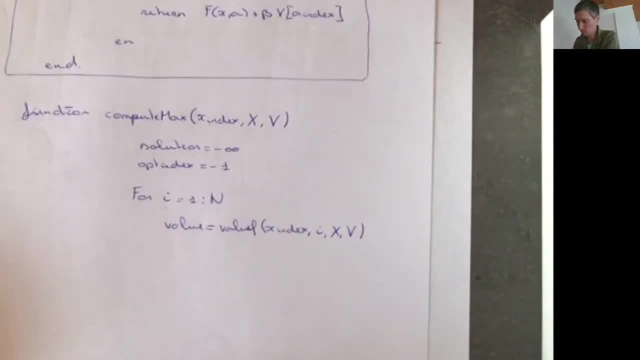 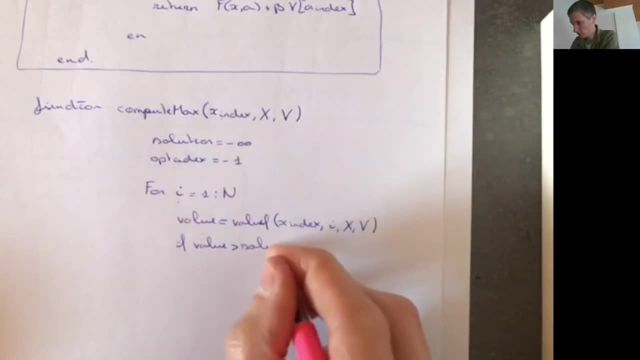 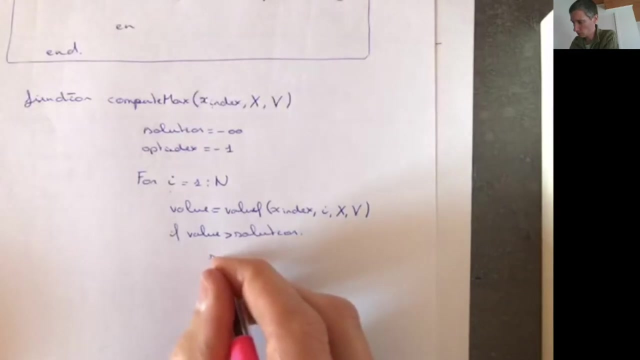 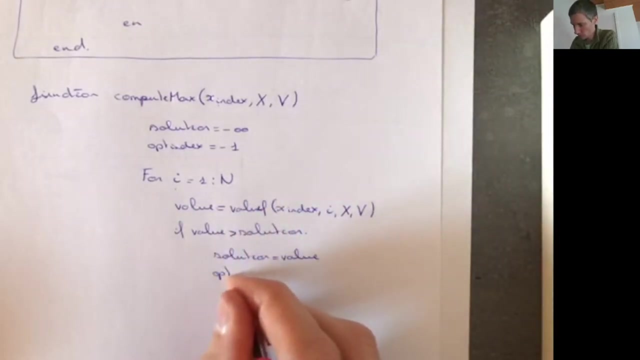 and i'm going to have to give it a value v, okay, and then if the value is bigger than solution, right. so i have found a value that's that's better than the solution i have until now. i'm going to put solution equal to value and also going to put opt index equal to i here. 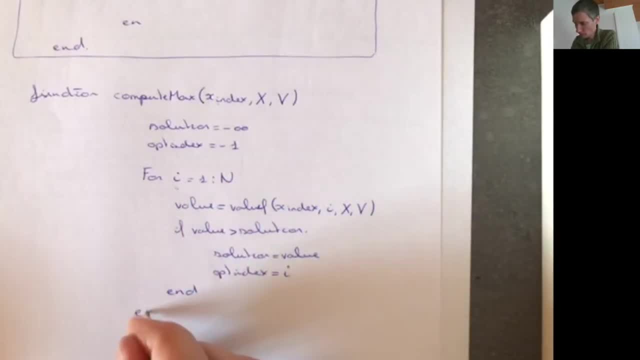 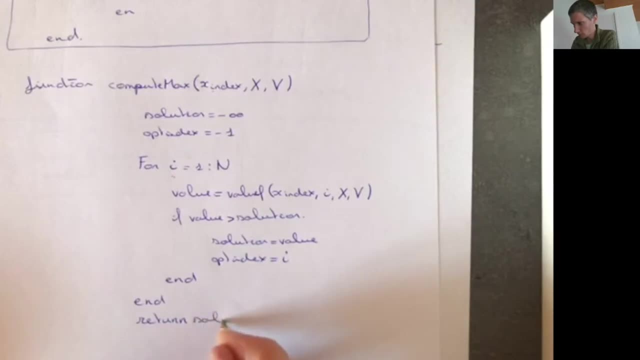 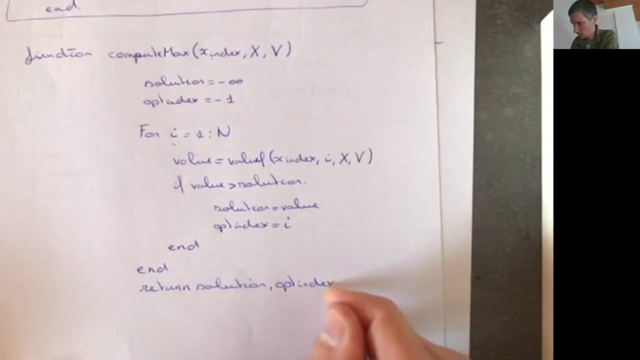 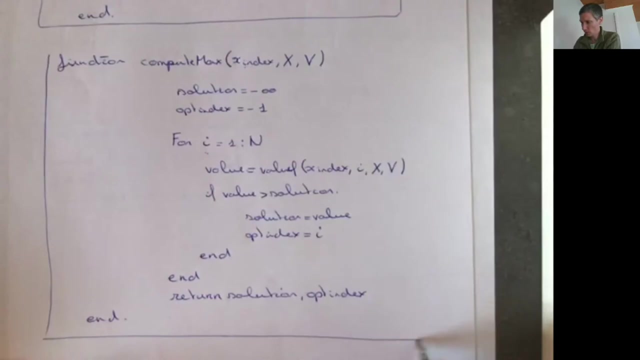 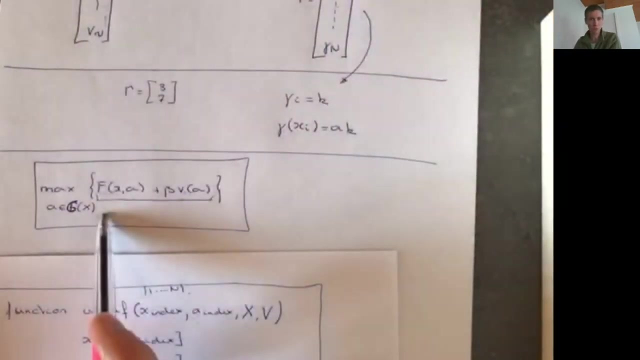 i'm going to end this and this and then i'm going to return solution and i'm going to also return optimal index. okay, and this is going to end my function. so now, if i run this function for a given x index, i'm going to solve this maximization. 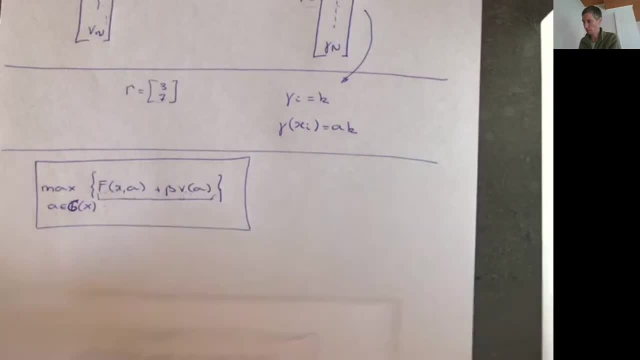 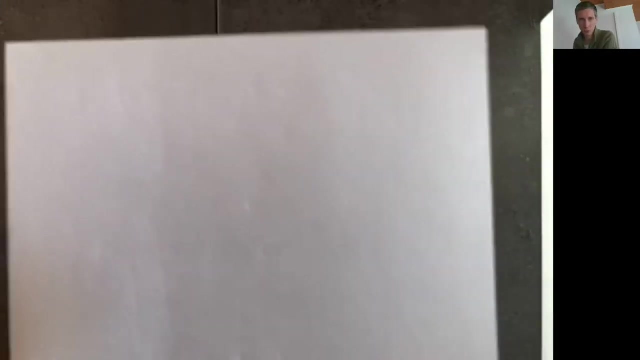 problem for this x here. okay, so the thing is, i have to do this for every x, right, because i want to have my tv. okay, of x, which is the next iterator. okay, so i can do this using a new function. maybe i can call this, um what i've called it: value function- complete max. maybe i can. 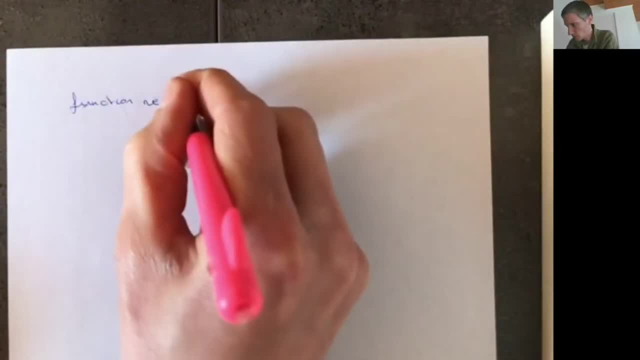 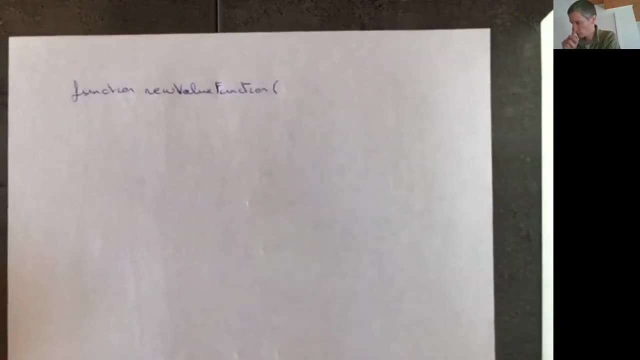 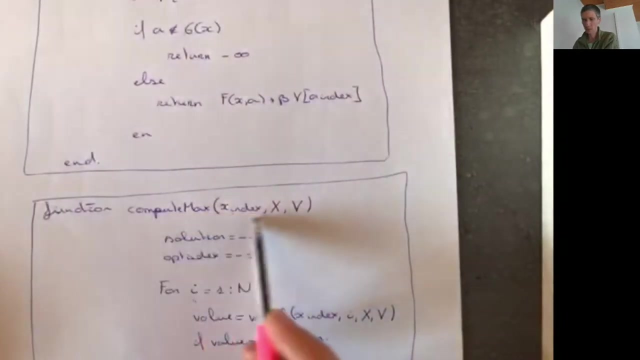 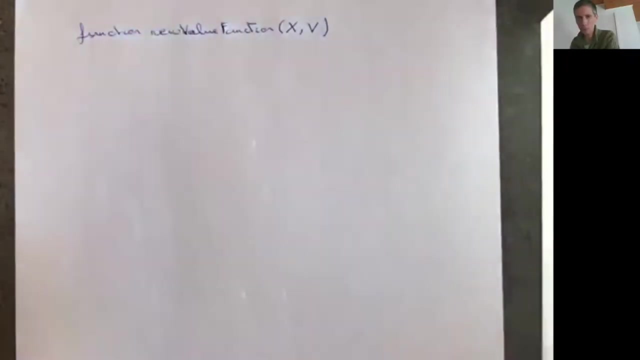 call this new value function. okay, so now i need a set of states and i will probably also need a vector v of the current value function, and what i need to do is, well, basically i need to iterate. i need to iterate this over all possible values of x. okay, so i will have to need to store the new value function into something right? so 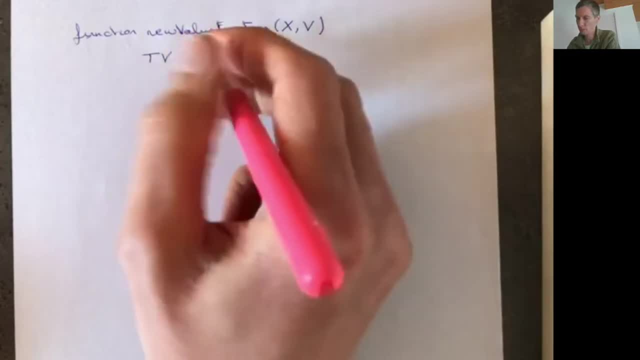 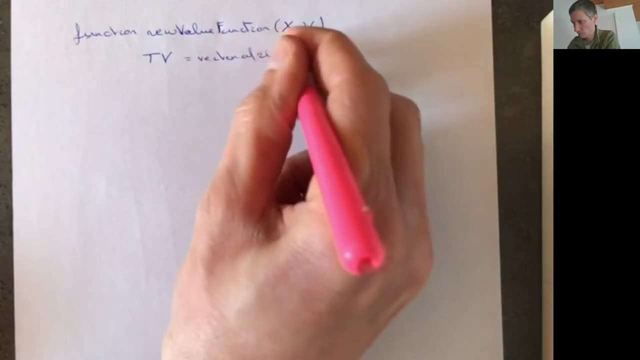 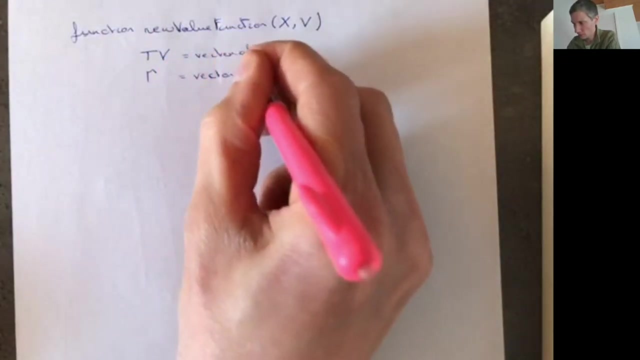 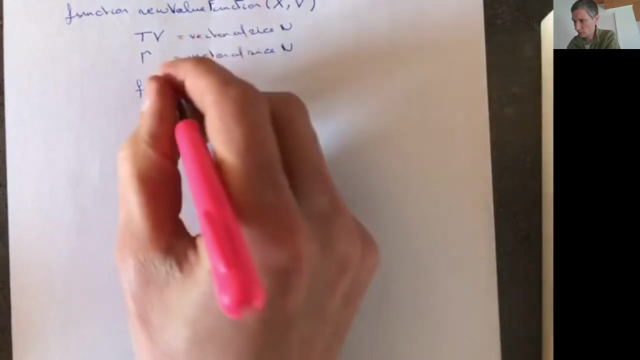 this tv is going to be just a vector of size n. i'm going to get a solution- is also going to be a vector of size n, okay, and then i'm going for. let me call it i equal from one completely to moment. Proper Vector representing v and. 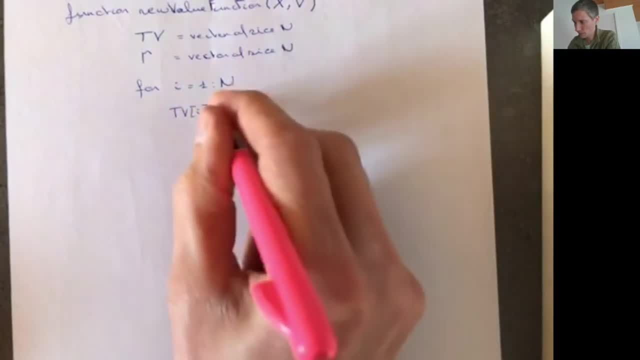 n about d. v is dalej again and gamma i is going to be equal to multiplicative i people from one to n, d. now I'll just wait and favorite that function for some reason, because it's going to be picked right. but I'll do it with the certain thing that I'll tell you right now, because today we don't. 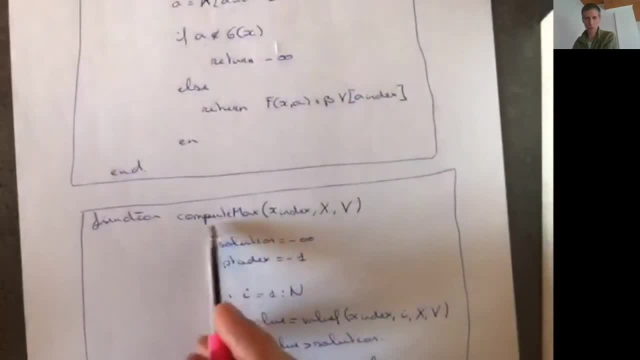 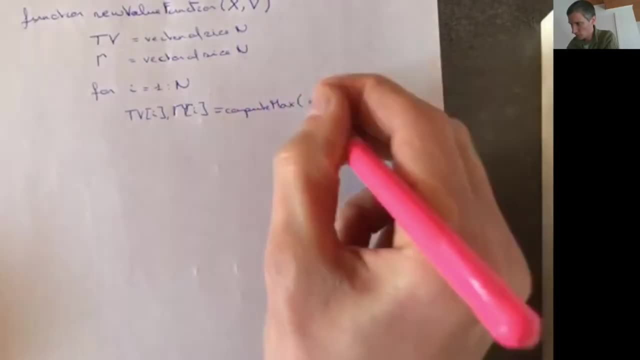 have to live by anything other than a query, while the tag bed now use a function of using the function command confidently or just leave the simple. will we to close the code? click off is go with to this function here, computeMax, of which, well, the index for the state my, 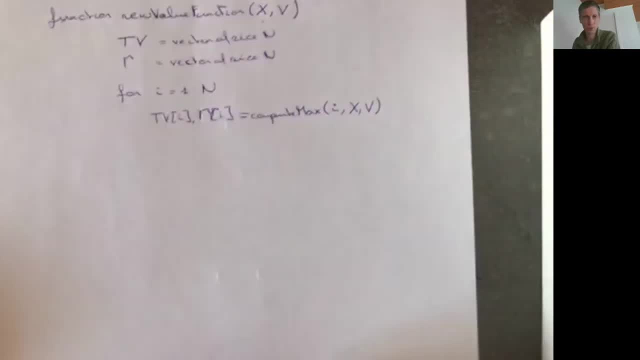 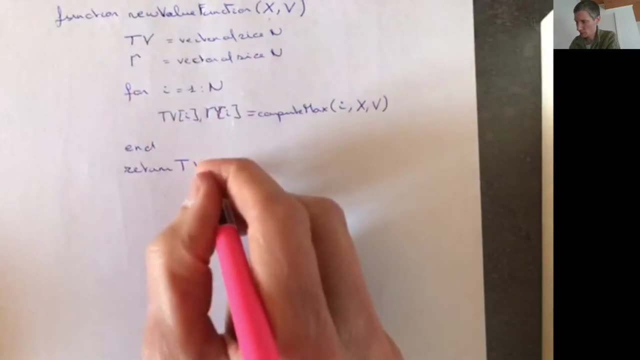 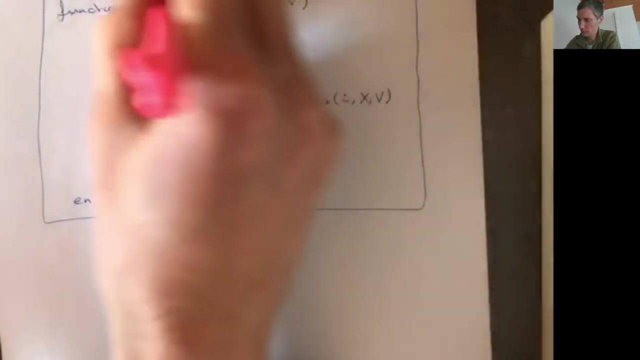 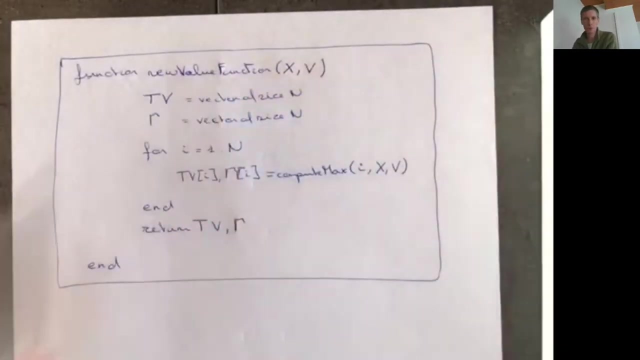 vector of states and the value function. okay, this is going to end and I'm going to return this entire vector here, then my gamma here, so this is going to be my third function. okay, so far, so good. so now, finally, I'm almost done. I need one. 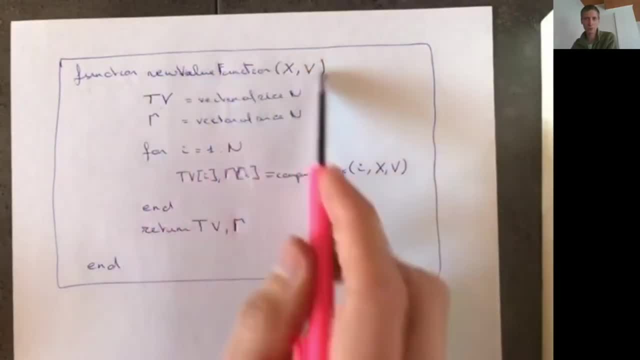 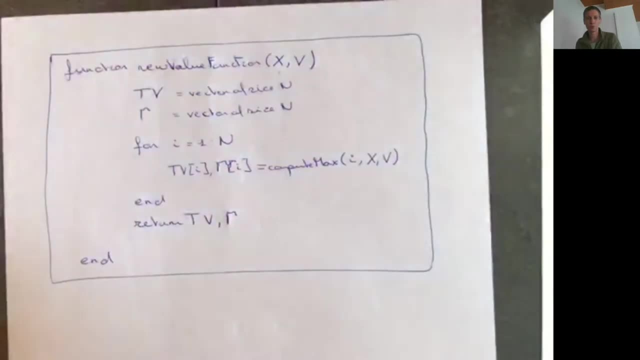 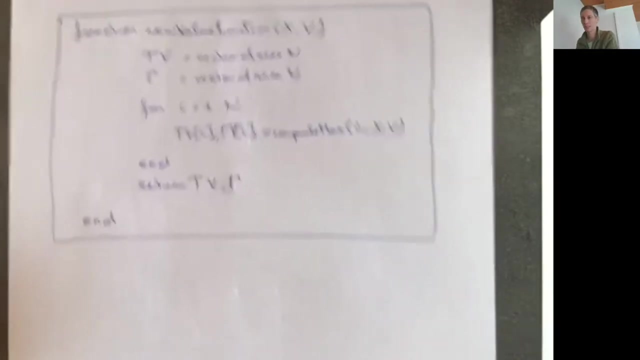 more function. basically, I have to iterate this over and over and over until I get the fixed points. okay, so how will I know that I'm at the fixed point? well, I in principle, you never will reach the fixed point. right, you will get closer and closer and closer to the fixed point, but you will never get there. 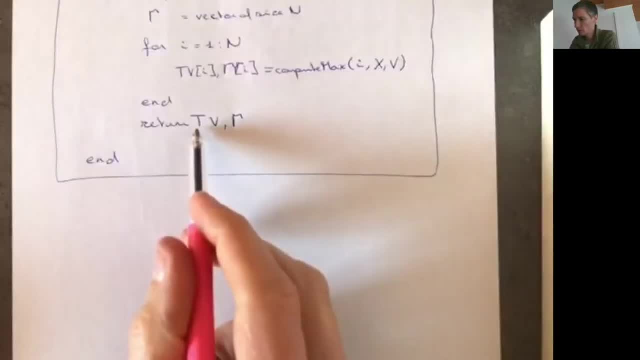 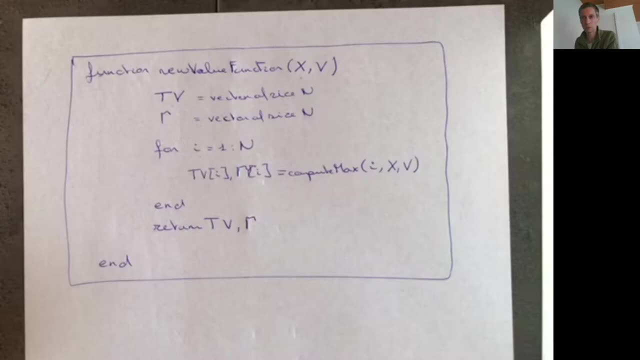 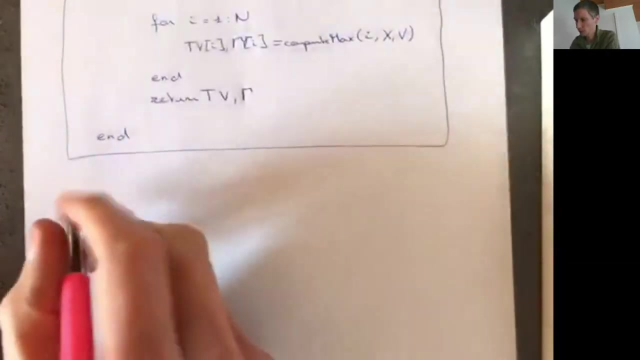 in the end, probably, so what are we going to do? we're going to iterate this over and over again and we're going to measure the distance from the next iteration to the previous one, and if this distance is smaller than some very, very small number, then we're going to stop the algorithm. okay, so let me get my 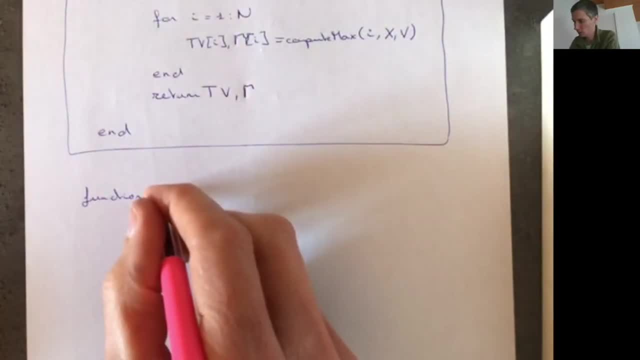 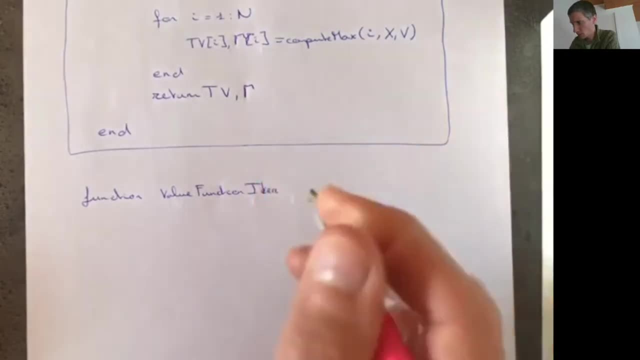 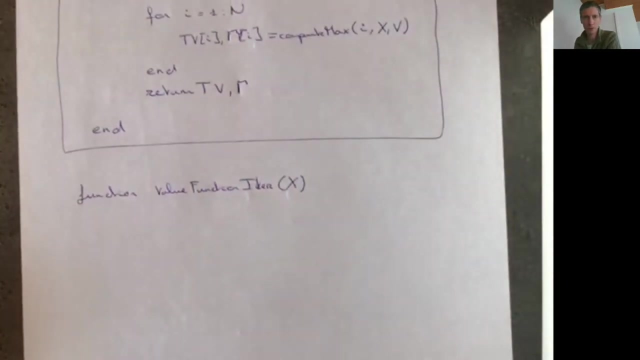 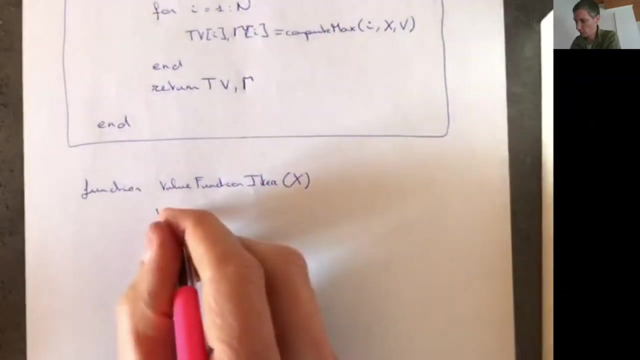 function. let me call this value function iteration. so what do I need as inputs? well, basically, I only need my states here, right? then I'm going to be have to make a vector values, right? I'm gonna have to loop over each time computing a new vector. so let me call this a vector. 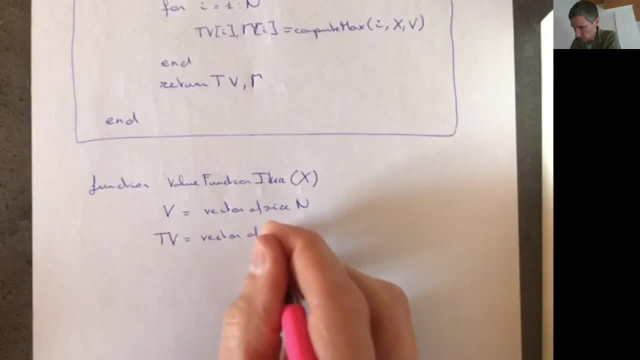 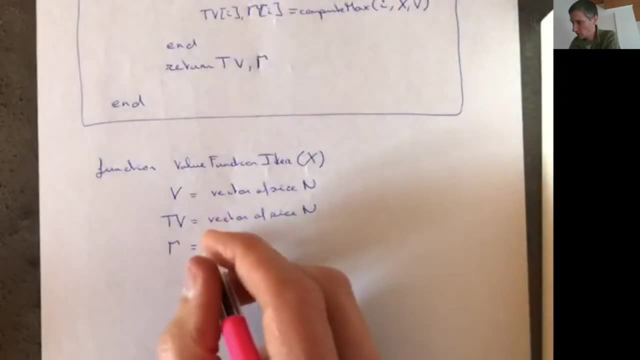 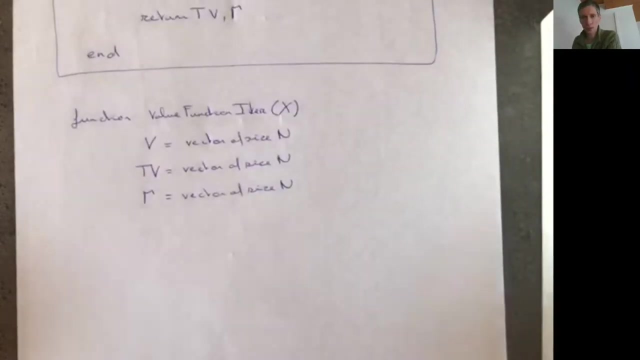 TV, okay, and then I'm gonna have to get my solution. vector is also a vector of size, and okay, then let me call something to capture or to compute the distance between this one and this one over each iteration, and let me just put it at some big number. at the moment I don't know. let's say that right, as long as it's. 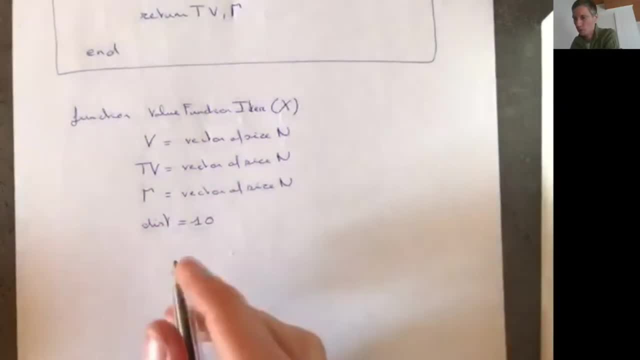 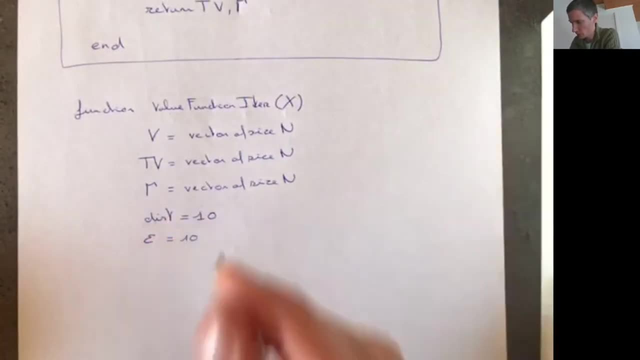 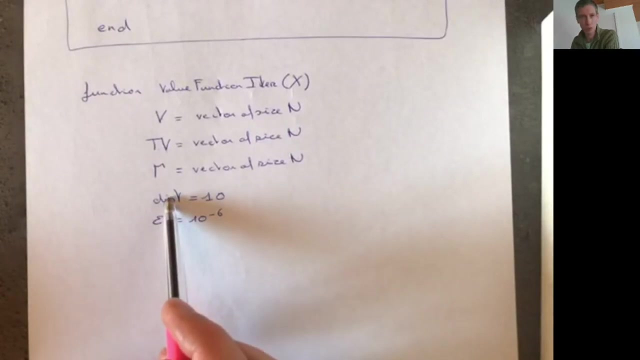 big enough and I'm going to introduce some very small number. let me call this epsilon. it's, for example, 10 to the minus 6, right. so it's a very small number. so what I'm going to do, at each iteration, I'm going to compute the distance. 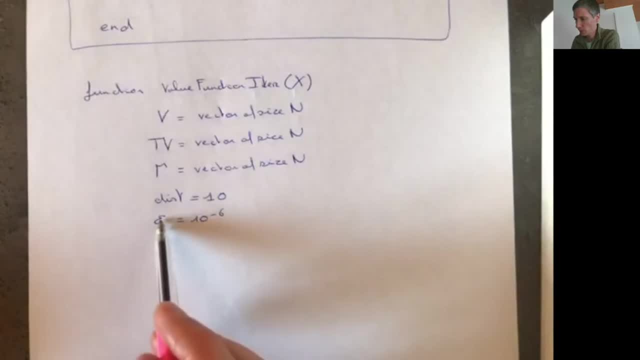 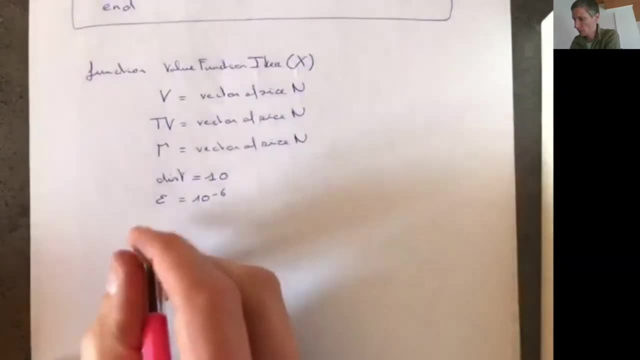 between this and this vector. okay, and as soon as the distance is below this epsilon, I'm going to stop the algorithm and just give the solution here. okay, so this is going to be a while loop, right? I'm going to iterate until some condition is satisfied. well, until as soon as distance is below epsilon, I'm 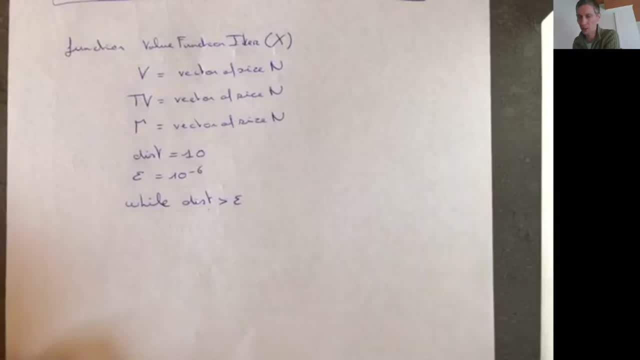 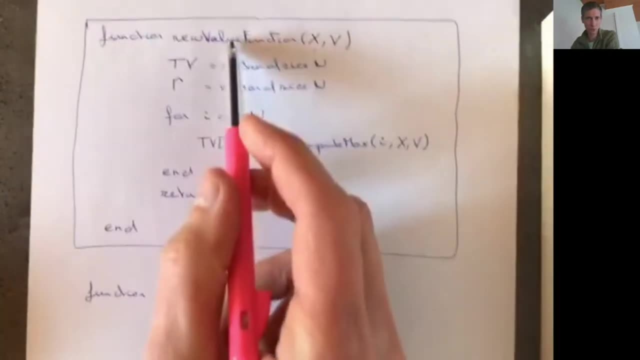 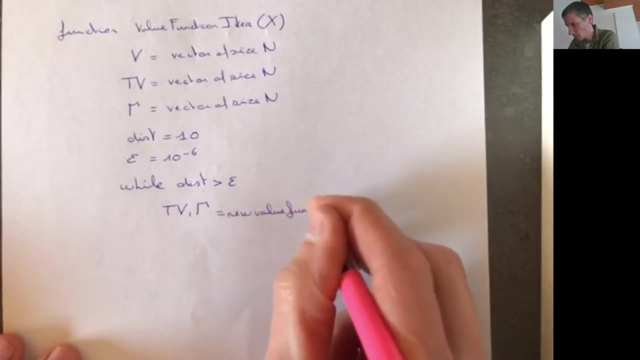 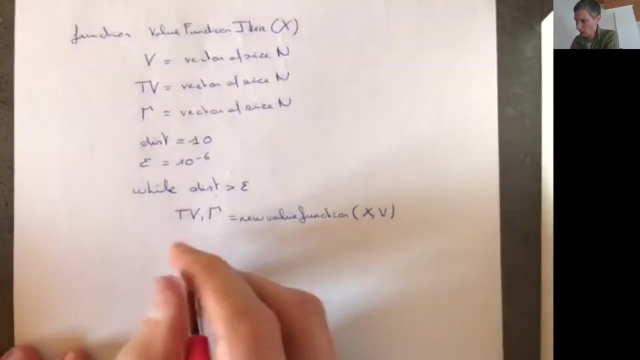 going to stop. okay, so, while distance is still bigger than epsilon, I'm going to set TV and gamma to be equal to what? well, here, new value: function of X and V. okay, then, what I'm going to do, I'm going to compute. distance is going to be equal to the. what I can do is I can take the infinity norm of TV. 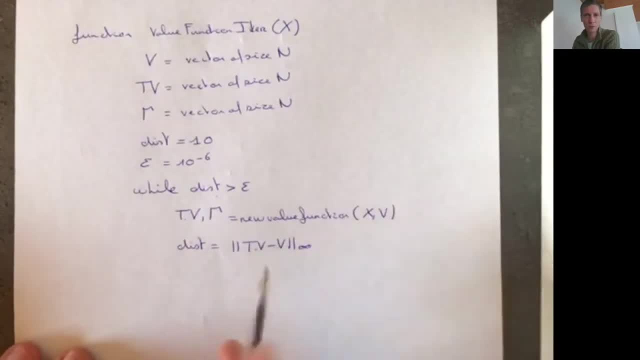 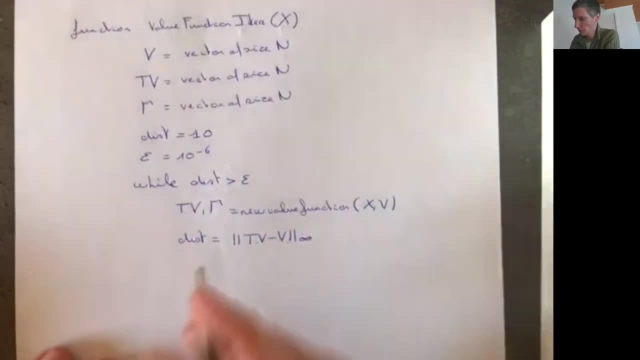 and V, right? so this is maximum of the difference between these two vectors. okay, the maximum of the absolute value of t. okay, the maximum of the absolute value of t. okay, the maximum of the absolute value of t of the distance between these two vectors. and then what i'm going to have to do is, if this distance is still bigger than, 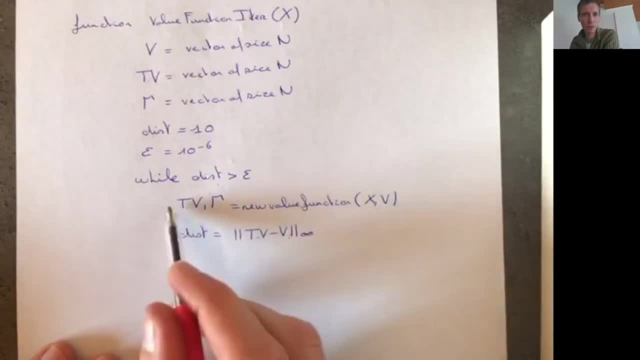 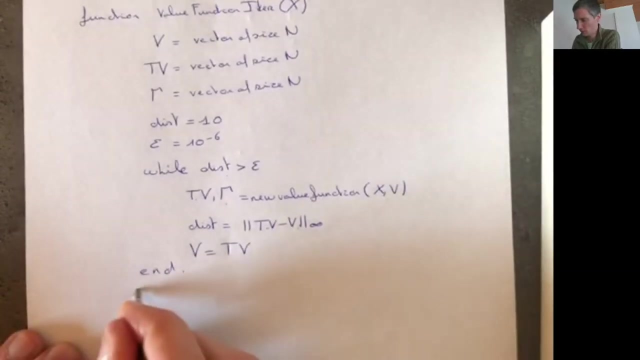 epsilon, i'm going to have to iterate this, but now tv will be here and the new tv will be here, right? so i'm gonna have to set v equal to tv in order to get the new loop started. okay, so this updates the value of v, so i'm going to end this and then 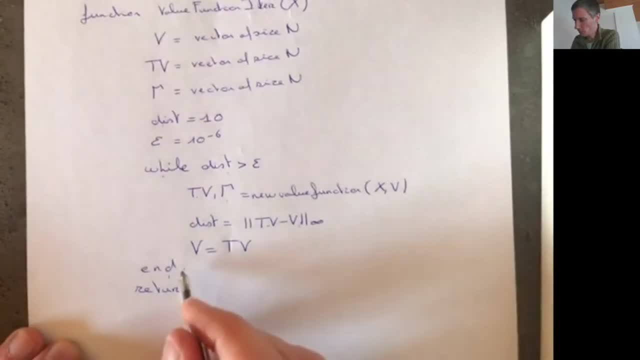 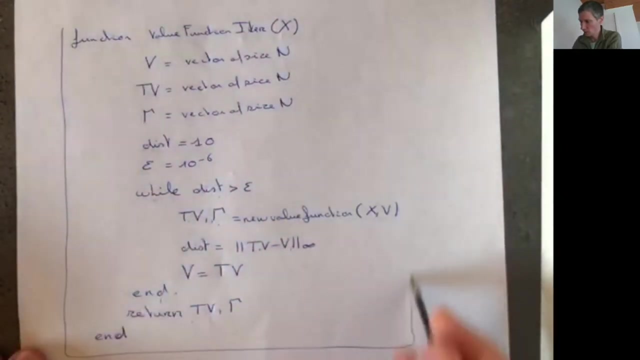 once i exit the loop, what i'm going to do is i'm going to return tv and i'm going to return the last value of gamma here, okay, and i'm going to to end this function. okay, so this is going to be my value function- iteration- okay. so here i split it up and 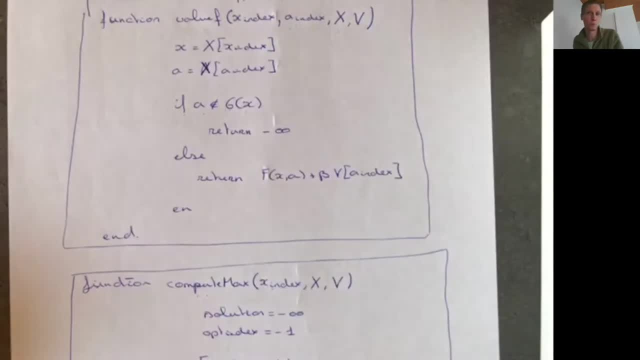 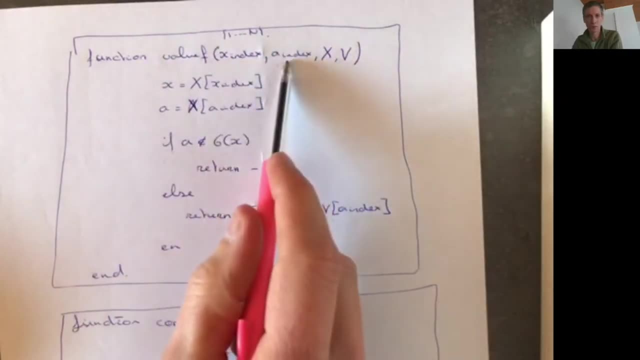 in principle, you can put everything in one big function- okay, which is also reasonably valid, but here i try to split it up and into a function that computes for a given state and a given action, the, the function you want to optimize then, for a given state, this is going to: 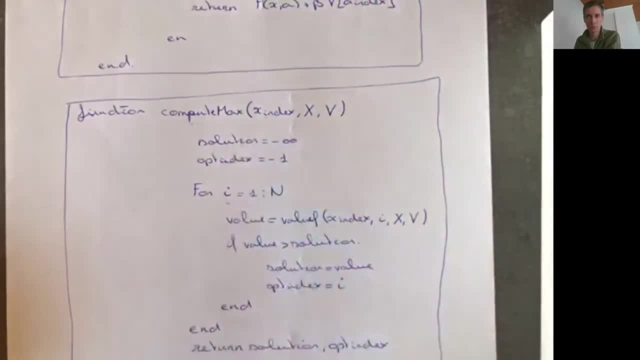 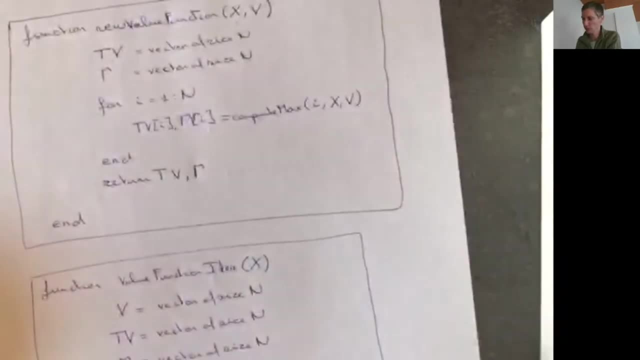 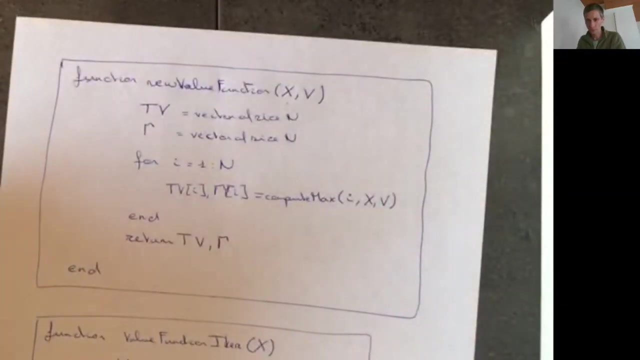 give you the maximum value, all right. then this is going to compute your new value function right over all states, and then this one is going to iterate the loop over and over again until you hit the fixed point. okay, so in order to implement this on the computer, i'm going to focus on one. 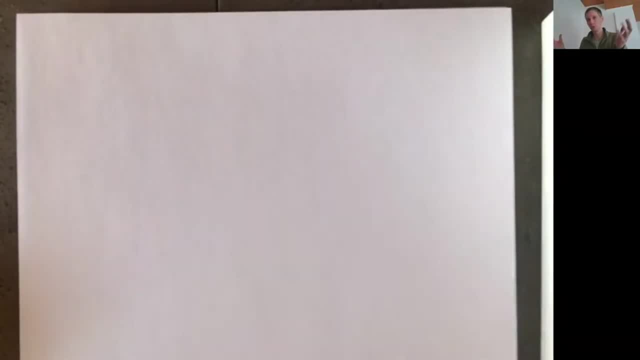 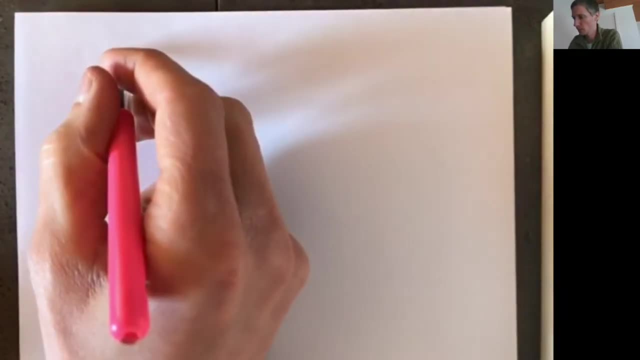 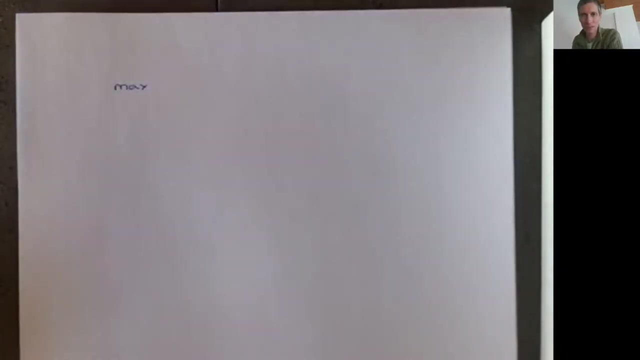 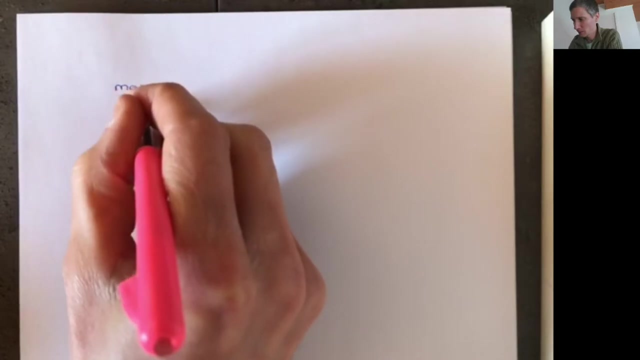 particular problem. right, i'm not going to look at the general function f and so on. no, i'm going to look at a growth model. okay, that's the the name. so, in principle, i'm going to look at a consumption capital stock trade-off model. so i'm going to maximize c in zero. now i'm going to have to use a. 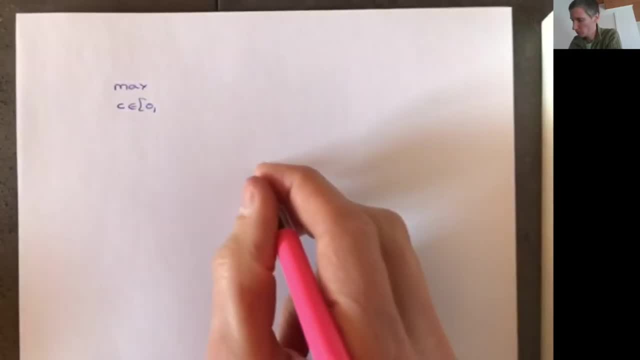 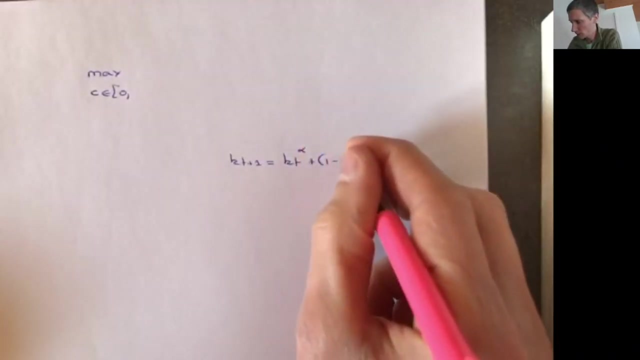 production function. so i'm going to use a law of motion where kt plus 1 is equal to kt, let's say to the power alpha. i'm going to give a value of alpha in a minute, and then there's some one minus delta times kt. right, so a fraction, one minus delta of the 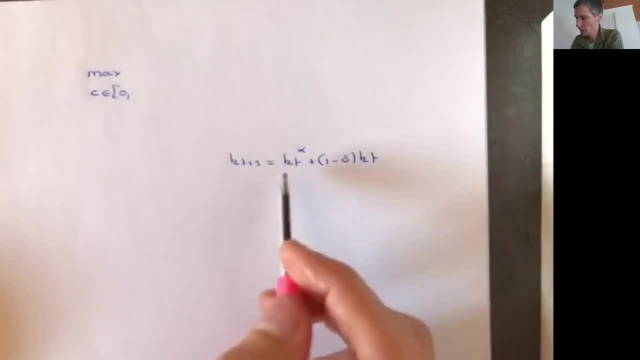 capital stock today gets into the capital stock of tomorrow and then, using the capital stock today, i'm going to be able to produce a production function. so i'm going to use some output, and then, of course, i'm going to consume something. okay, so i'm using ct. 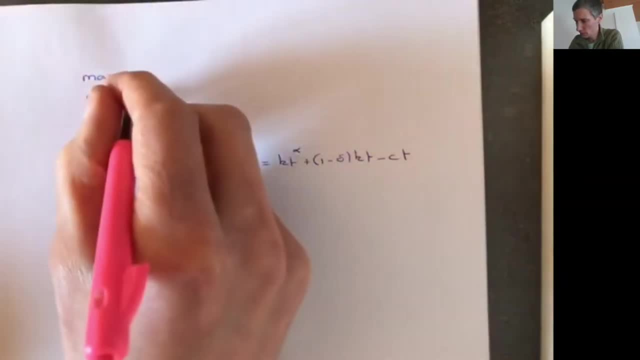 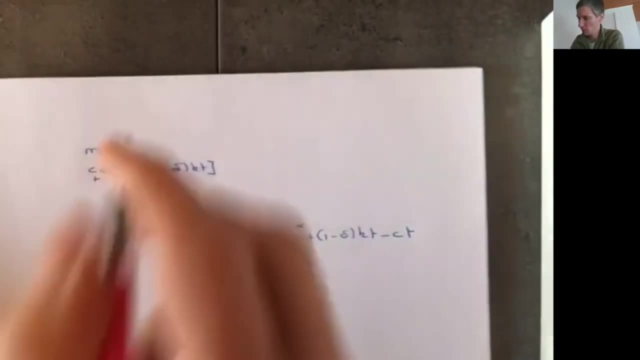 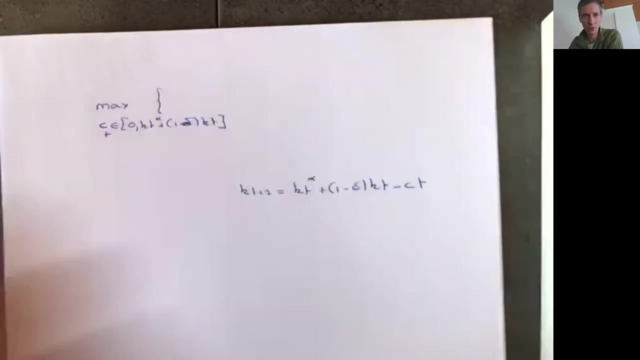 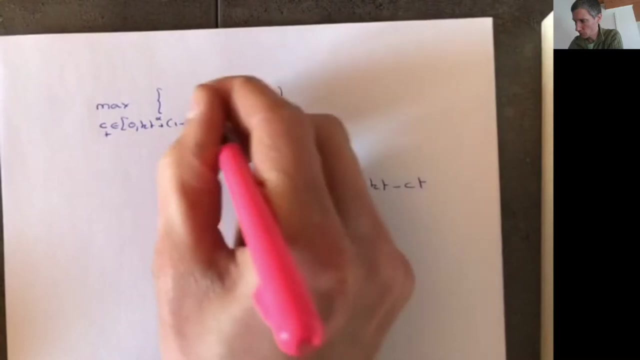 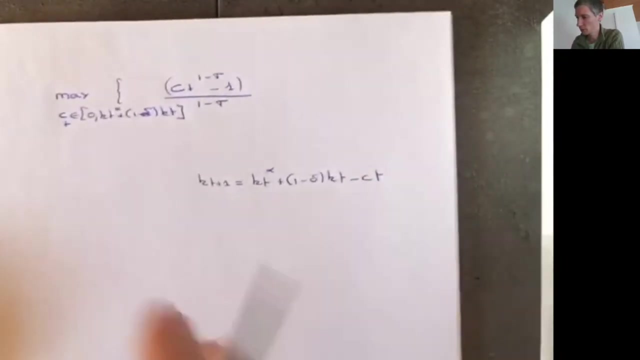 ct is going to be between zero and kt, alpha plus one minus delta kt. okay, and then, as a utility function, i'm going to use a ces utility function. so this is ct: one minus sigma minus one divided by one minus sigma. okay, so this is a standard concave utility function. 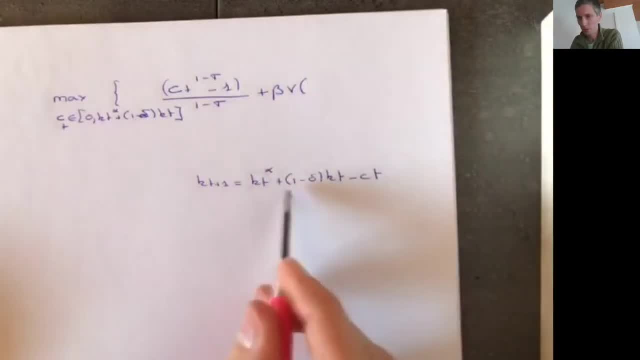 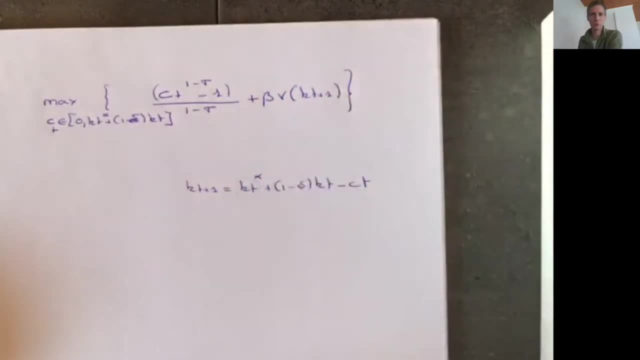 plus beta, and then v, and this is going to be kt plus one. okay, so this is my bellman equation, given this law of motion, right? so instead of writing kt plus one, i could have just also substituted this in here. so the first thing i'm going to try to: 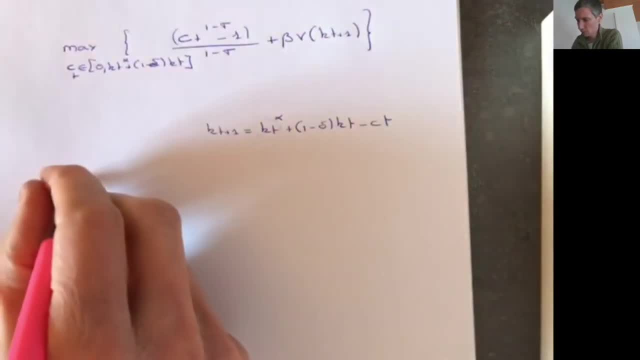 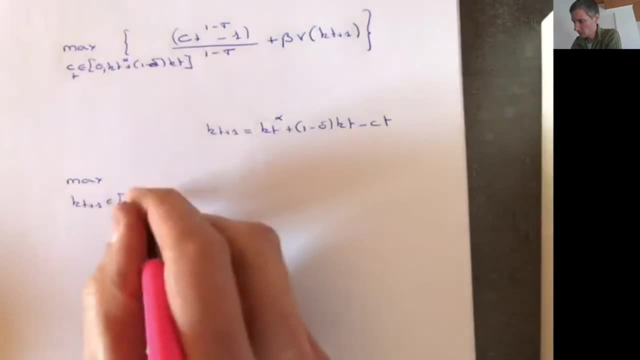 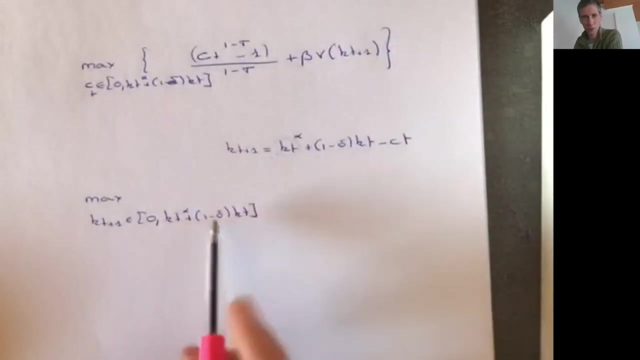 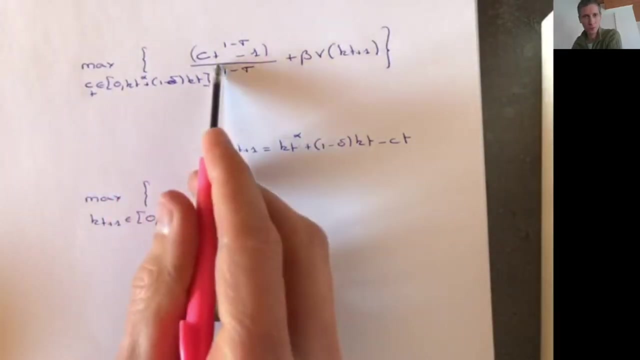 to get rid of the ct variable here, right, so i'm going to maximize kt plus one which is in zero kt, alpha plus one minus delta kt. right, so this is going to be my g of kt. okay, of the instantaneous utility function. so if i substitute ct, plug it in here, then i get. 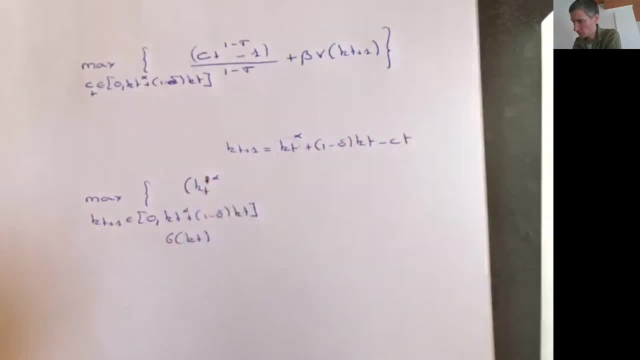 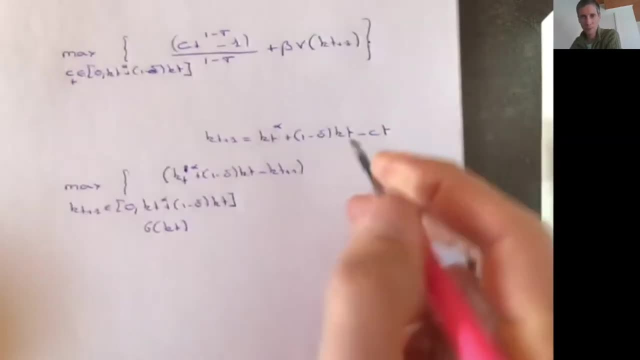 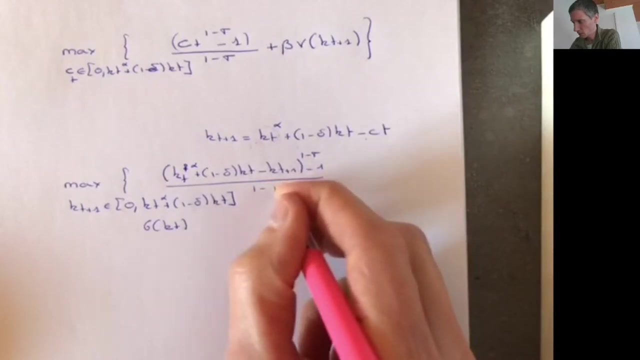 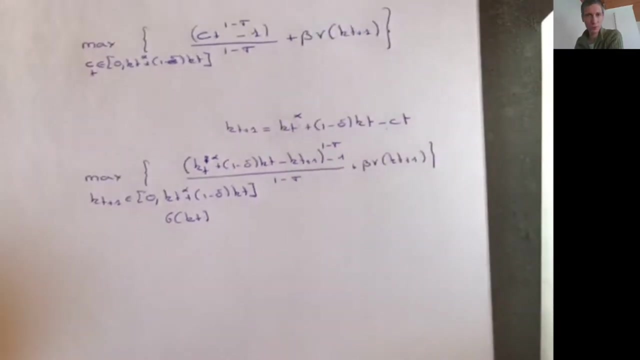 kt to the power alpha- there's a t at the bottom- plus one minus delta, kt minus kt plus one. and then to the power: one minus sigma, minus one divided by one minus sigma, and then plus beta, v, kt plus one. okay, so this is my bellman equation and this is going to be. give me tv. 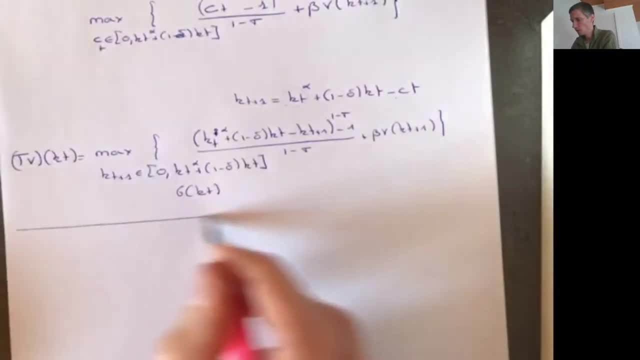 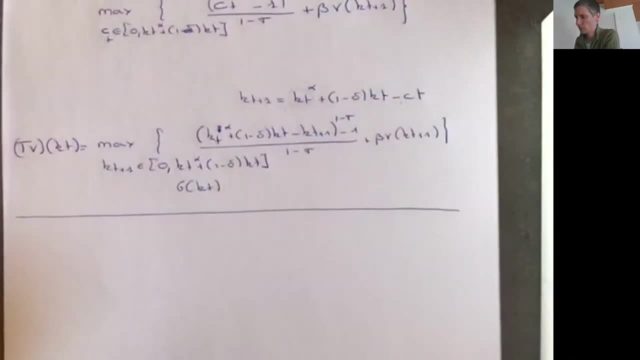 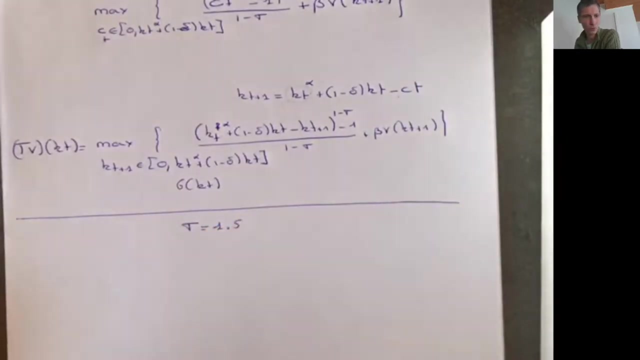 of kt. okay, so this is a particular instance of a growth model, so i need some parameter values, so let me check which ones. i'm going to use it yourself at home, so i'm going to use sigma equal to 1.5. i'm going to use beta to be equal to. 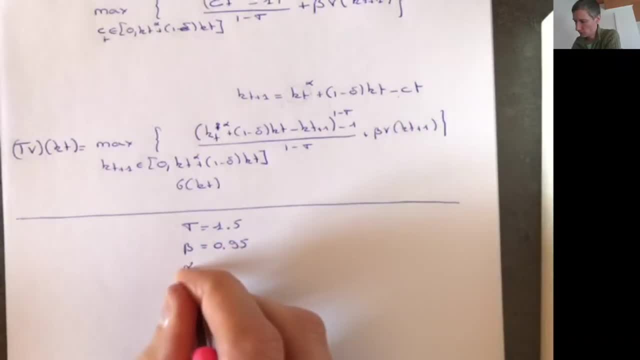 0.95, i'm going to use alpha equal to 0.3 and i'm going to use delta to be equal to 0.1, which is the depreciation rate of capital. okay, okay. so in order to get this model running, what i need to do is i need to write some functions. 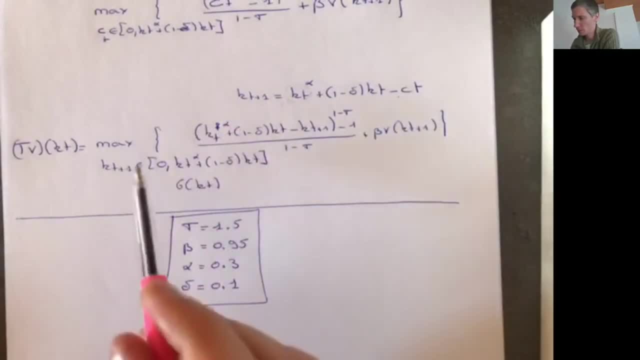 first to compute this one here. next, i give the function to compute the maximum for a given kt. i need to compute the optimal kt plus one. i have to do this for every kt, and then i have to iterate again and again. okay, so i'm going to use this in julia, but you can also do this in. 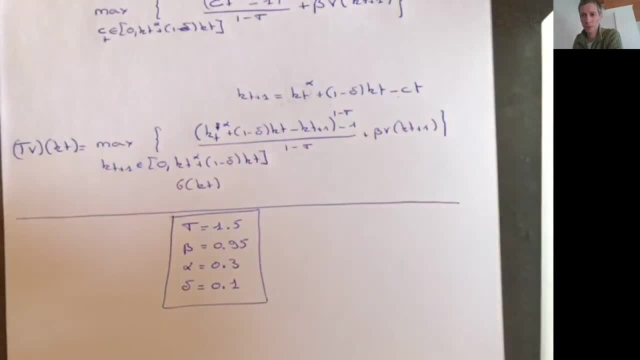 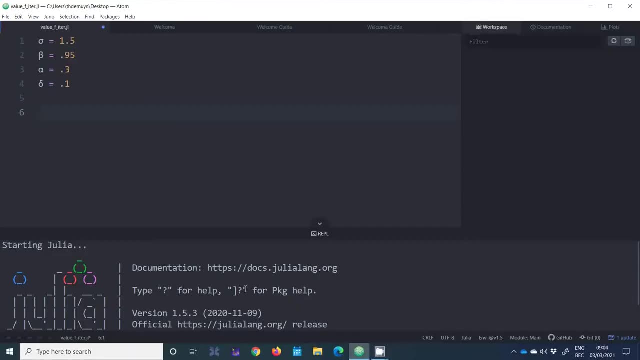 other programming languages. it's very similar. uh, so let's start programming. so this is julia, in particular julia 1.5.3, but all the coding that i'm doing here should also work for earlier versions or later versions. so so far, what i've done is i've just inputted these parameter values for alpha beta. 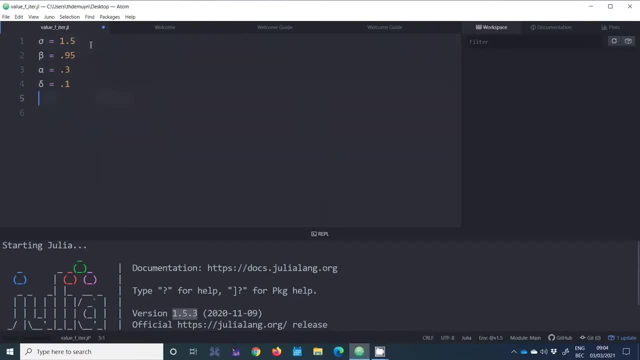 sorry- sigma, beta, alpha and delta. so what do we also need? well, we need a vector to save all the states. so normally i call this a vector x, but for this model let me call it the vector k of capital stocks. so i'm going to use a vector of equally spaced values. so for this we can use the command. 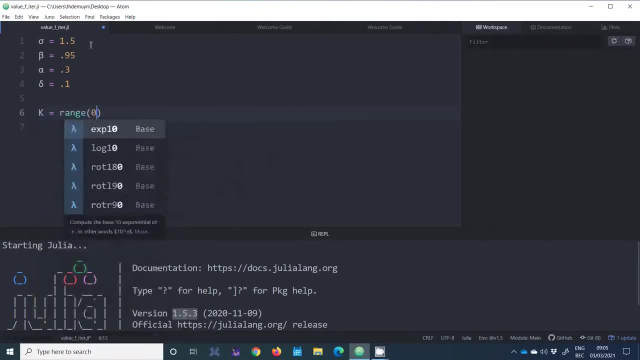 range. so i need the starting value- let's put it equal to zero- and value- put it equal to five and then a length of the vector. so i need to put it equal to zero and then a length of the vector. so let's take 100 for now, so we can increase this value later on. so i'm going to change this to. 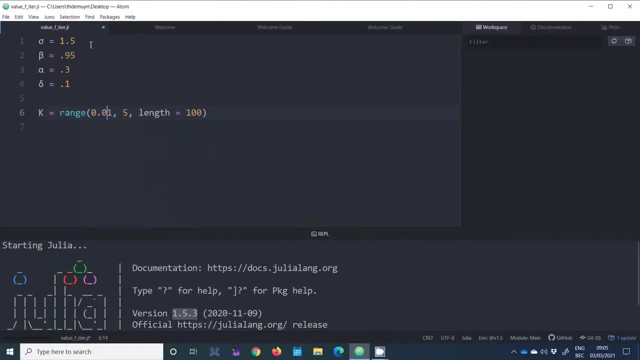 a low value, which is strictly positive, because if i start with a capital stock of zero, then next period i will again have a capital stock of zero and from then onwards, every time i will have a capital stock of zero, right? so this is not a very interesting value, so i'll start at 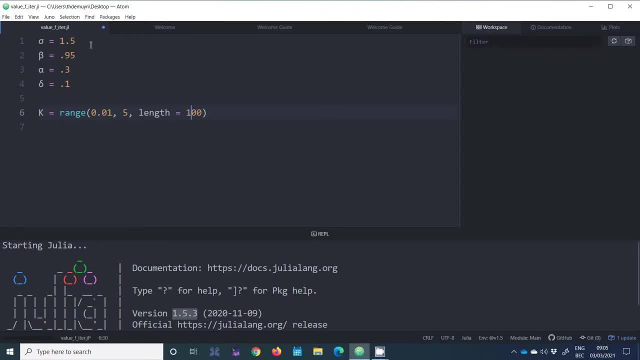 least some strictly positive value for the capital stock, okay. so let me first read in all these values. so here i have just a vector of length 100 with equally spaced values. okay, so now let's start the real coding. so first i need a function- let me call this objective value, okay- which is going to give for a given 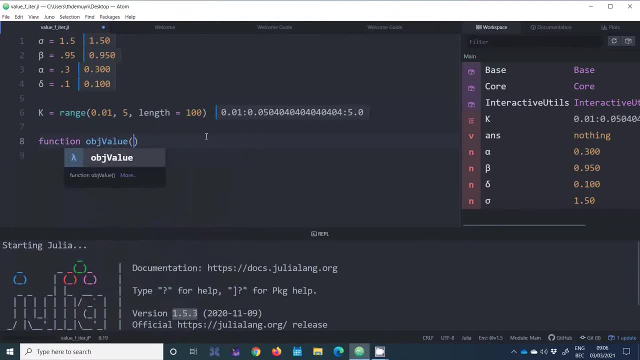 state and action, the value of the objective function. so what i need? i need an index for the capital stock today, so let me call this k index. i need a index for the action to take, which is the capital stock next period. so this is capital stock in the next period and the index of 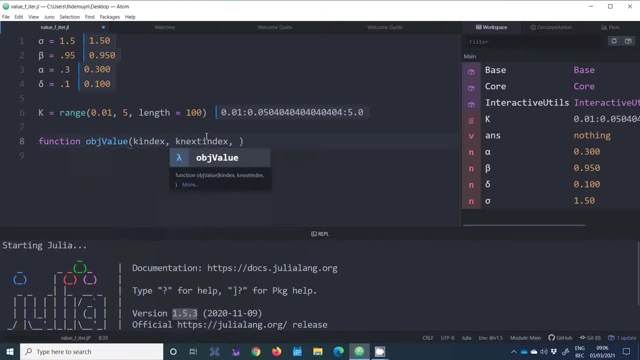 this capital stock, then i need to to enter the vector of k and i need a vector for the value function. okay, let me end it here. so my capital stock today is going to be the value of k at k index, my capital stock in the next period. so let me call this k. next it's going to be k at k. 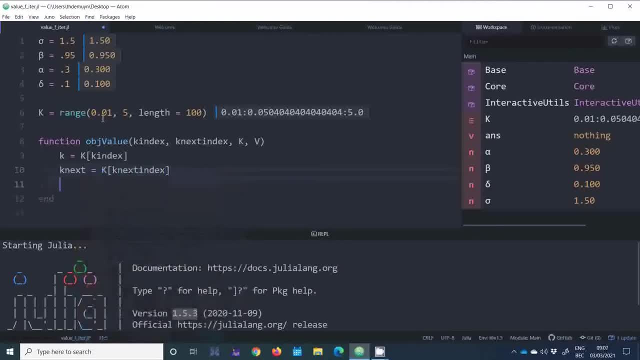 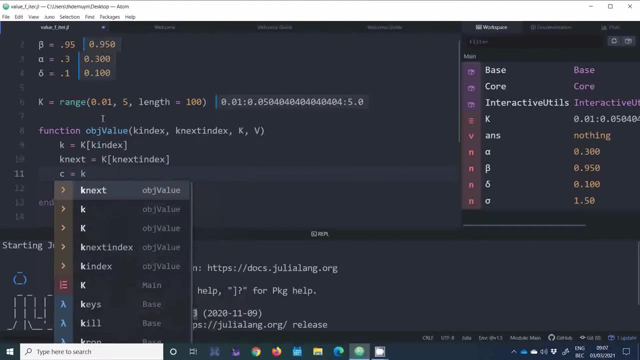 next index. okay, and from these two things i can already compute the amount of consumption. okay, so c is going to be the total amount of output that i have available, or capital that i have available, which is k to the power alpha plus one, minus delta times k, and then minus what i consume in the next, the capital stock of the next period. so this is k. 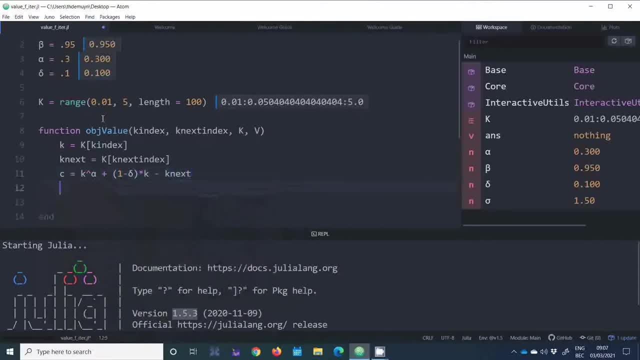 next: okay, so this is my consumption amount. so if c is strictly below zero, then i know that my optimization problem is not feasible. okay, so if c is strictly below zero, then i'm going to output the value of k and i'm going to return a value of that number. that's very negative. so here i can. 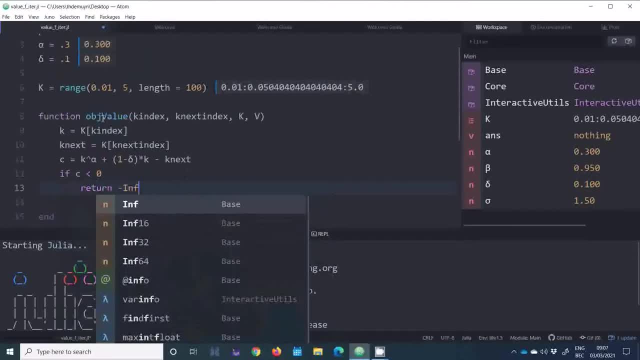 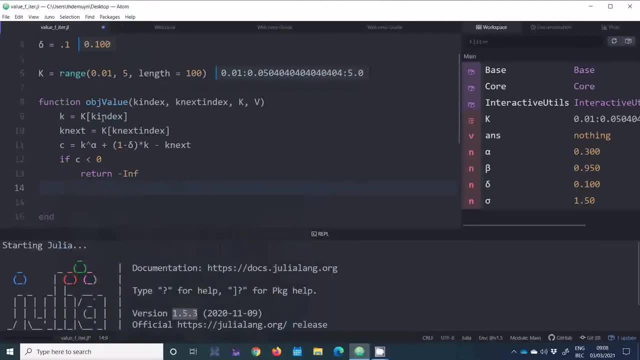 use the minus command. so it's going to be a very, very big number. so it's a part of the software, probably the biggest number that computer can generate to some degree. okay, so if c is smaller than zero then i'm going to return very negative value, else i'm gonna have to return the objective. 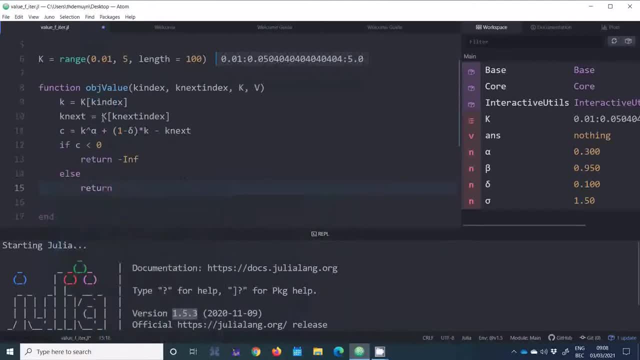 function. so so the utility which you see to the power, one minus sigma, minus one, divided by one minus sigma, okay, and then plus beta times v, at well, the capital stock in x period. so this is k, next index, okay, and this is going to end it here. okay, so let's compile this, and it's always good if you. 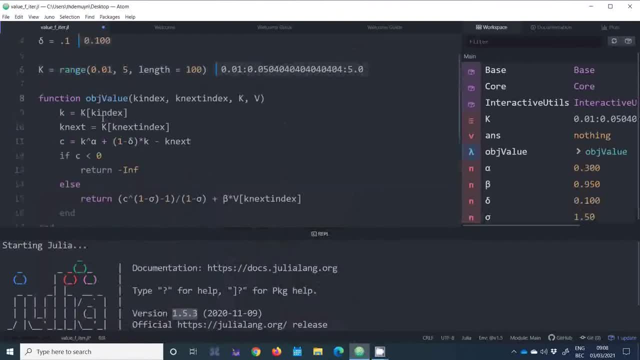 write a function to at least try to run the function. so if you're going to run the function, just leave it at any time. you need some v, and of course we're not characters, but comfort. okay, so you see that it gives some output. so for this we need a vector v, of course. 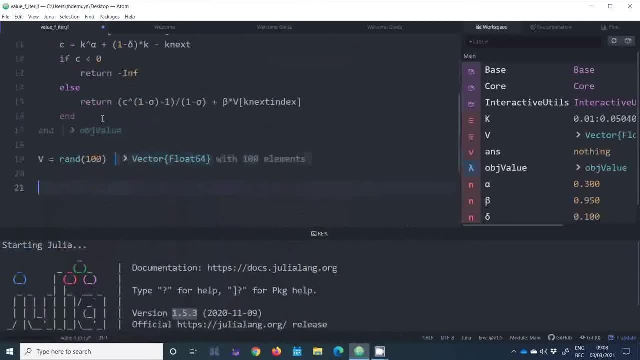 so let me take now for the moment some random vector of size 100, okay, and then let's try to run this. so i need the k index. let me pick this, for example: 30, the index angles period. we pick this to be 20.. then i have to give it. 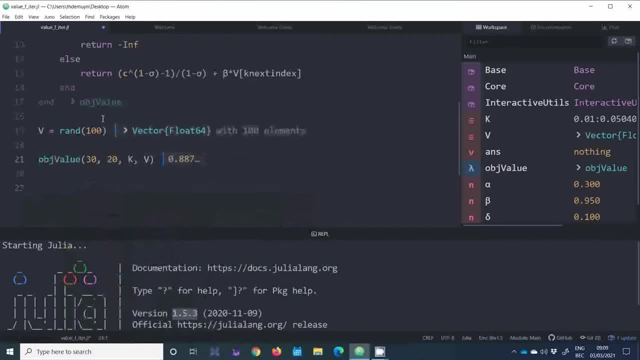 uh, the vector k and vector v, and it should give me a number, okay, which is here 0.8875. um, let me try to generate a capital stock that's very much bigger. well then, it's here, this amount of capital. the next period is not feasible because it returns a value of minus infinity. so this: 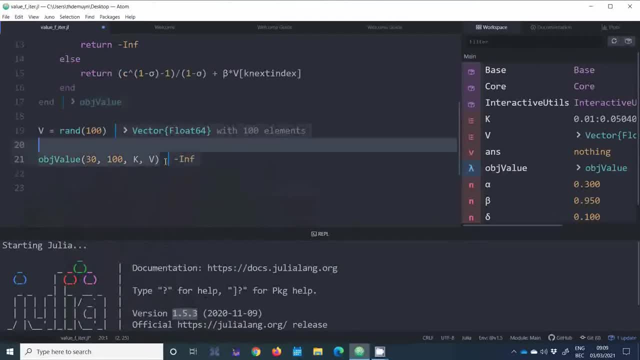 seems to work just fine. all right, so next i also need a function that computes the maximum for a given k index over all the possible value of k next index. okay, so let me name this compute max. so as input it has a k index, it has a vector k and it has a vector v. okay, so here i'm programming. 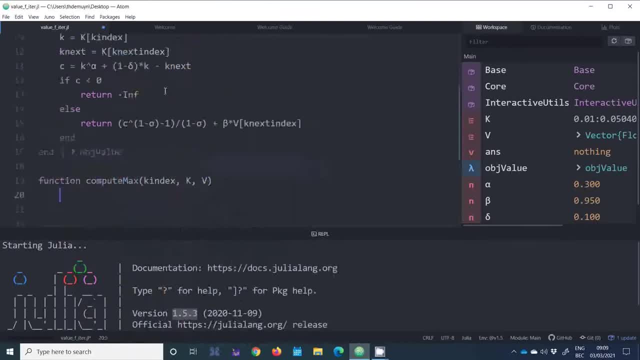 very rudimentary. just on this program run. of course you can add the symbols and probably do stuff much more quicker than i'm doing here or much more efficient. okay, so the aim here is just to have a program that's that's running and giving me the output that i 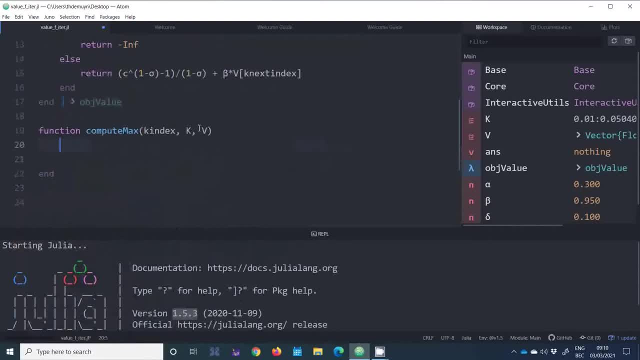 want, um, so what i need to do is i need, uh, an output of this function is going to give me a value of the objective function, so let me call this solution, let me put it at some very low for a moment, and then i need a number, the, that's going to give the index at which i have the 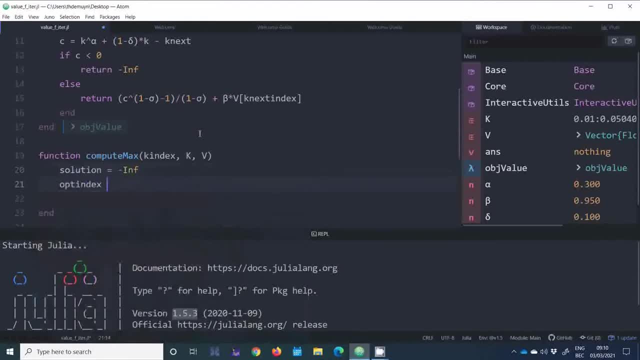 so let me put it at some integer value which makes sense at the moment. okay, and then i have to loop over all possible values of next period capital stock. so there are n of them and i can put. so i can say: for i equal to 1 until 100. but now i 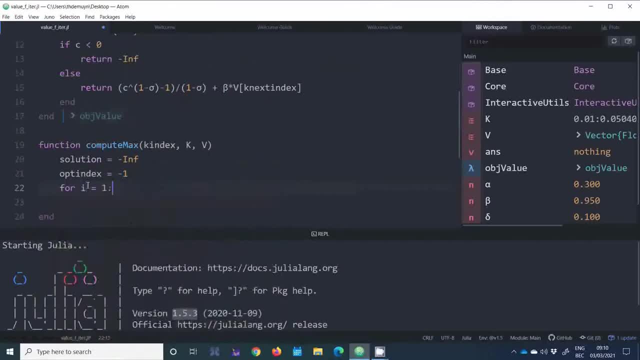 have the problem that if i change, for example, here the length of my k vector, i have to also change this number right so i can can get it actually from this vector here, which will be of length n. so I just put here n equal to the length of k, and then I can run from 1 to n. 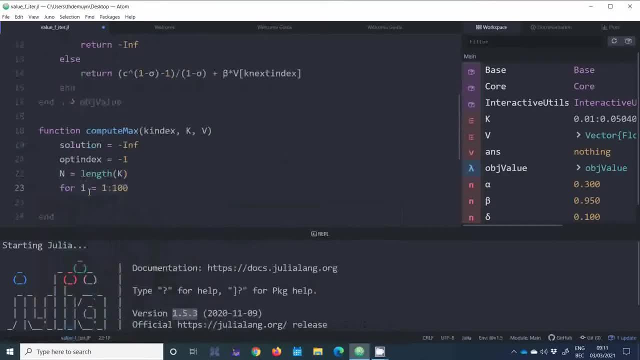 Then if I change the length of this vector at some point here, this will change automatically. So let me compute a value which is going to be objective value for k index. k index period is going to be i. I'm going to have to give it a vector k and a vector v. 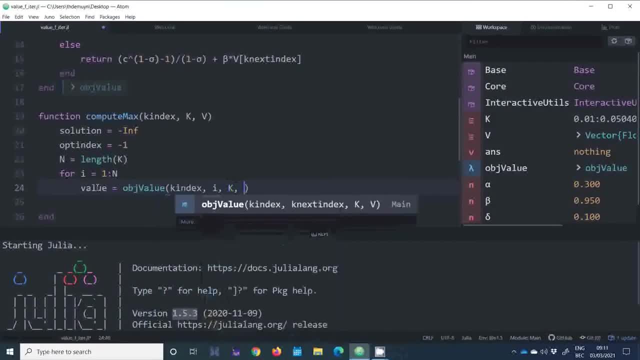 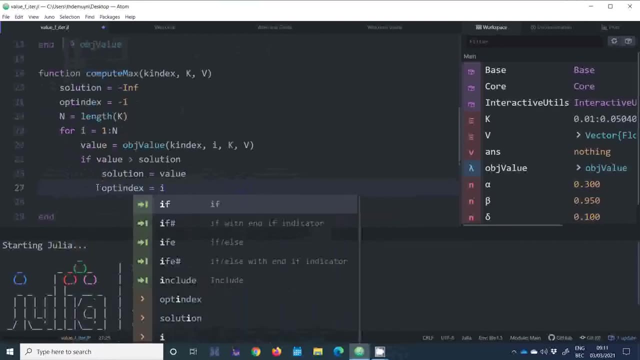 So if I find a value that's bigger than solution, I'm going to update the solution. I'm going to update the opt index. It's going to be equal to i in this case. I'm going to end these loops and then I'm going to return solution opt index. 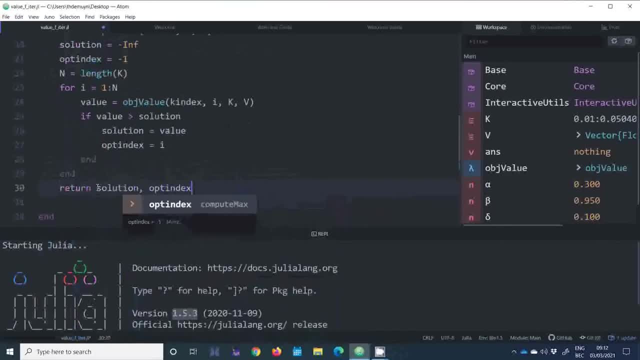 Okay, so let me see if this works. So compute max. If I give it, for example, at capital stock, 50, right, and then I have to give it a vector k and a vector v, it should give me a number for the value, okay. and then the index number at which the optimum is reached. 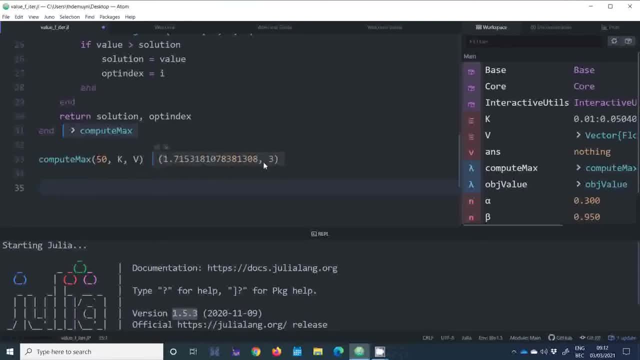 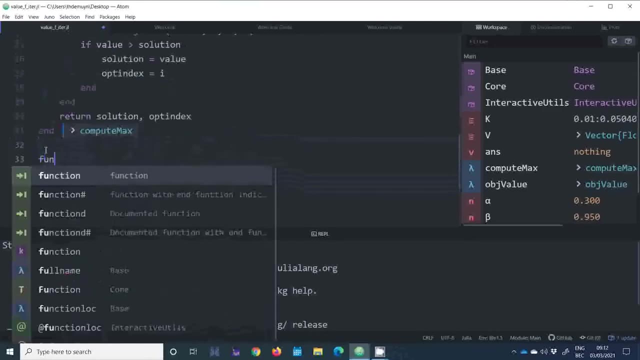 which is here a tree. Okay, so this looks good for the moment. Then I need a function to compute a new value function. Okay, so the new value function is going to take us inputs k and v, So what I need to do is I have to loop this over: all values of k index. 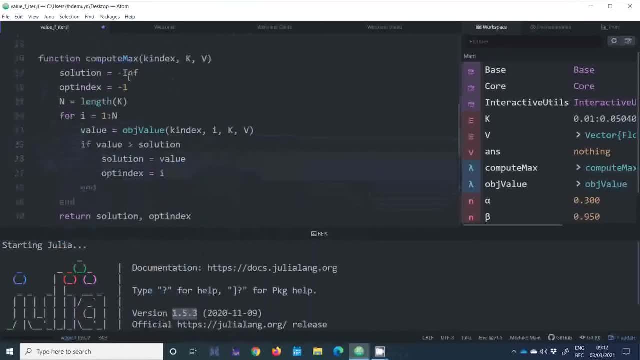 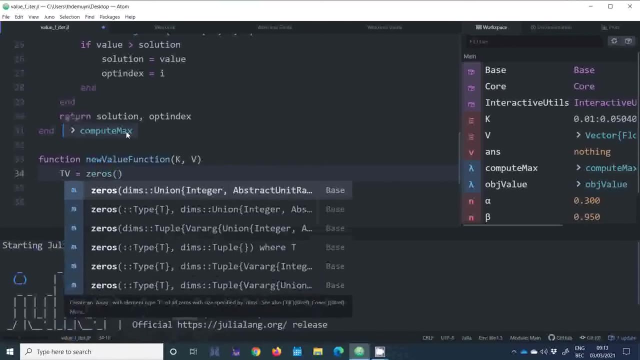 Okay, I'm going to store this in a new vector which is going to be tv. It's going to be a vector. Let me Initialize it as a vector of zeros of size n, And here again, n is going to be the length of this vector, k. 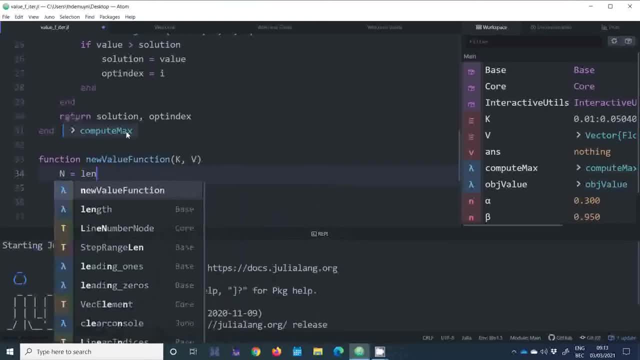 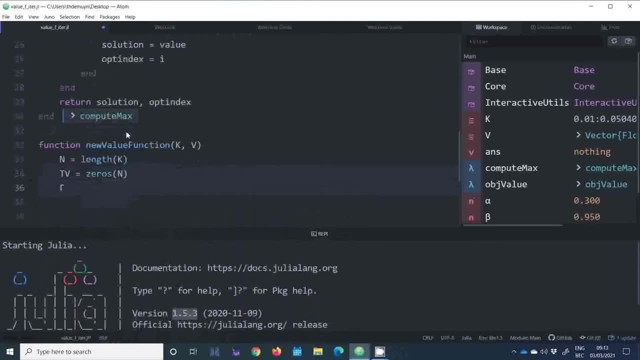 And I'm also going to store the solution, which I'm going to store in the vector gamma. It's going to be a vector of zeros and now it's gamma is only going to contain integers, right? So I'm going to specify that this is a vector of integers. 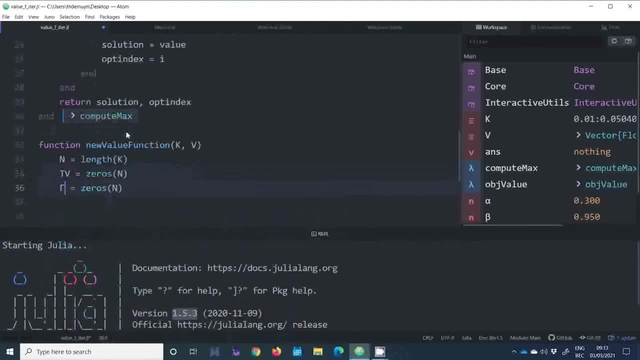 Otherwise my computer will give me an error I know in advance. Okay, so now I'm going to loop for i equal to 1 until n. I'm going to compute tv i and gamma i. It's going to be equal to compute max of k index at i and then k and then v. 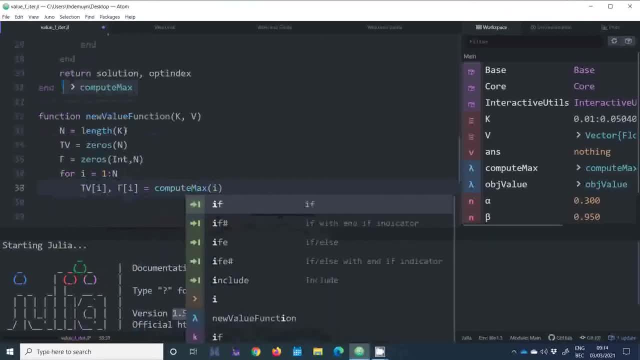 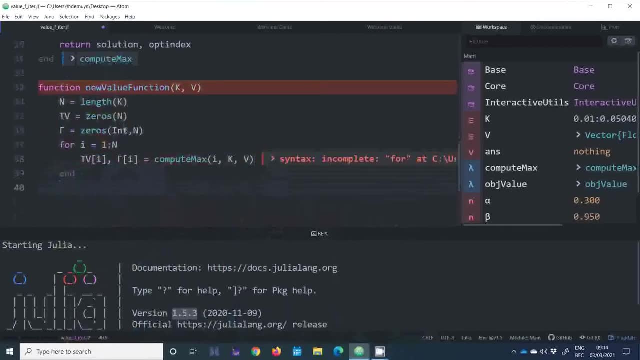 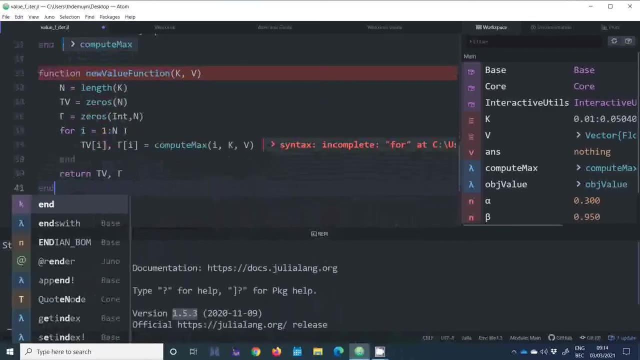 No, not compiling. I'm going to end this. Yeah, I know there's an error. I'm going to return tv and I'm going to return gamma. All right, I'm going to end it. and now it should compile. So if I compute new value, function of k and v. 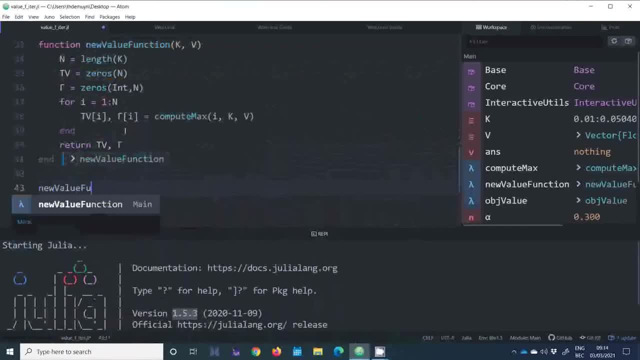 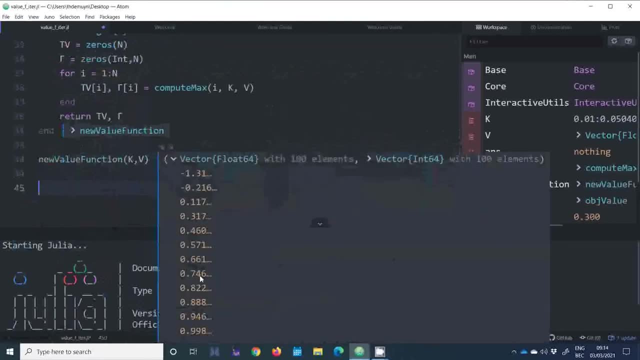 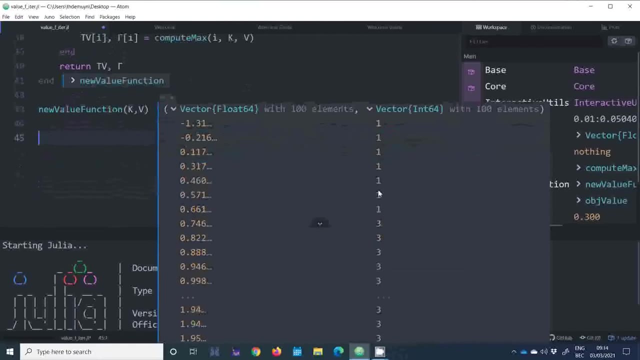 Now, this gives me a vector of all the new value function- right, Which is this one? And then a vector that says at which index I'm reaching the maximum value. Okay, So to finish up, I need one more function, And this function is going to iterate this function over and over again. 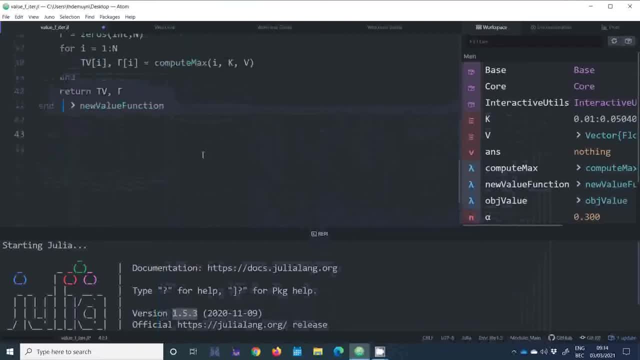 Okay So, function- let me call this value function iteration, And it's going simply to take a capital, the vector of capital stocks. Okay So I need a vector, first into the dimension, Which is simply this, Then I need a vector. 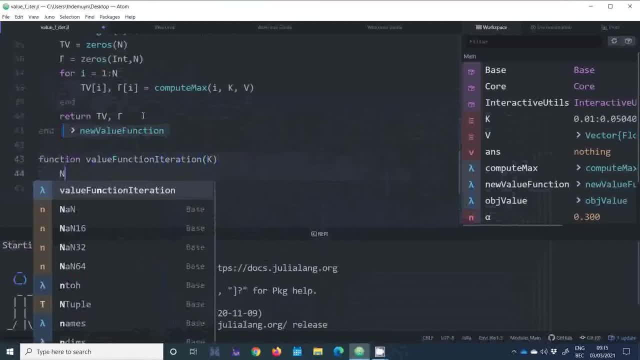 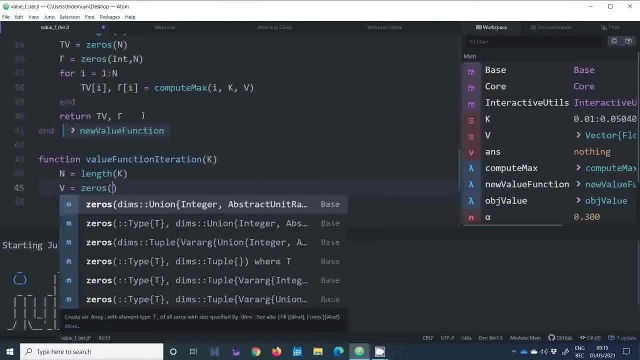 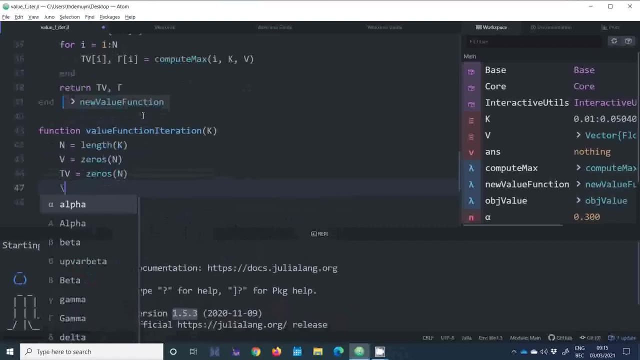 Let me just start with the vector of zeros of size n. I need another vector for the next iteration And I need a vector of solutions. This is going to be zeros of integer values of size n, Okay, And then I need each time, at each iteration: 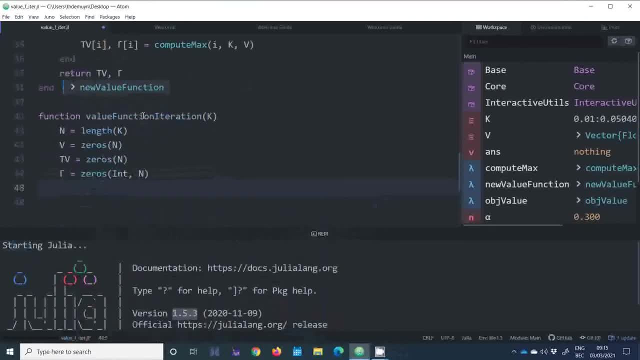 I'm going to compare to the distance between this v and this tv Right, And if this distance is below some threshold, then I'm going to stop the iteration. Okay, So I will need to have some variable that captures the distance And let me put it at some arbitrary big number now. 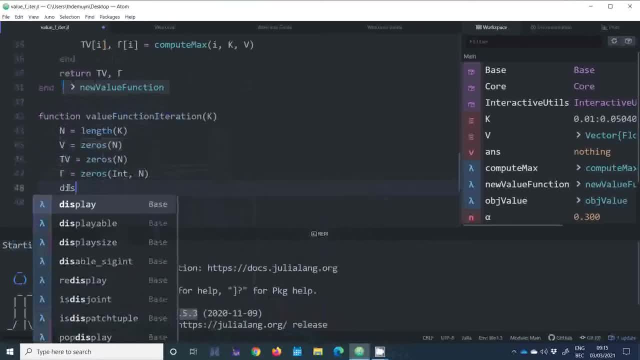 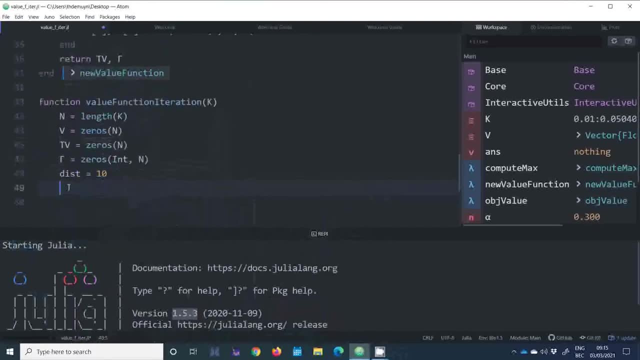 Let's say 10. And I need a cutoff for when this distance is below some threshold. So let me call this epsilon. I'm going to put it at some small number like 1 to the minus 6.. Okay, So that's normally 6 zeros with a 1.. 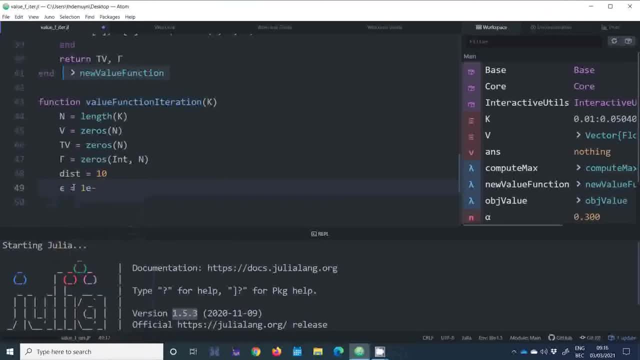 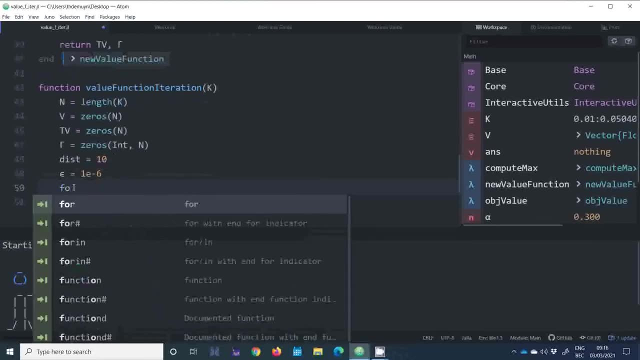 And then I'm going to have- I'm going to have a while loop, Okay, So, while the distance is still bigger than epsilon, I'm going to iterate this Right, So I'm going to compute tv and gamma is going to be equal to new value function at k and v. 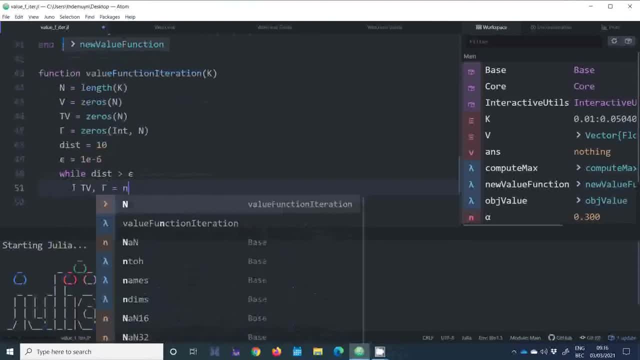 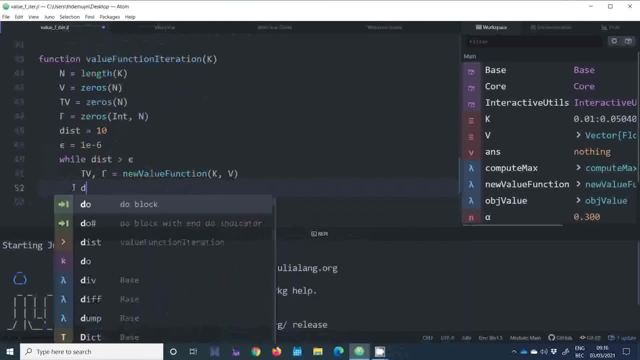 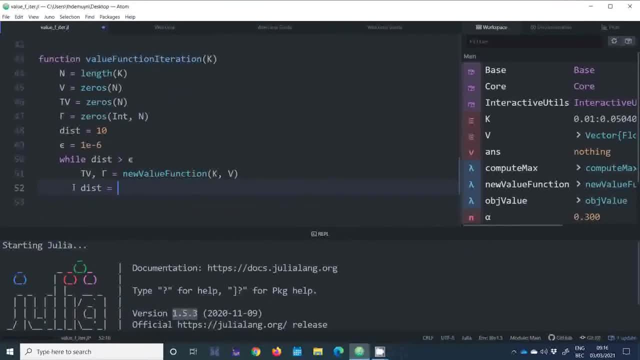 Okay, Okay, Okay Okay. Here v and tv are vectors and the absolute. So in Julia, if you want to use a function that you want to apply to a multidimensional vector, normally you put a point after the function, Right? 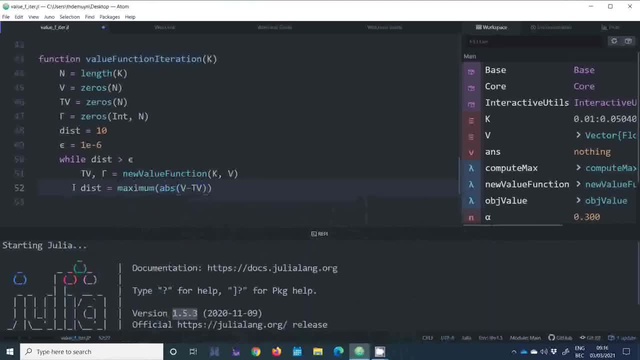 So there's that use the absolute value function that apply to the input, which is going to be a vector. Okay, So this should give me the distance, or the maximum distance between v and tv. Okay, So once I have this, it's going to check out the distance. 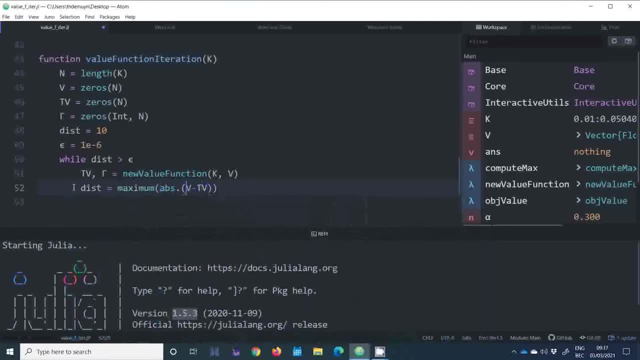 It's going to check if the distance is bigger than epsilon and then it's going to iterate. But now I have to use the output tv of the previous period and in return for the function v instead of the function v here. All right, So I have to switch v with tv here and here. 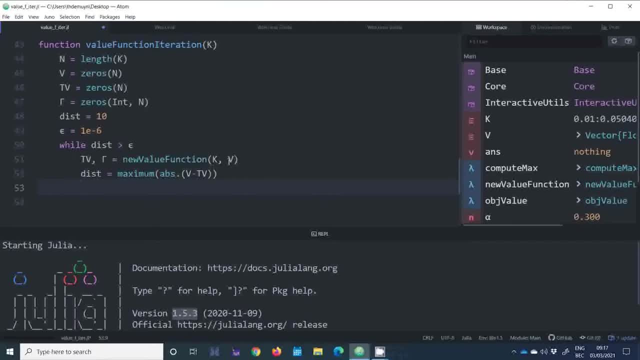 this is something particular about Julia and also Python. If you write an assignment like this, Julia is not going to copy the contents of tv and put it into v. No, it's going to assign the name v also to the vector tv. Okay, 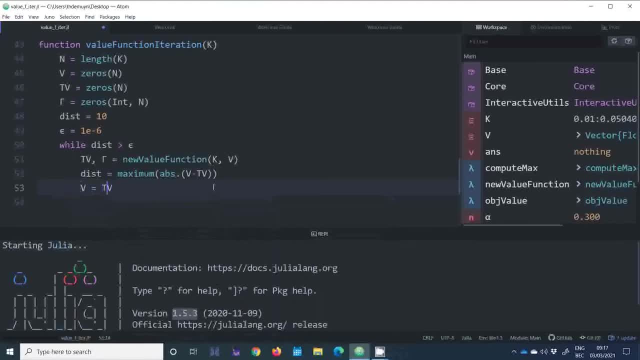 So when, in the next iteration, you're going to change tv, then actually you're also going to change v at the same time, And this is something that we don't want Right? Actually, we want to copy all the values of tv into v. 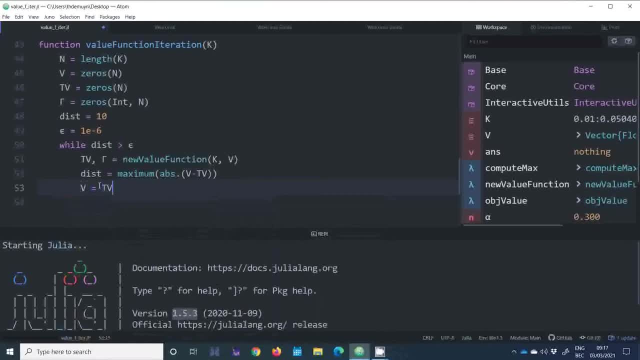 So you have to put the command copy here Right? So copy here says that: take all the values of tv, put it in the vector v, which is going to be then inputted in the next iteration here to compute a new value of tv. 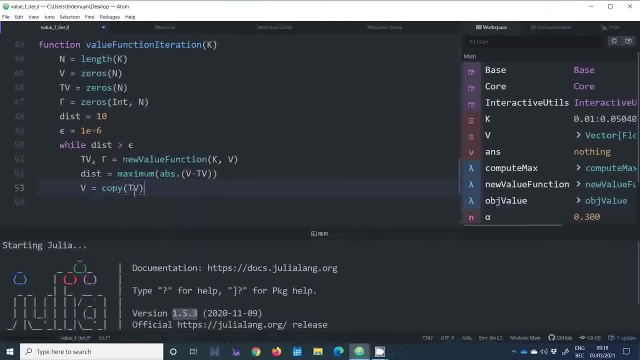 Okay, So we're going to end this and then maybe end this, And then we're going to return. once the distance is smaller than epsilon, it's going to skip this loop and we're going to return tv and comma. Okay, Or we can actually also return v. 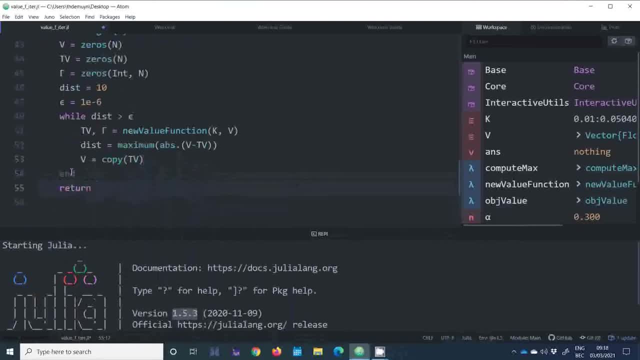 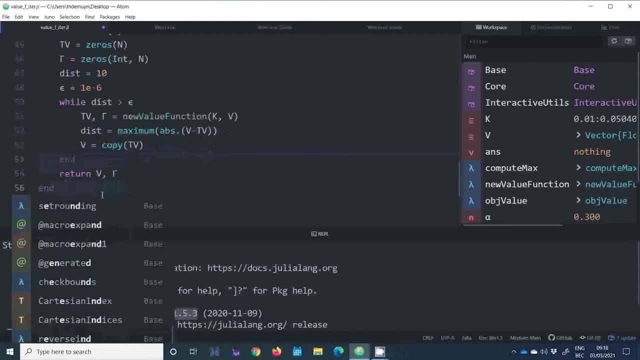 right, Because v is going to be equal to tv. So here we're going to end, And maybe it's easy also to provide some output to this algorithm. So let's, let's first count the number of loops. So here we set it at zero. 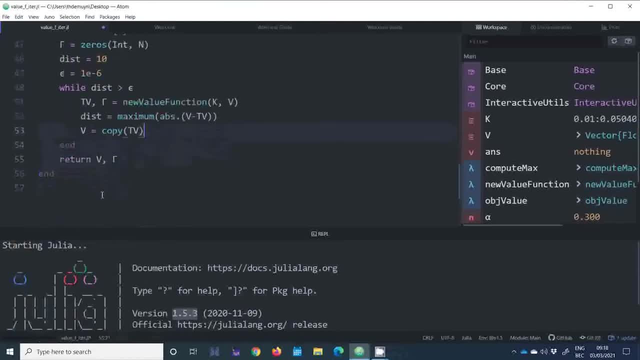 And then at every iteration we can add one to the number of loops. So you can do this. plus equal actually says that take the variable loops and add one to it. Okay, So, so, so, so, let's put loop number loops, and then with the distance, 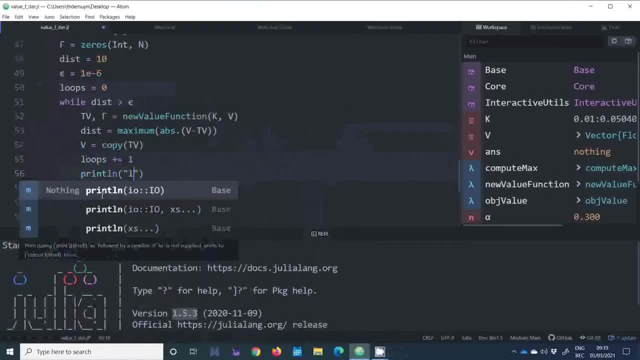 So you also have an idea of the distance, how far we are from obtaining the threshold epsilon here. Okay, So this should output where we are at the algorithm. Okay So let's compile it and let's now try this. So I'm going to store this at my optimal value function. 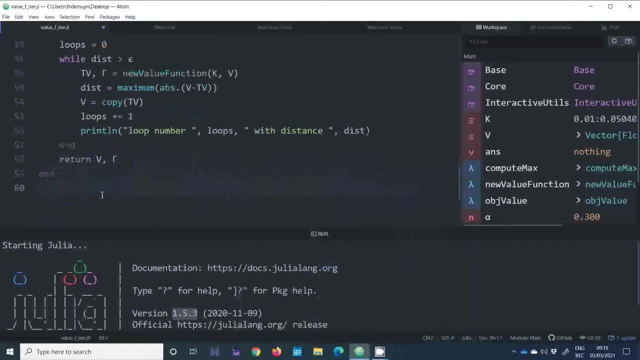 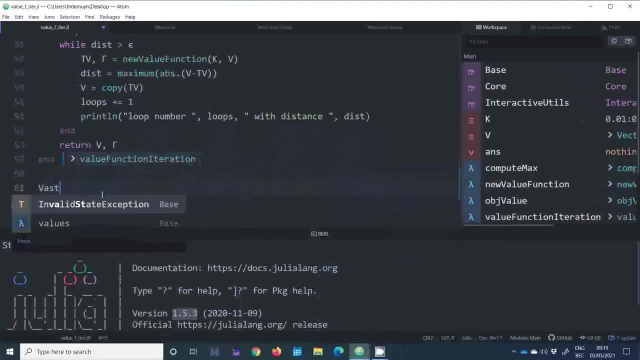 And then. so I'm going to store this at my optimal policy function value, function iteration, And I only should enter the capital K. So, fingers crossed, Let's see what happens. Okay, So you see, here at the bottom I'm looping 200 times. 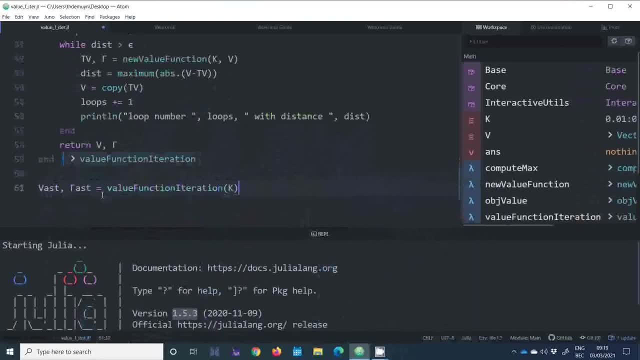 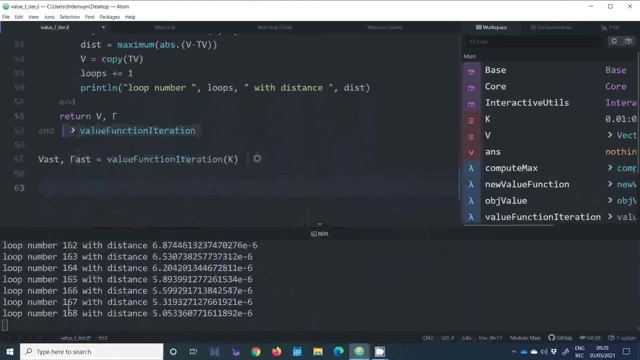 right. So after 200 times the distance has reached something that's smaller than my epsilon, And you see indeed that. so, number one, let's start with the distance of 1.3, and that every iteration it goes down. All right, 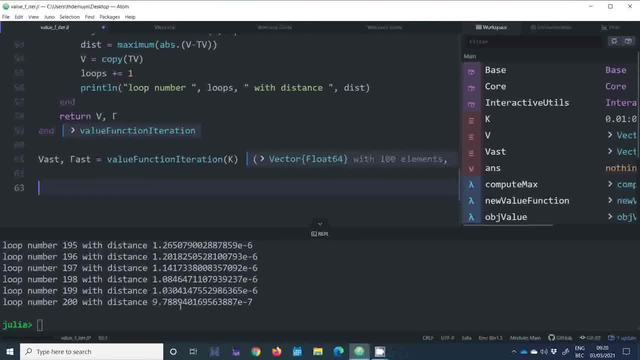 So this is this contraction mapping property: that the distance between iterative value functions actually gets smaller and smaller and smaller until you converge to below your thresholds. Okay, So what we can do is we can. so this shows that it converged. So let's not plot to the small pieces. 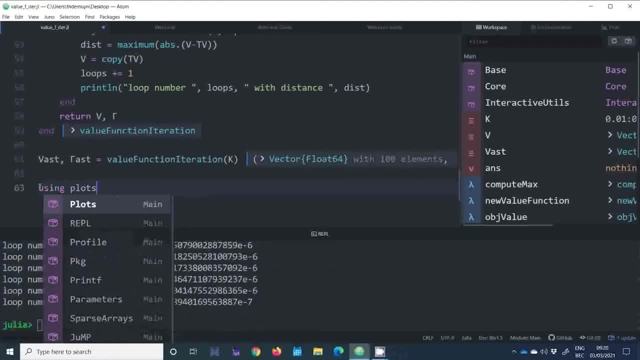 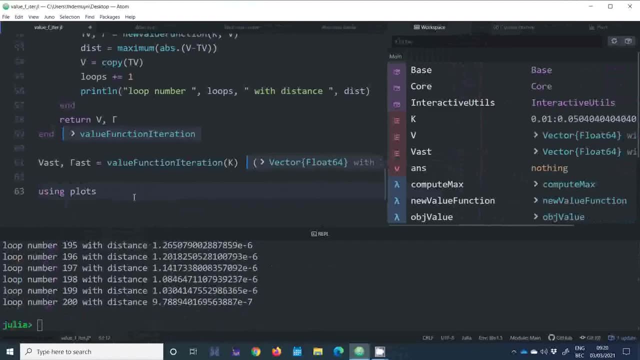 So let's make some graphs here, right? So this is a big package, So it takes some time to to to load into memory. But what we can do is we can plot K on the X axis against the optimal value function. 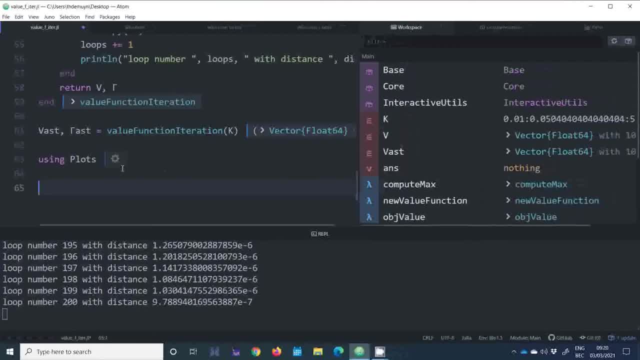 P S on the Y axis. Okay, Then we can maybe also plot K against the K Next period, right? So if K is so, let me try to plot it here, So it should appear here, next to it, The Pane plots. 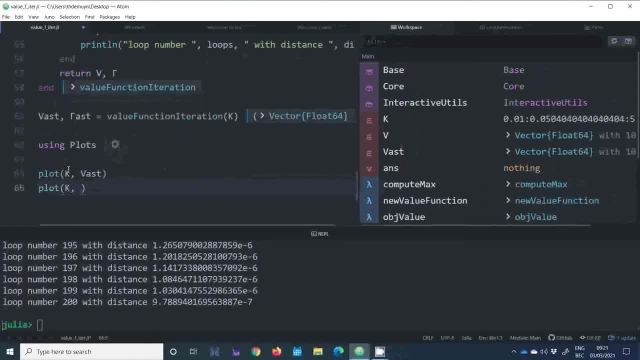 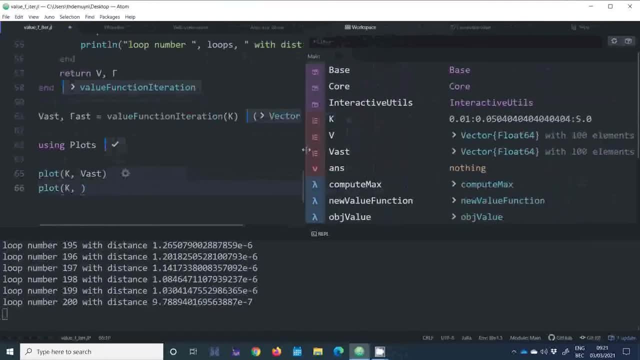 So let's wait a minute. The first plot is always taking a bit more, So what we can also do is you can plot K today against K tomorrow, and K tomorrow is going to be K of gamma. it doesn't want to. it's too busy taking the picture, so let's wait a little bit, okay. 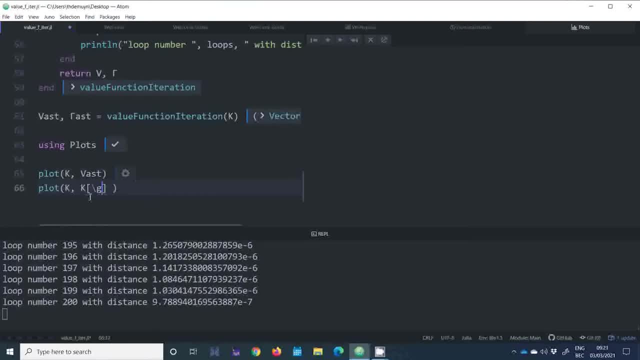 yeah, that's the one. so gamma asked as a vector that points you to the capital stock and the index of the capital stock next period. right, so if i input it into the vector k, this vector will now contain the values of the capital stock in the next periods. okay, so here on the right hand. 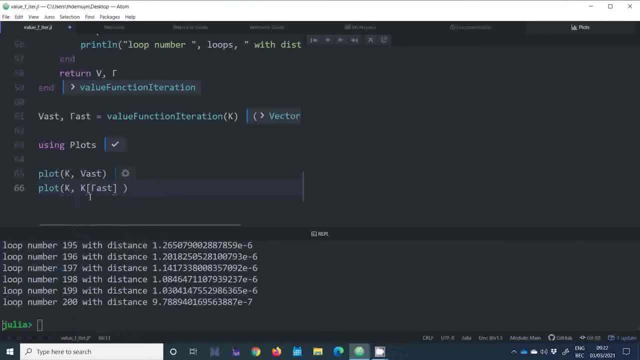 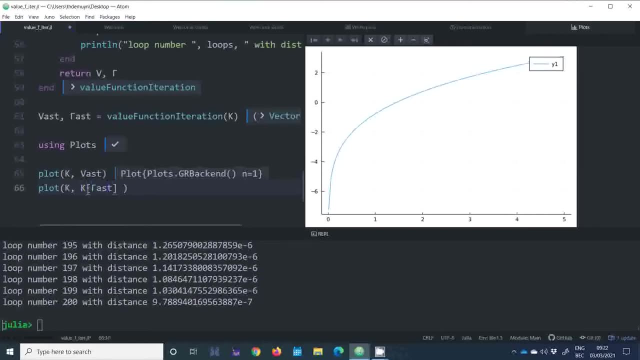 side. we see it has compiled the first one. so you have k on the x-axis and you have the value function on the y-axis. so you see that this gives you a nice concave function and for each capital stock k, it gives you the value v of k right, which is the function, the fixed point that we computed. 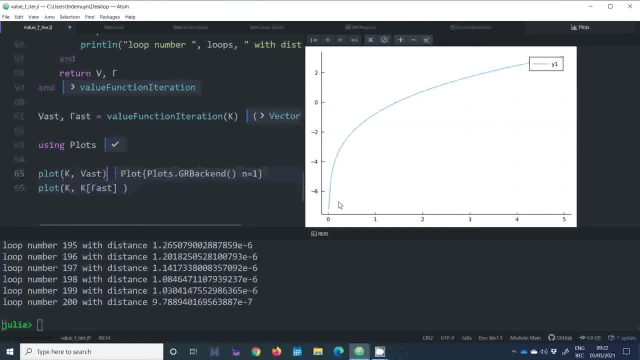 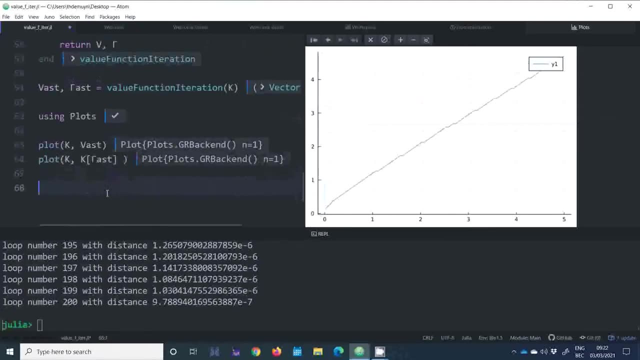 okay, so let's plot the second one. so here we see that this gives you a somehow of a straight line. so it's a bit erect here, because i only used 100 values, so maybe i can increase this to 1000. let's see what it does now. 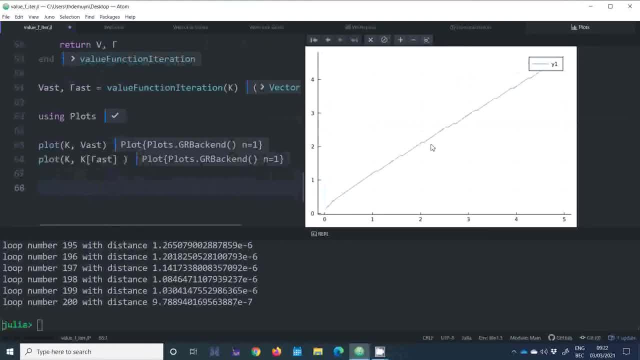 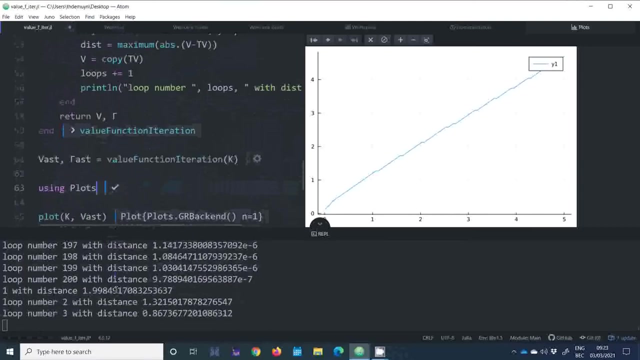 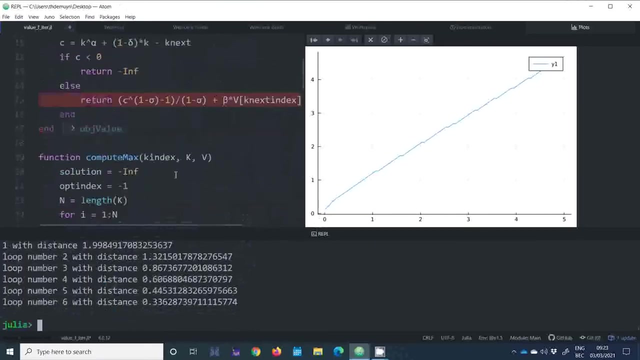 so we can run the same functions. probably will go a little bit slower. oh yeah, it goes much slower, so let's cancel this. i don't have too much time, so maybe i can make this 500, which is already five times bigger than my first one. okay, so you see again that here the distance goes down. 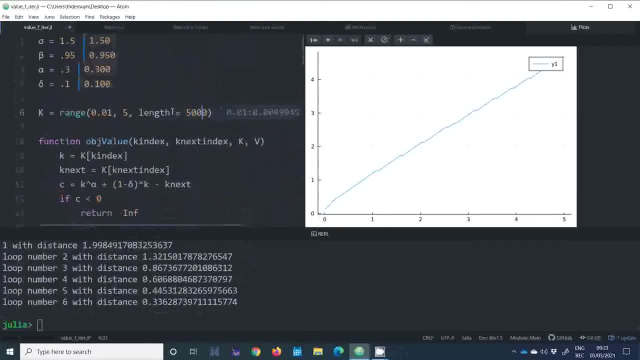 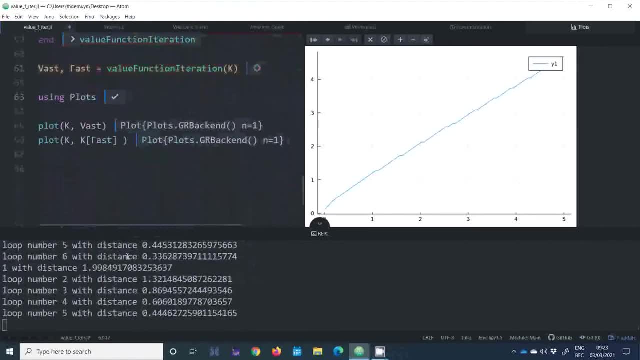 right, and it should reach a value of one to the minus sixth. okay, so i'm at a minus three, i think. of course, the lower you take epsilon, the longer this will take to converge, right. but you see that, as if these numbers go up in your algorithm, then you know you have. 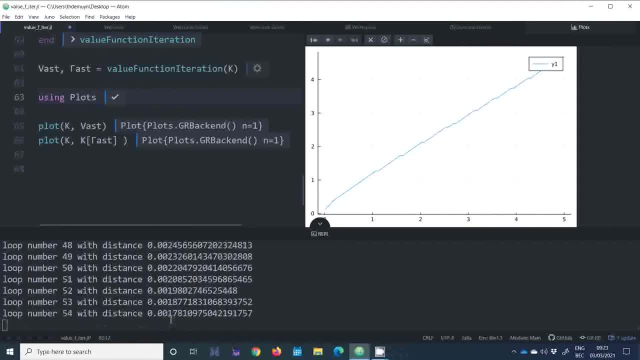 done something wrong in terms of programming, right? you have made an error, so i'm already at four digits, five digits. so if this goes below one, then i'm the algorithm should stop. i think, come on, almost, is this all right? oh, that's right, that's right. 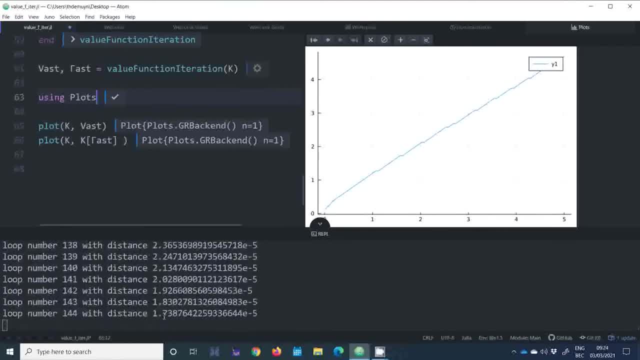 all right, so it's all right, all right, so, so all right, finally. so let's now plot this again, right? so here you have the value function as before, plotting capital against capital stock tomorrow. now you see, you have a smooth line. okay, and let's put it in the same plot, right? so here is the red line. 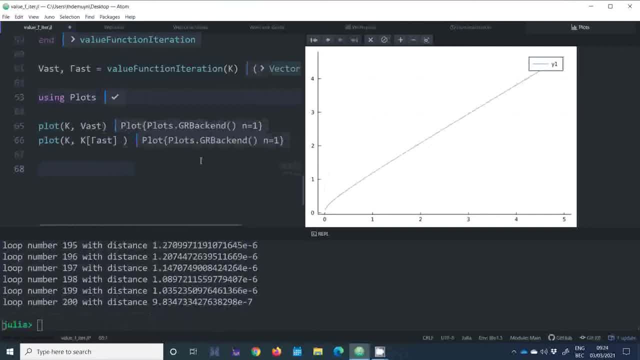 this 45 degree line, and here we have the blue line, which is gives you, for every capital stock, the capital stock tomorrow. and here we see that in the end we're going to converge to this point, to the intersection of the two right, which is going to be the 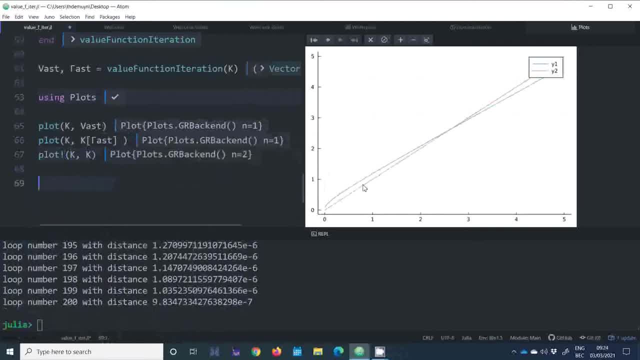 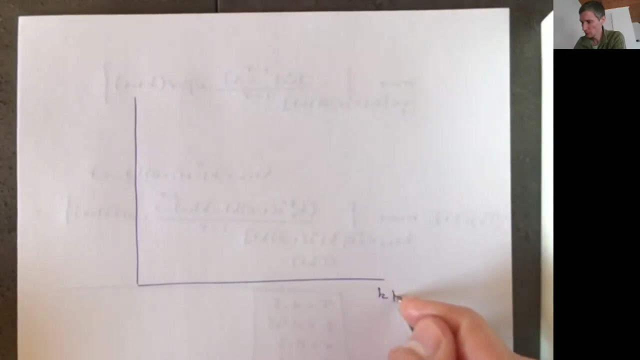 capital stock and limit, okay, so. so basically, this is the capital stock today and this is the capital stock tomorrow, and let me put here the 45 degree line. okay, so here i have a 45 degree line, which means that the capital stock tomorrow i can easily 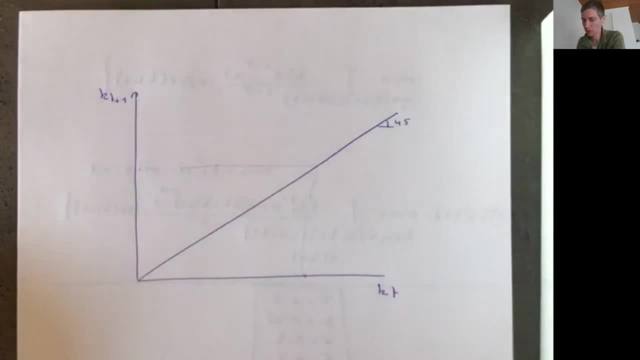 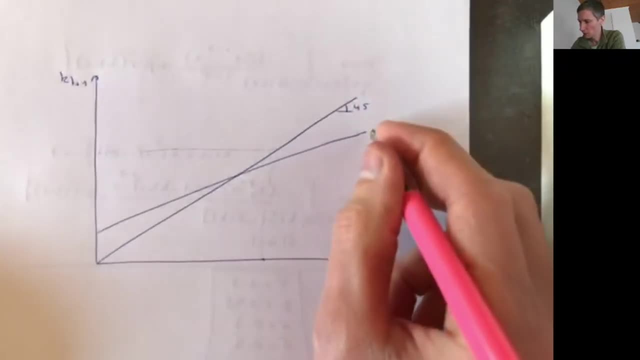 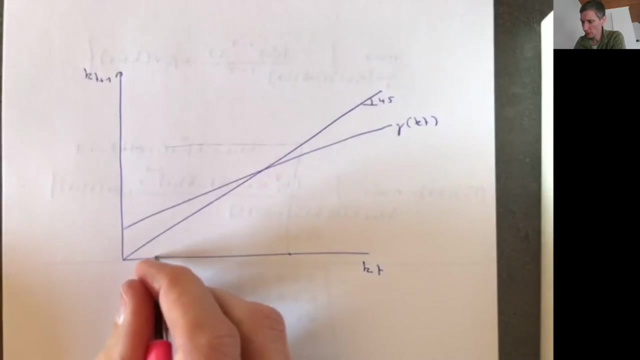 project it into the capital stock today to iterate this process. okay, and then i had a another graph which basically gave me gamma of kt, right, which gives you the capital stock tomorrow in terms of the capital stock today. so let's assume that here i started the capital stock of zero. 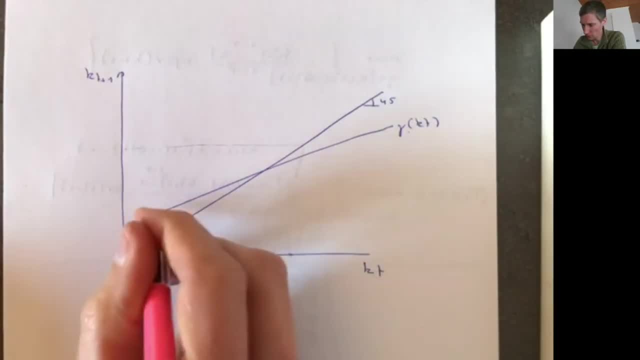 and i have to look at this function in order to obtain the capital stock tomorrow, which is my k1, okay, and then i can use the 45 degree line to project this back to the capital stock today and then can use this one here, this gamma, in order to get the capital stock. 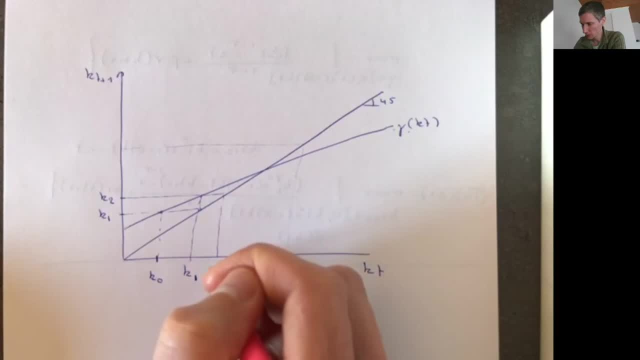 in two days. i can project it back to today using the 45 degree line and so on. okay, this is k3, and so on. right? so basically, what i will have is i have this kind of a zigzag pattern and in the end, this will come closer and closer to this point here. 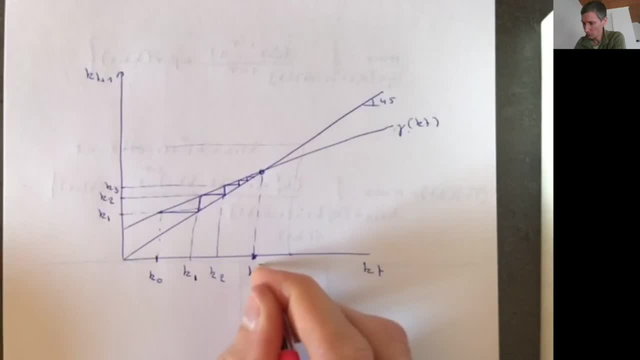 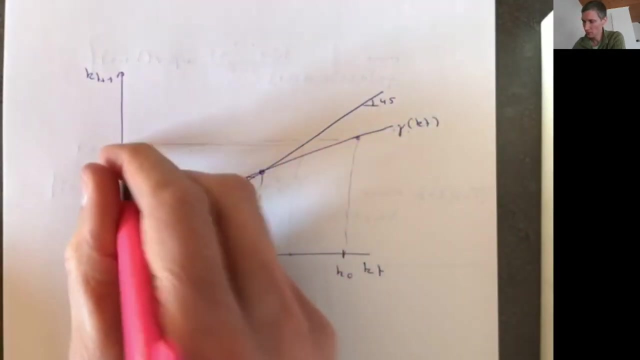 which you can say: this will be my capital stock in the in the long run. right, i will converge to this point. so what happens if i? if i start at the capital stock here today? well, i can do the same exercise. this will be the capital stock tomorrow. then i go with the 45 degree. 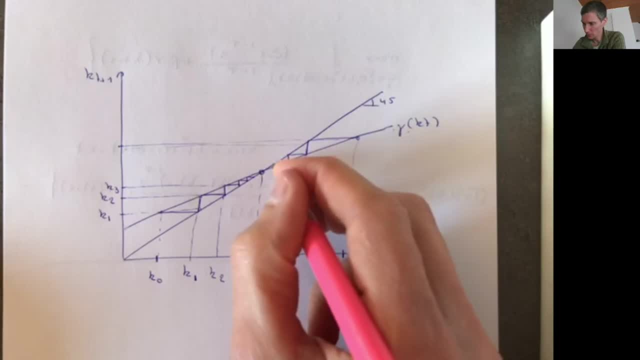 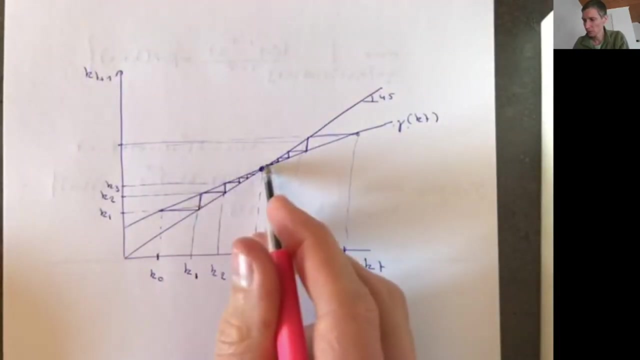 line and so on. so i have here is exact pattern in the reverse direction. okay, so it also goes to this level of capital stock and the elements, right? so using this kind of figure, you can look at the dynamics, uh, of the model and you can see whether it converges to stable equilibrium or not. 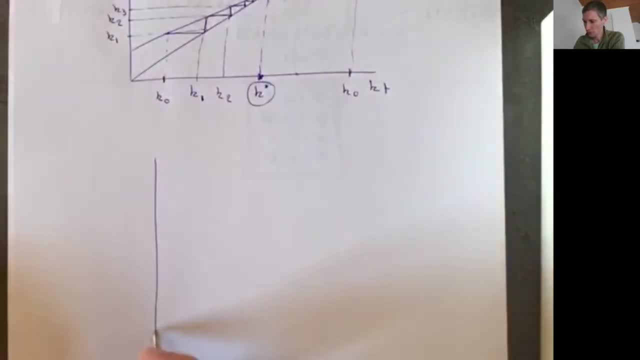 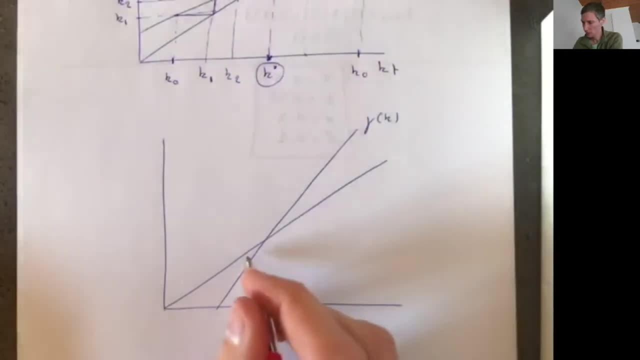 right. so if, for example, if it would have happened that this would have been my gamma k, right then, starting at some point here, i would have decreased my capital stock in the limits. if i started at some point here, i would have moved further and further away from the capital stock. so right so. 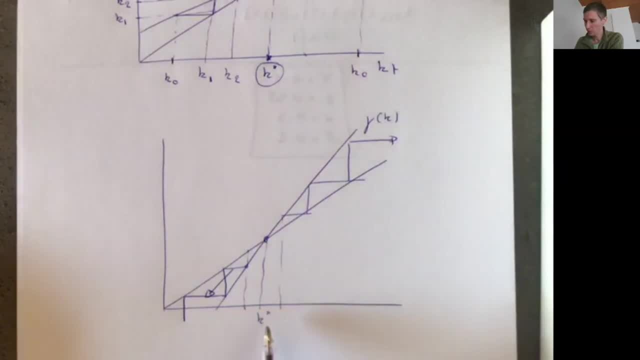 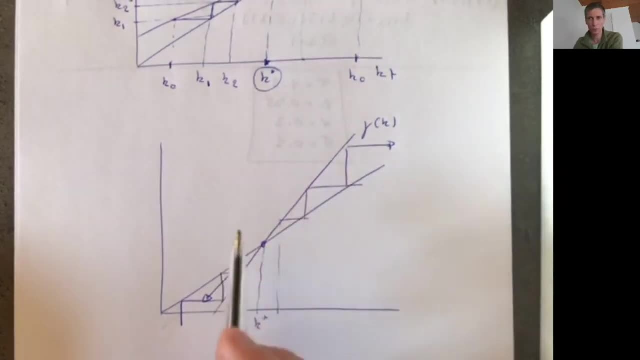 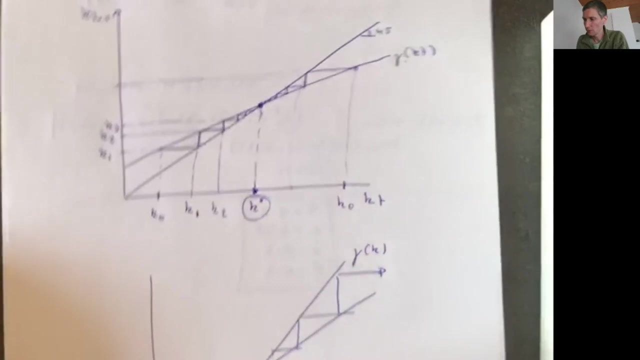 this. this would have been a point of instability, right? so small deviation from this point onwards would either move you down or up, right? so this is what we call an unstable, uh- equilibrium. this is a stable equilibrium, right? so in this kind of model- uh, we have just generated this figure. 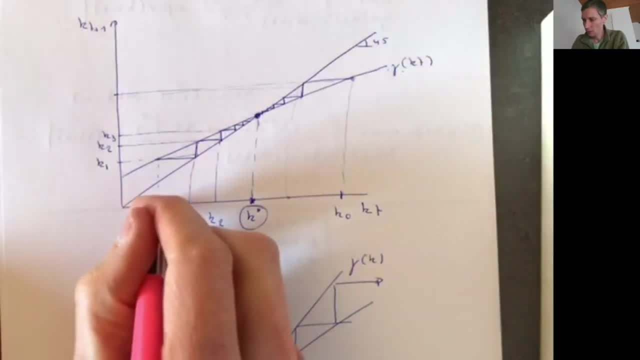 actually we have a stable equilibrium, and then this also shows that we can start from some capital stock and you can actually simulate the path towards equilibrium. okay, i'm not going to to do this, but you have all the results from the program and actually to do this kind of dynamical analysis. 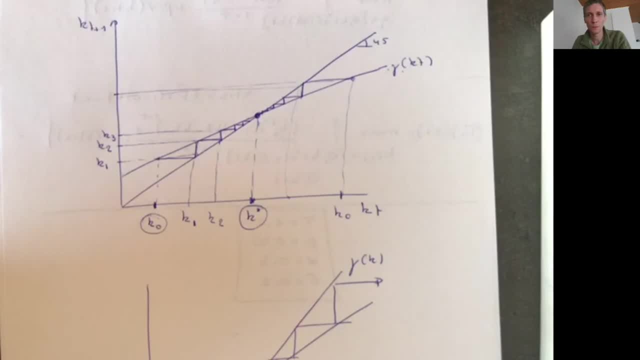 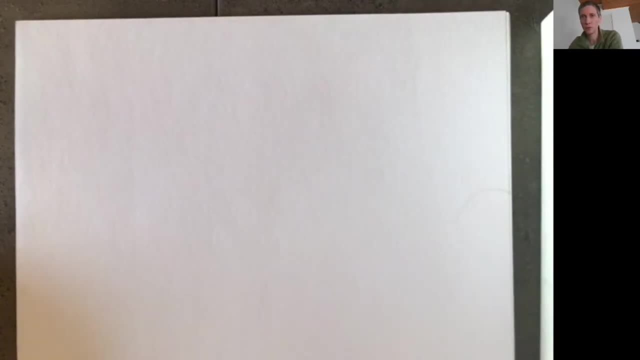 of your model here, so just a very simple model, but okay. so one thing that's quite slow in the model is the optimization step, right. so now we basically iterated to every possible action that we could take, and then we only updated the value if we found something bigger. right, because this is? 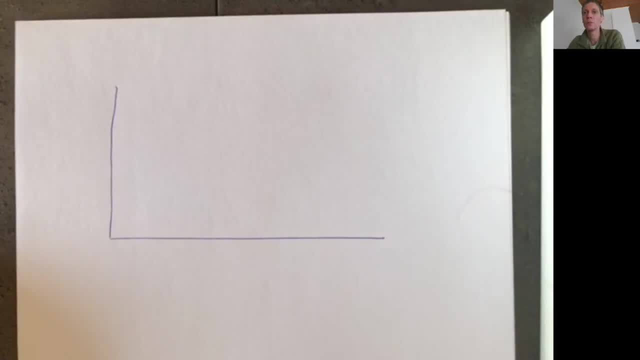 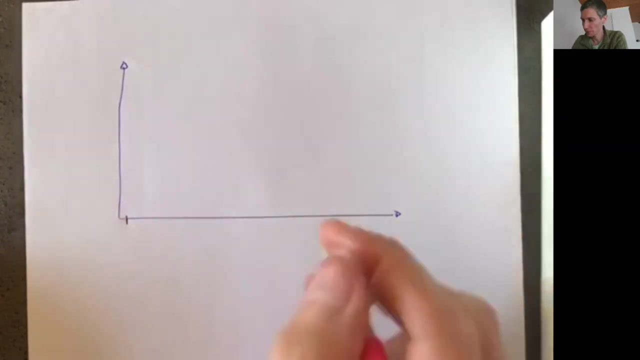 in general, this is a very bad idea because it's a very lazy way of optimizing a function. so, however, we know that the objective function is concave, right because of the theoretical analysis beforehand. so, basically, we can be a bit smarter here. so in the sense that, so if these are all my levels of capital, i have a discrete grid. 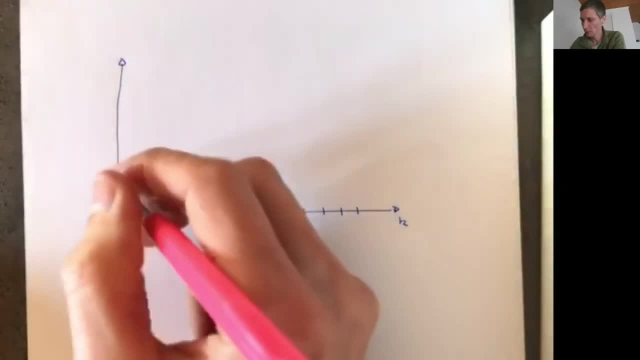 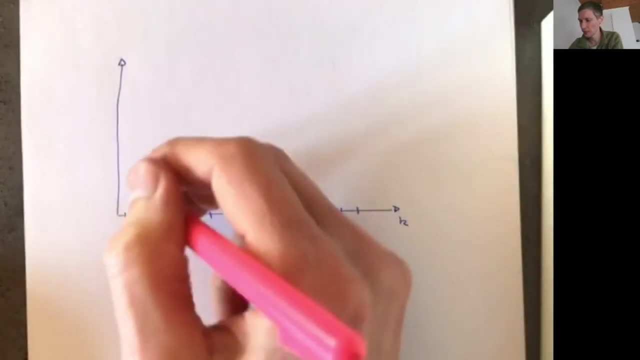 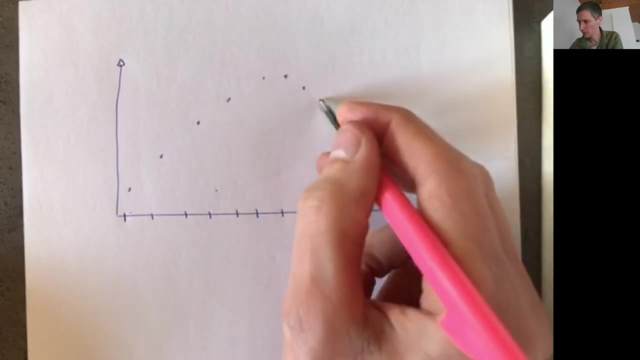 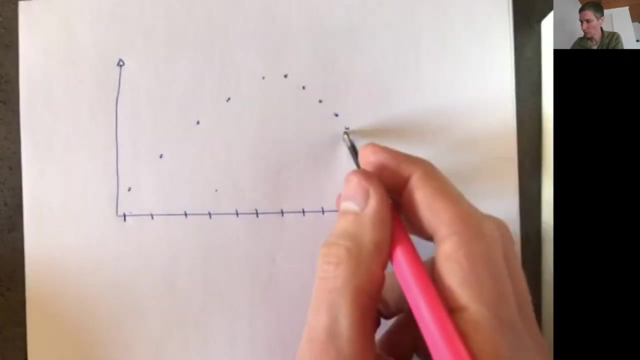 right. so this is levels of capital. basically, i want to optimize a concave function right, or a concave discrete function, in the sense that it first increases and it reaches some optimal value and then it decreases later on, right and if so, this is my choice- variable kt plus one and if at some point kt plus one is too big, 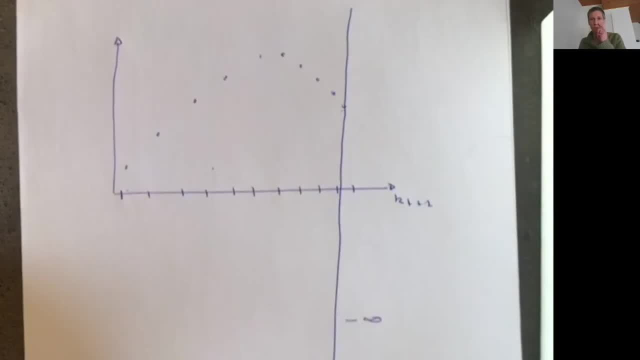 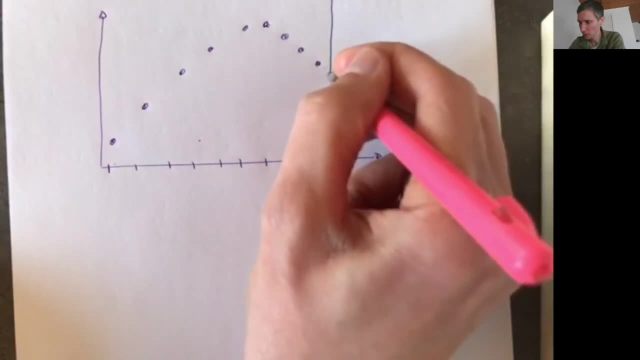 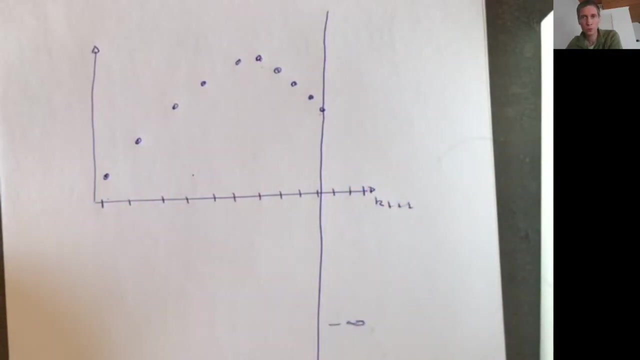 then basically, i'm going to minus infinity because it's no longer feasible. all right, so this is the kind of function that i would like to optimize right. it first increases and then it decreases, so there's a unique maximum point here. so what i could do in order to to there are probably 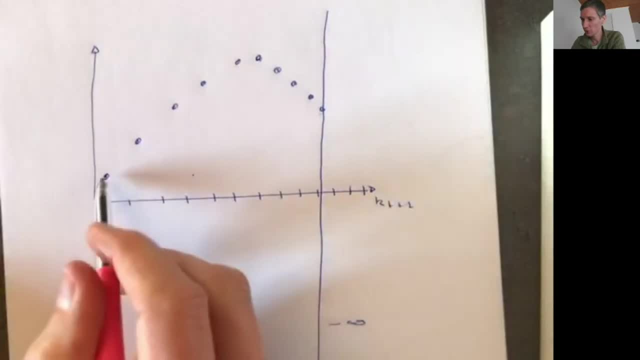 many things that you can do to find the optimum faster than just. so what we did now is we computed this value, right. then we computed this value and said: if it's bigger, okay, substituted by this one. and then we computed this one, and then we computed this one, and then this one, and then this one, and we 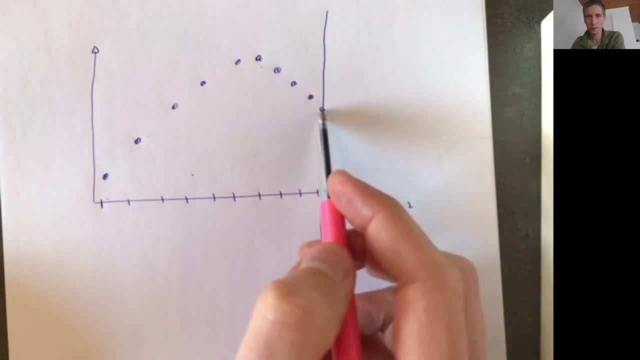 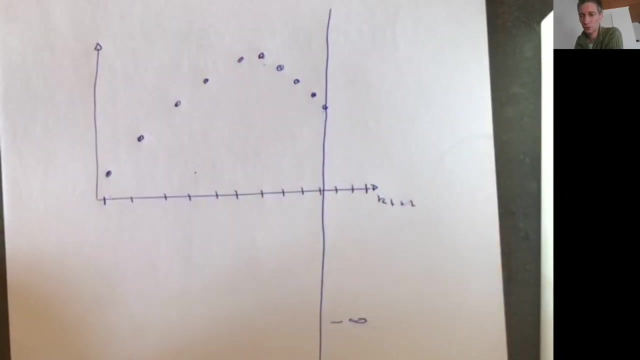 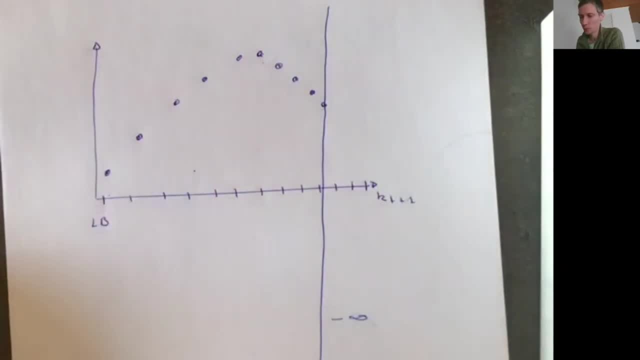 that you can do well is you can use a lower bound and an upper bound, okay. so the idea is, i know that my optimum is between my lower bound and my upper bound here, and then i can take a point here between the two. let's say this one here and i can evaluate the function at this point, okay. 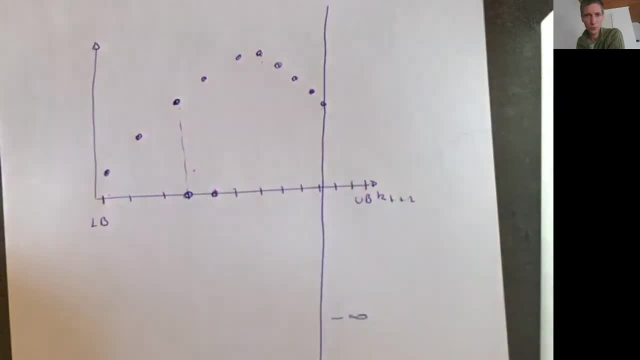 and then i can take, for example, this point, which is the next one, and evaluate it here and i can compare this value with this value and then if the second one is bigger than the first one, i know that i'm moving you on the upwards part of my my graph. so i know that if there's an optimum, it has to be. 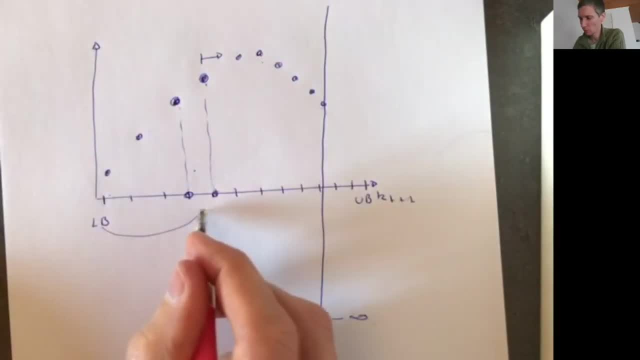 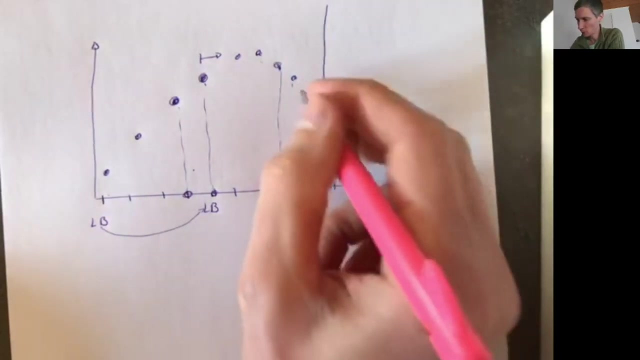 to the right of this point. so what i can do is i can update my lower bound to this value here, okay, similarly, if i, for example, am at this point right, i can take this point, i can take the next one. so here, the next one is lower than the first one. so i know that i'm 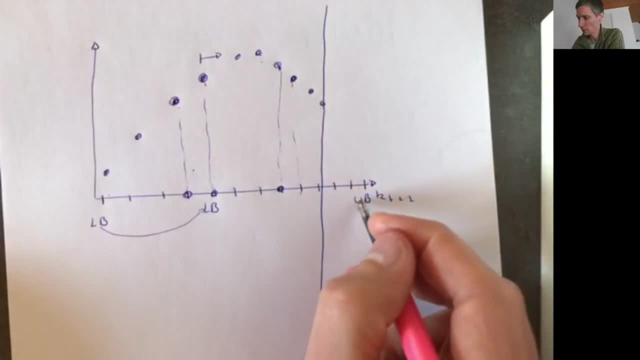 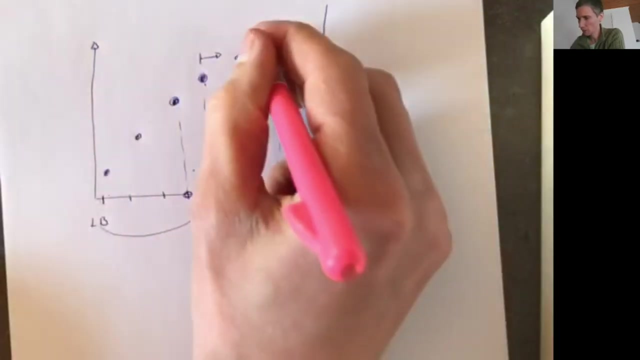 in my downward part of the graph. so i know i can move my upper bounds to this point here. all right, so basically i can take a value in between and each time i can move my lower bound and upper bound closer and closer together until they converge to the point where my graph is maximum. okay, and this will give me an algorithm. that's. 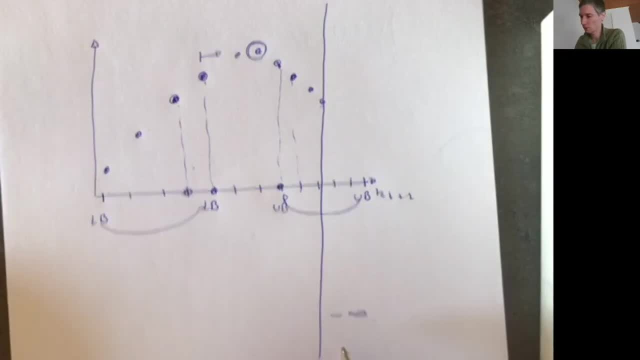 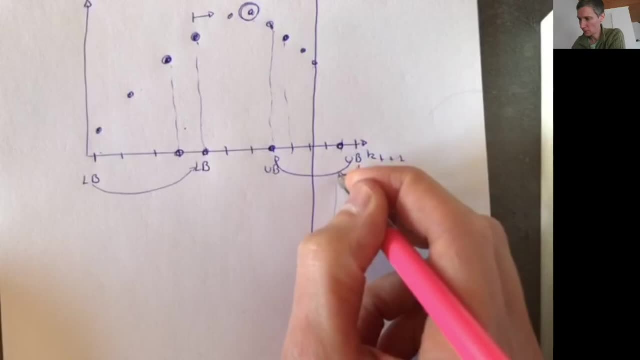 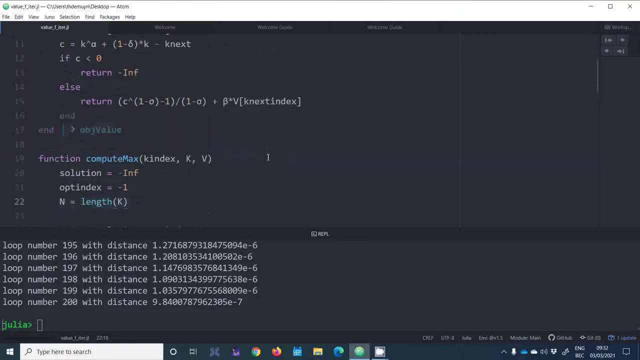 way, way more efficient than the current one that i have. also, if i, for example, sample this point and i get to minus infinity, i can easily move my upper bound here, because i know the optimum is going to be somewhere over here. okay, okay, so let's go back to our coding. so 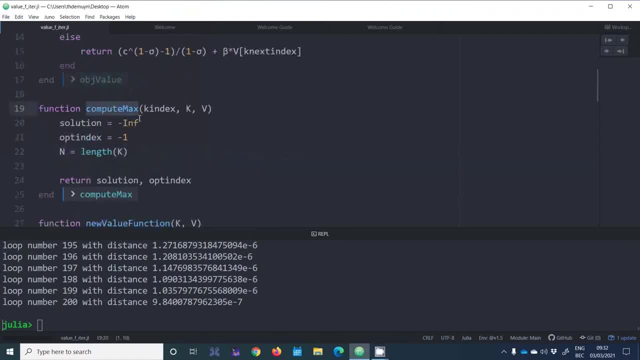 what you want to do is you want to optimize this function here, compute max. i'm already cleared out all the code that you don't need anymore. so here i'm going to have an upper bound it's going to be equal to n, and then my lower bound is going to be equal to one. 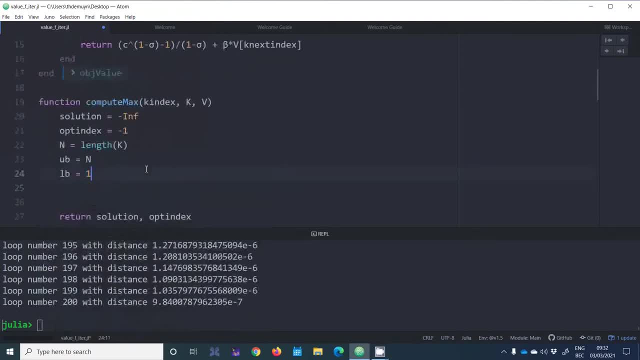 uh, so for python, counting starts at zero, right so, but this is julia, so start counting at one. for python, you have to change this to zero, okay, so we're going to have a while loop, so, while the upper bound is different from the lower bound, so i'm going to take the midpoint of d2 and i'm going 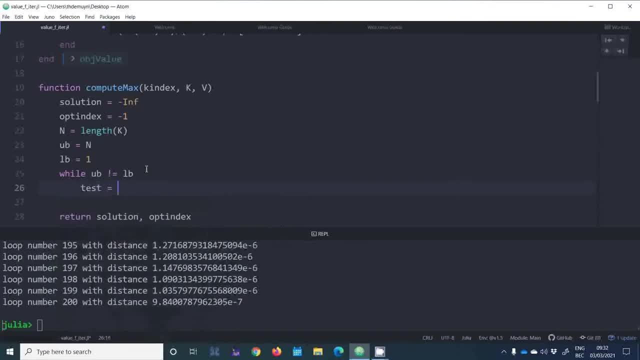 to put it at the value test. so this is going to be upper bound plus lower bound divided by two. but i want an index, right. so i'm going to take the flow which is the biggest number or integer below the mean here, and then i'm going to have to convert it to an integer because i want to use 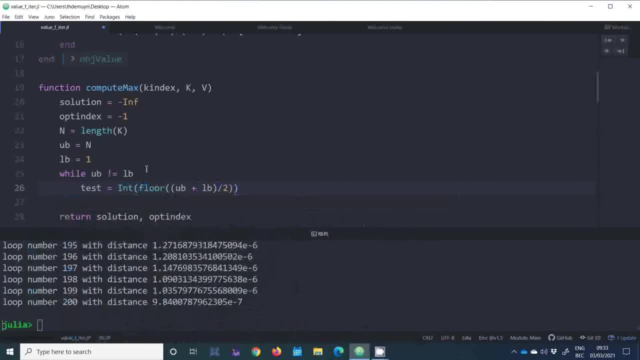 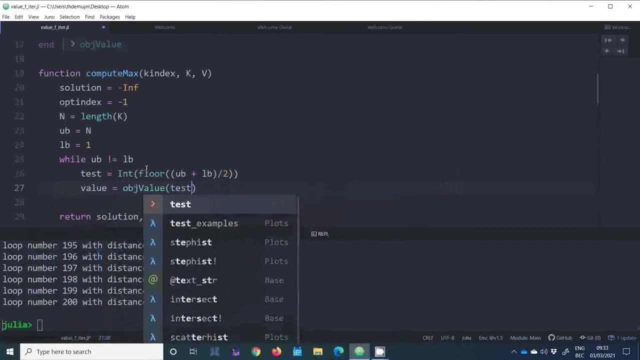 it as an index. okay, so i get this function here. then i want to compute the value of my objective function at this index here. so let me call: this value: is objective value at test? no, at k index of test. then i'm going to put k and v and i want to compute the value at the next. 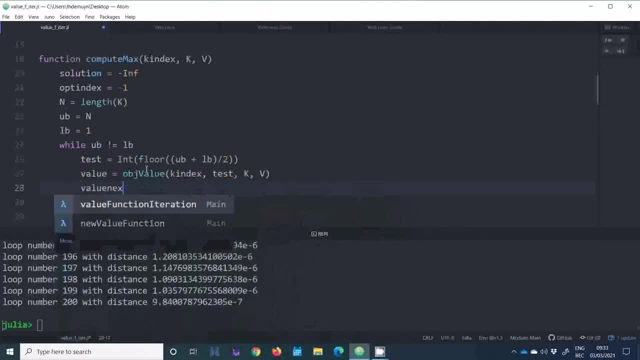 index, so let me call this value. next is objective value of k index test plus one, kv. okay, and because here i've took on the floor, i always i know that test plus one always exists, okay, so that's another problem here. so if value- i've taken the floor i always- i know that test plus one always exists, okay, so that's another problem here. 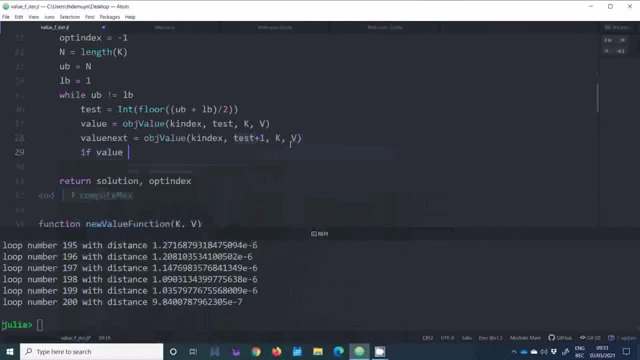 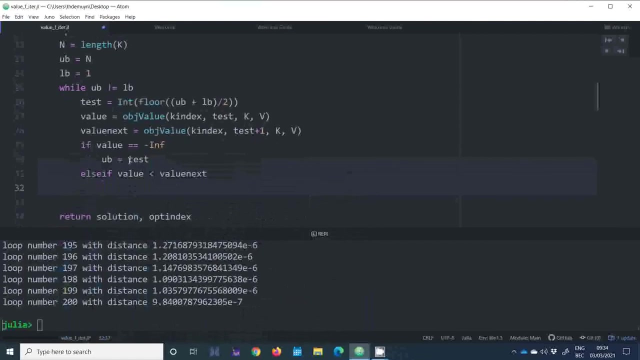 so if value is equal to minus infinity, right. this means that my objective function evaluates the minus infinity. so the problem is not feasible. i can put my upper bound equal to the value of test. okay, also, if it would happen that value is smaller than value next, well then i know that my optimum 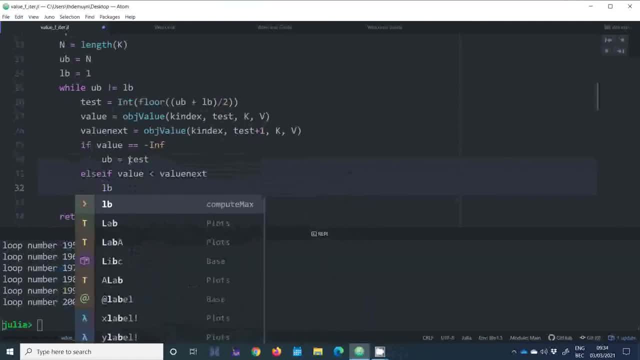 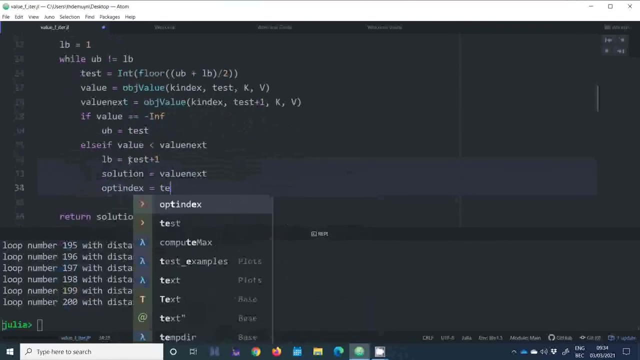 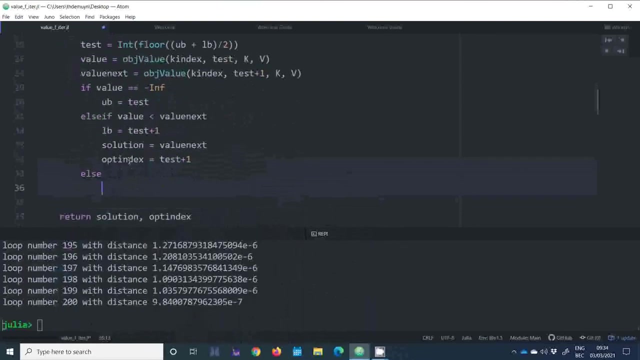 is to the right of value next, so i can put my lower bound equal to test plus one. i can update my opt, my solution, sorry- to value next and my opt index to test plus one, okay, and then else i know that value is bigger than value next. so my maximum value is to the left.